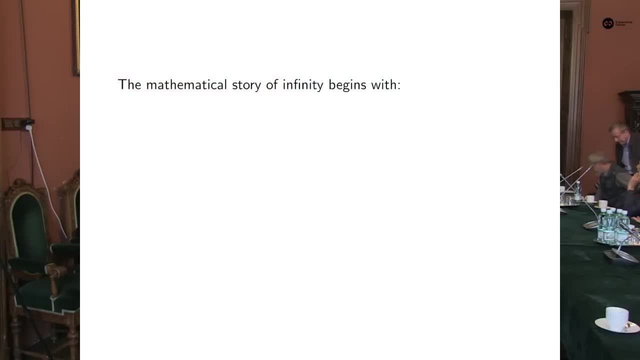 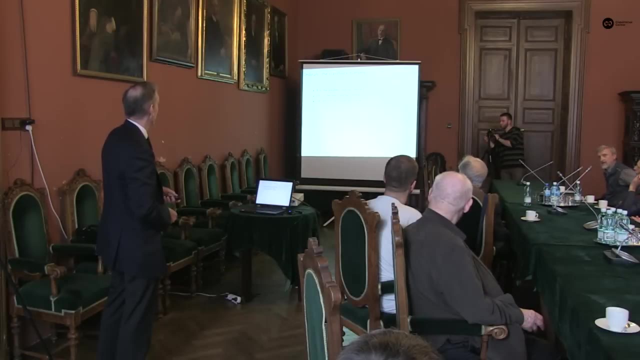 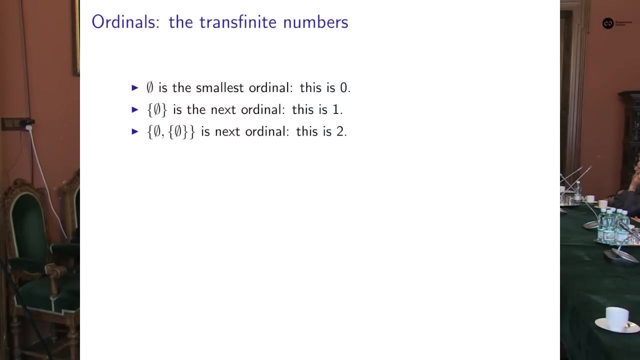 Okay. so if you're going to talk about infinity or set theory, you start with nothing- The empty set- And then you introduce the transfinite numbers. Again, you start with a finite. The empty set is zero, The set whose only member is the empty set is one, and so forth. If alpha 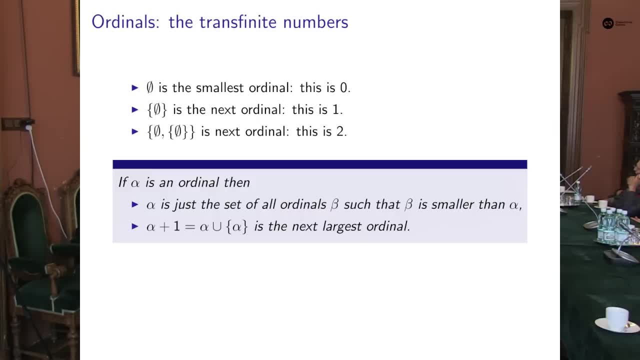 I'm defining the ordinals. Every ordinal is the set of all of the smaller ordinals And you get the next ordinal by just adding to the ordinal the set whose only member is that ordinal. And then omega denotes the first infinite ordinal. It's the set of all finite. 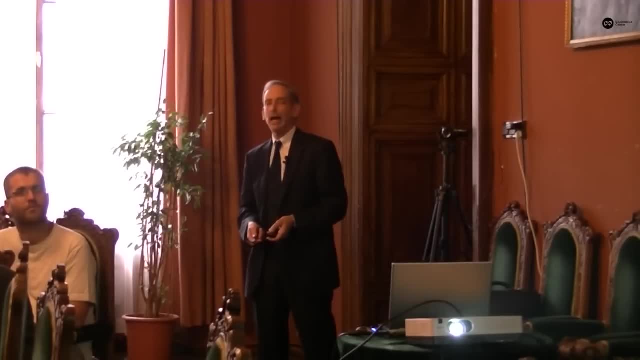 ordinals. Okay, so the ordinals provide the backbone, if you want, for the universe of sets. So I want to describe that, but I have to define an operation. So if you have a set, the power set of the set p of x is the set of all of the smaller ordinals, The set of all the 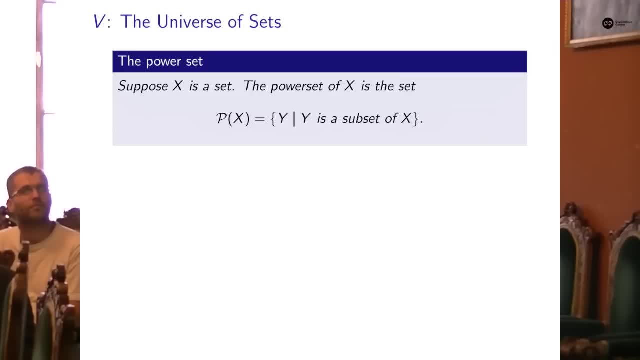 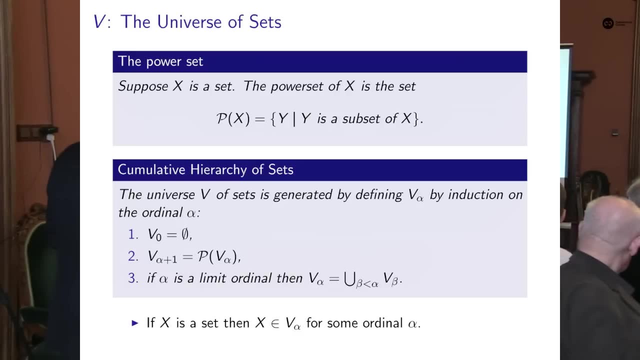 x is just the collection of all subsets of that set, And so we can now iterate this operation, And that gives us the cumulative hierarchy. So we start with nothing. At a successor step we take the power set, And at a limit stage we take the union of everything we've defined. 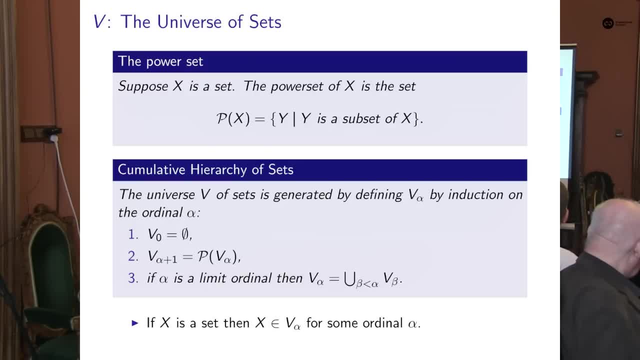 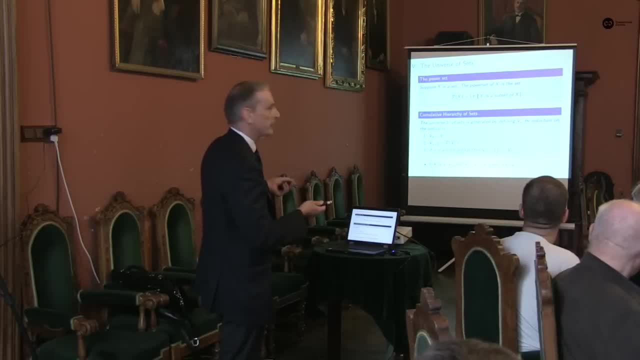 previously And then, as a consequence of the axioms of set theory, every set belongs to a v alpha for some alpha. So if you want to understand the union of all the sets, you could understand v0. That seems pretty simple- Then v1, then v2, and so forth. So let's look. 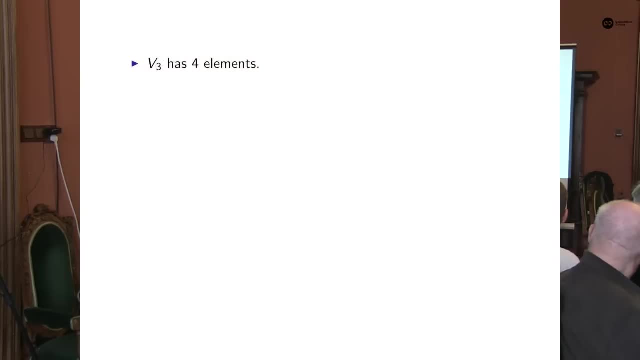 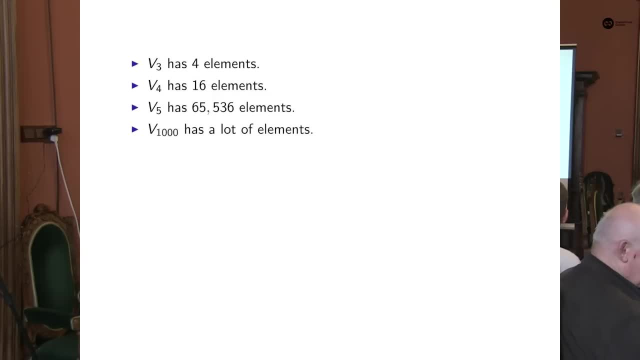 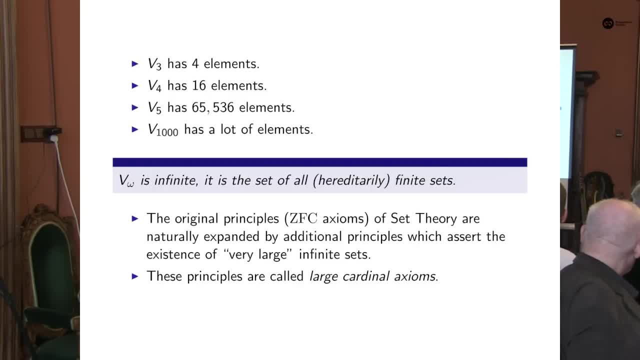 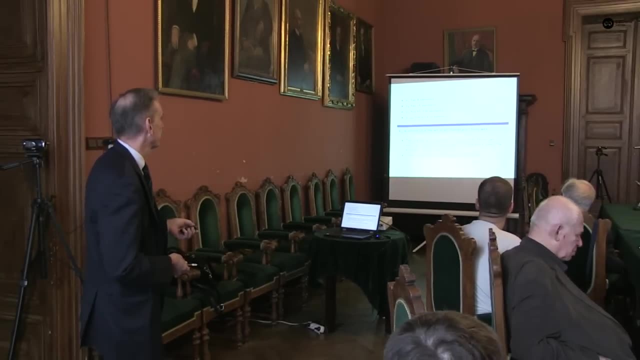 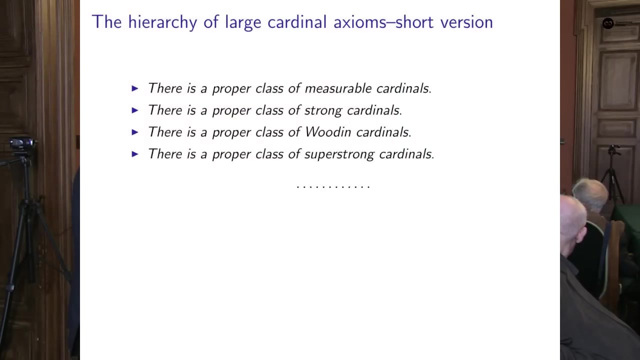 the universe of sets and they can be expanded by new principles. You assert the existence of very large sets and these are called large cardinal axioms. So it's the basic source of new principles and we'll see that we need new principles. So here's kind of a very short list of large cardinal axioms. 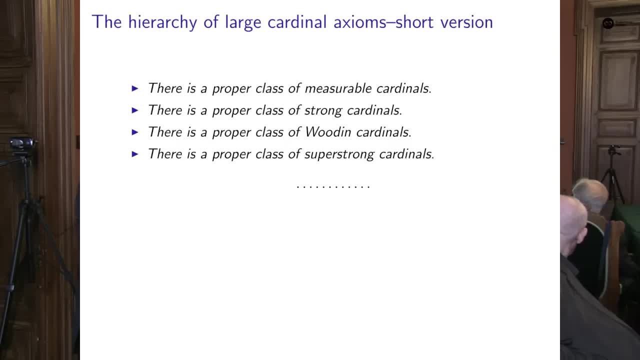 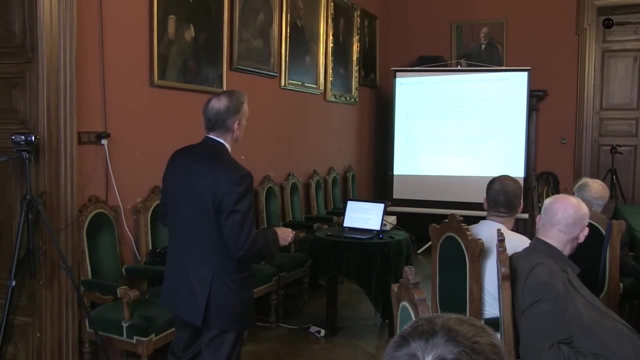 measurable cardinals, I put at the bottom, then strong cardinals- I have to mention wooden cardinals- then super strong, then super compact, extendable, huge, omega, huge. It's a big hierarchy. The reason for this dotted line is that we understand. 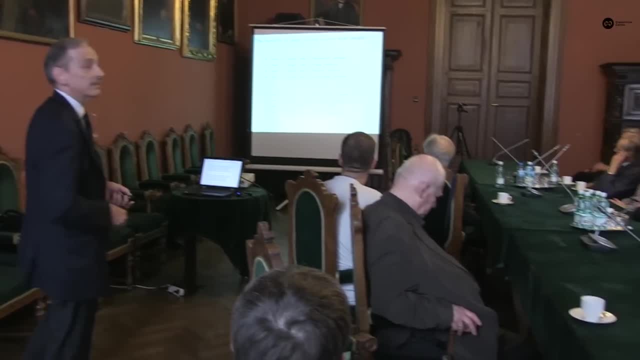 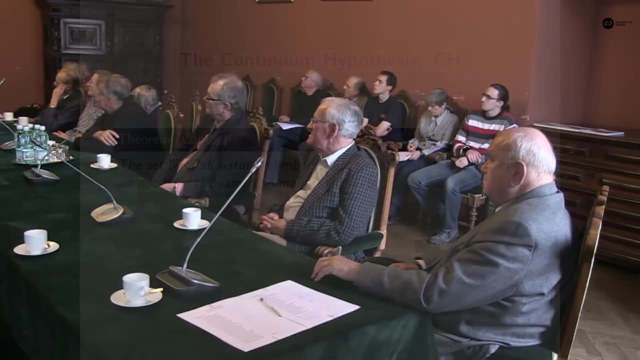 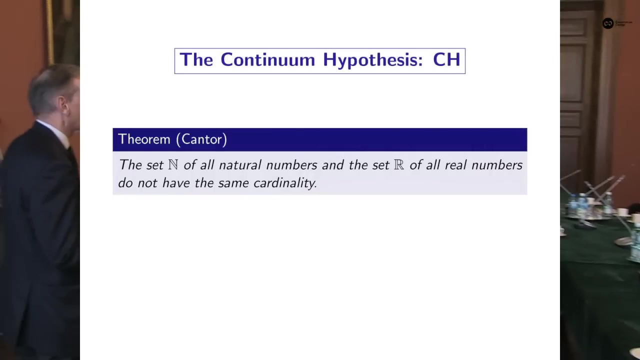 these principles more than we understand these, And that distinction is going to play a central role in what I'm going to say today. All right, the continuum hypothesis. It begins with the theorem of Cantor that if we let n be the set of all natural numbers, those are the numbers 1,, 2,, 3, and 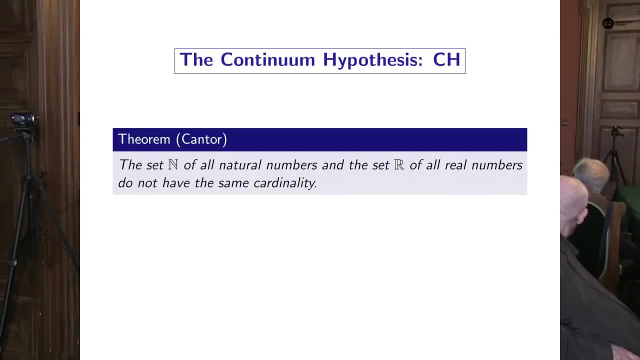 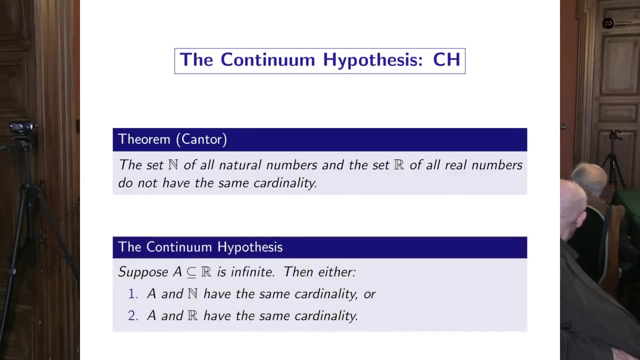 so forth. r as a set of all real numbers. these two infinite sets do not have the same size. There's no matching possible between these two sets. infinitely Infinite sets come in different sizes, And so once you have Cantor's theorem, you 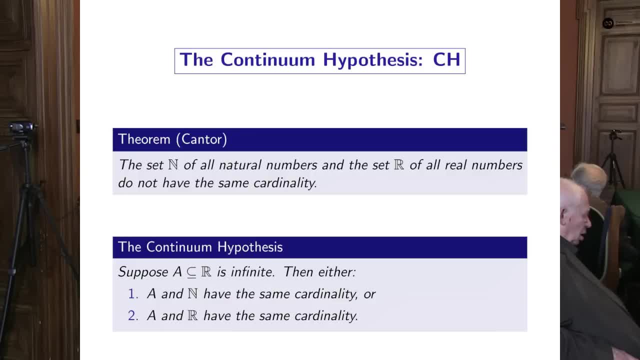 have a question: Is the infinity of the real numbers the next infinity after the infinity of the natural numbers? Another way of stating that is stated as the continuum hypothesis says that if you have an infinite set of real numbers, you can either match it with the natural numbers or you can match it with all of 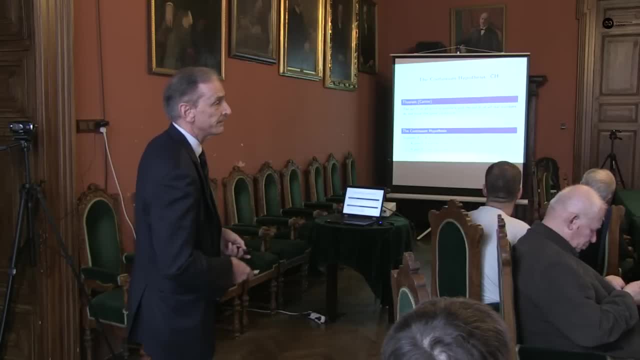 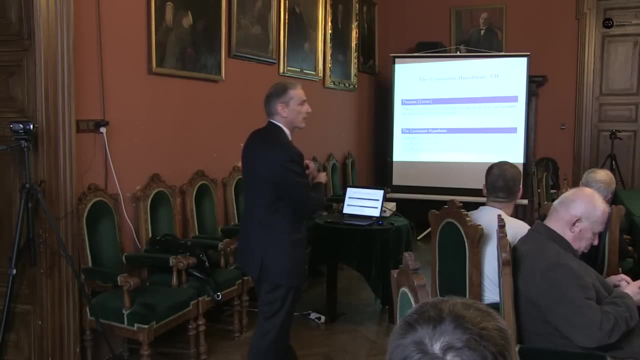 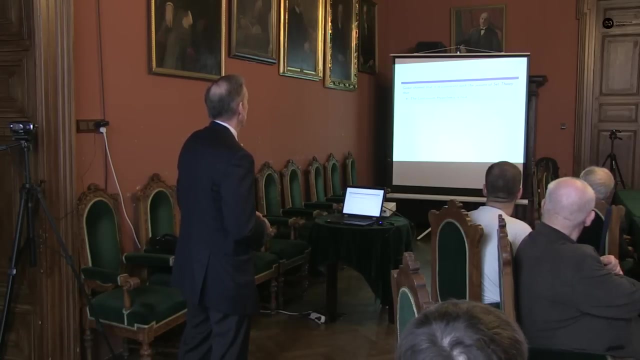 the real numbers. There would be no infinity in between. So if you're going to study infinite sets and study infinite arithmetic, this is the first question you would ask And that was the first question Cantor proposed. So I mean, as you all know, in 1900, Hilbert put: 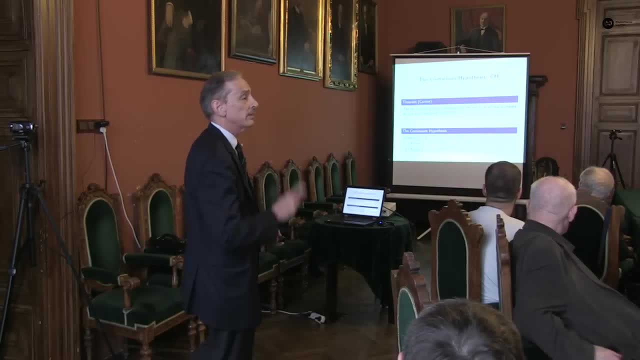 the problem of the continuum hypothesis as the first question on his list of his famous list of questions And his first question that he had was: if you have an infinite set of real numbers, will you be able to match them? So, If I have an infinite set of real numbers, 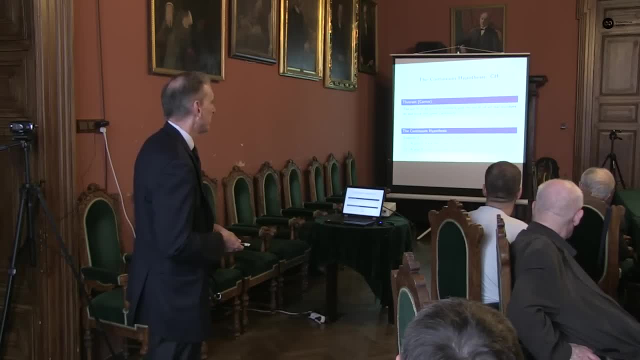 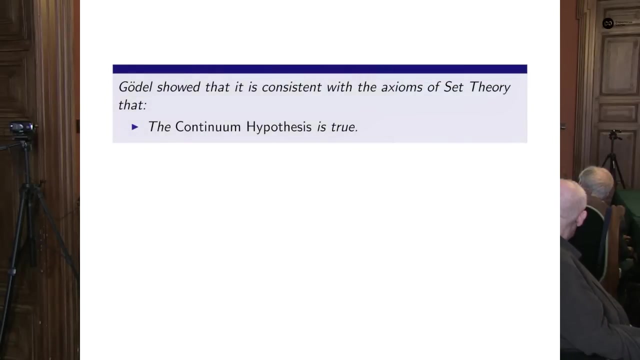 I'd say by the middle of the 20th century it was widely regarded as one of the major problems of mathematics. A lot of people tried to solve it. In 1940 Gödel showed that it's consistent with his axioms of set theory that the 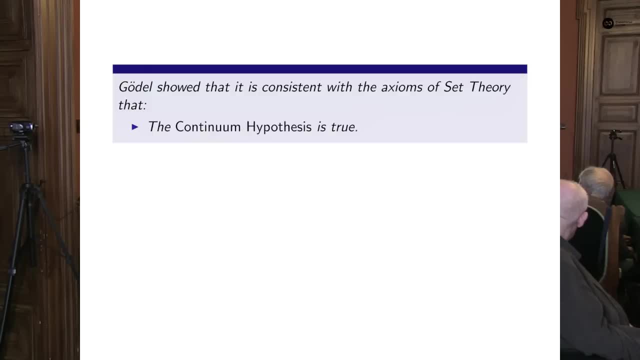 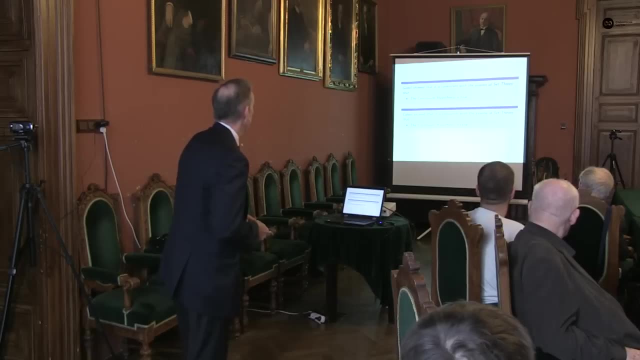 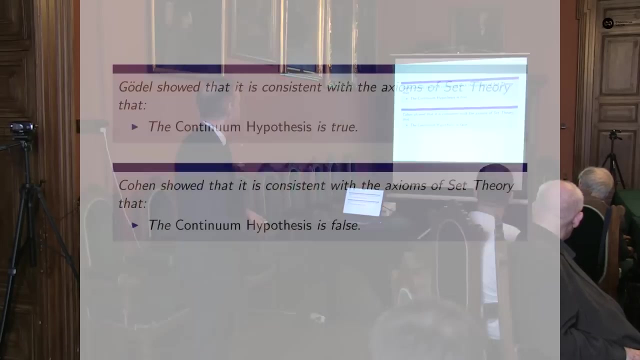 continuum hypothesis is true. In other words, you're not going to be able to refute the continuum hypothesis unless the axioms are inconsistent. And then the real change happened about 20 years later. It was in fact 50 years ago, last summer, that Cohen announced his result in a colloquium at Berkeley. So 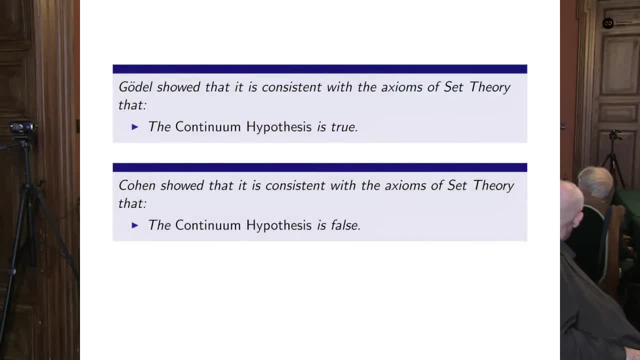 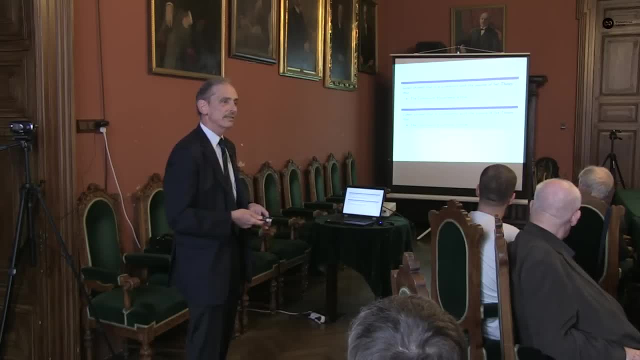 Cohen showed that if the axioms of set theory are consistent, then they're consistent with a statement that the continuum hypothesis is false. So, based on the ZFC axioms, there is no answer. It can be either true or false And the continuum hypothesis is just a statement about V, omega plus 2.. It's at: 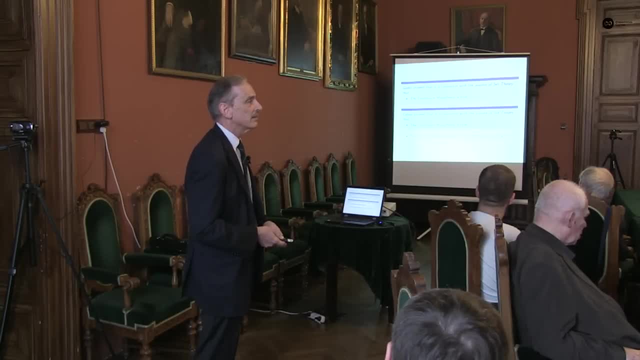 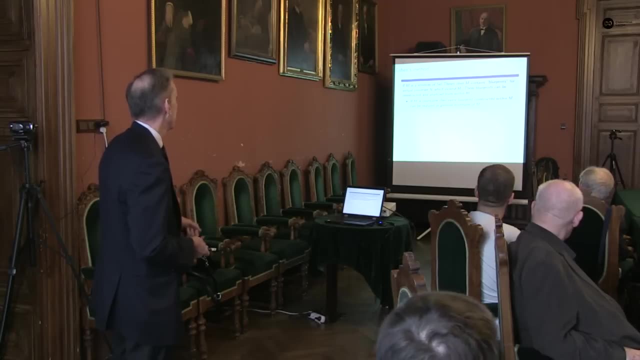 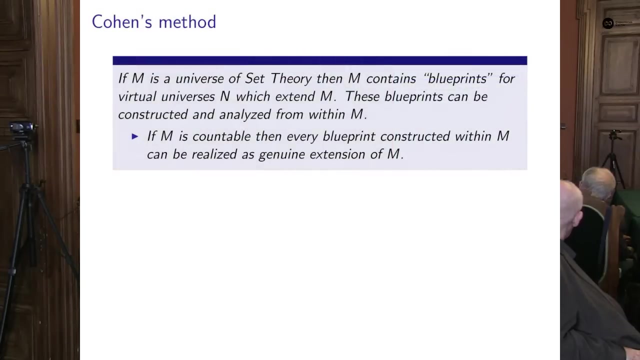 the bottom of this hierarchy of sets. So already we've run into trouble. So I want to say a little bit about Cohen's method. I'm going to do it in very informal terms. If you have a universe, a structure in which the ZFC axioms hold, we'll call. 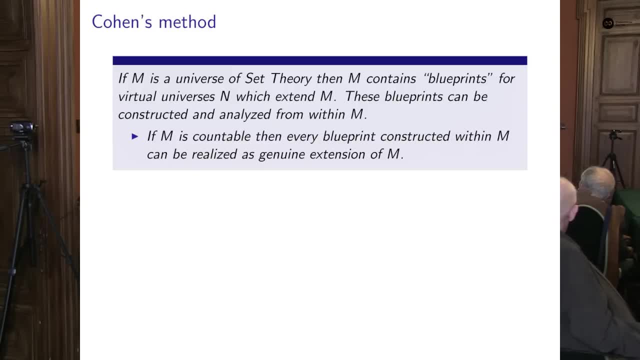 that a universe of set theory. then within the universe M you have blueprints for virtual universes which extend M And these blueprints can be constructed and analyzed within the initial universe. If M is countable as a structure, then you can actually realize these blueprints as genuine. 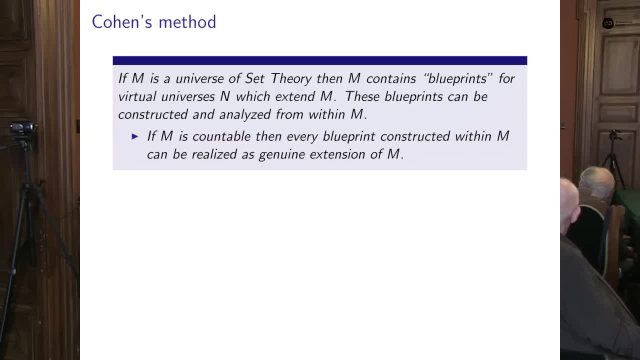 extensions. So that's what Cohen's innovation was. Cohen proved that every universe contains a blueprint for an extension in which the continuum hypothesis is false. That's how he showed that the ZFC could not refute the continuum hypothesis, could not prove the continuum hypothesis. Cohen's method actually also. 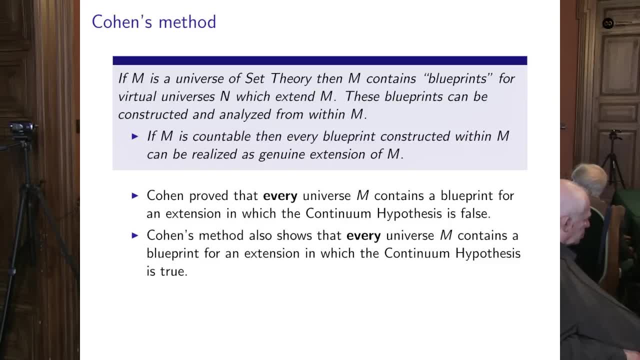 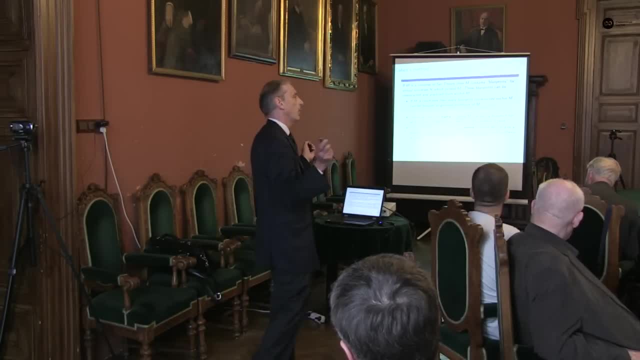 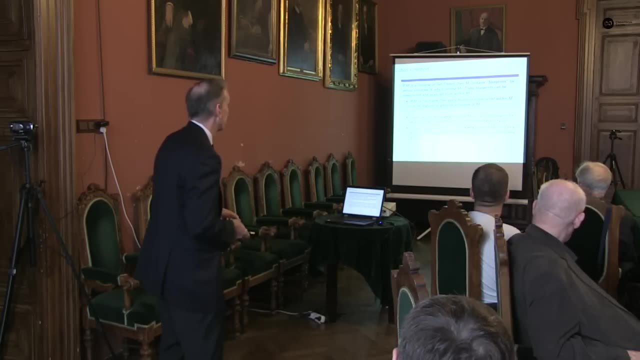 shows that every universe contains a blueprint for an extension in which the continuum hypothesis is true. And that's not how Gödel, of course, did it, because the whole idea that you could build extensions was the major unsolved problem. So that's the mathematical problem that Cohen 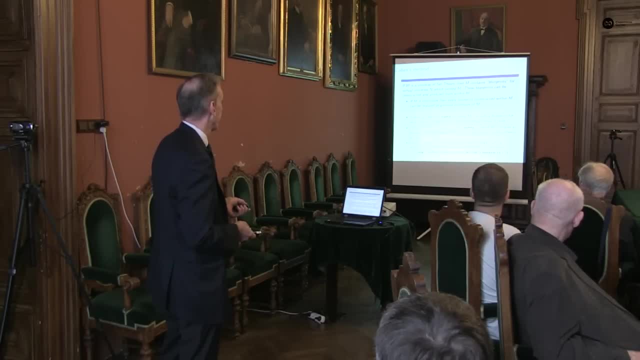 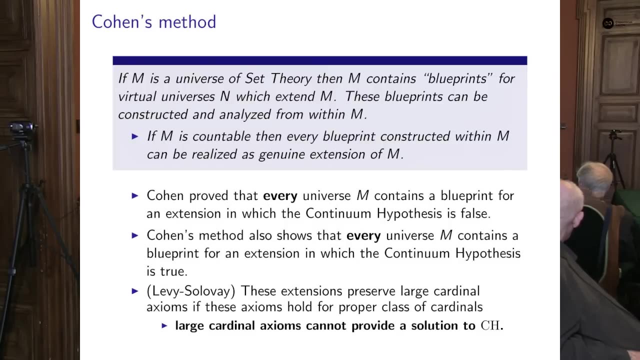 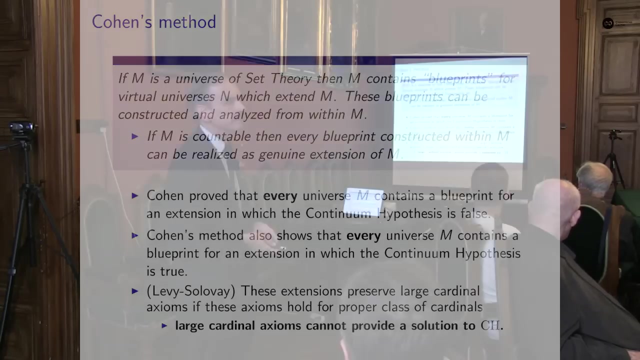 solved, and a very powerful method. Levy and Solovey showed that these extensions preserve large cardinal axioms. The axioms hold for a proper class. Therefore large cardinal axioms can't be used to build extensions. The axioms cannot provide the solution, Because if you had these large cardinal axioms, 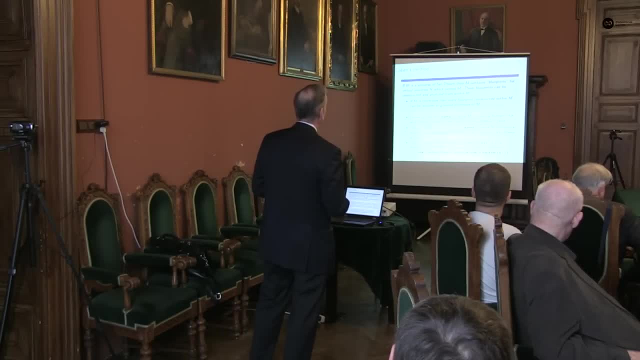 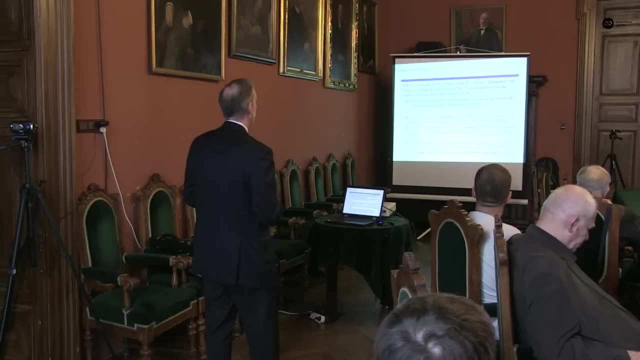 within M. holding the blueprint that Cohen defined here would preserve those axioms and make the continuum hypothesis false. This blueprint would preserve those axioms but make the axioms true. So the major source of new intuitions about sets cannot answer CH. 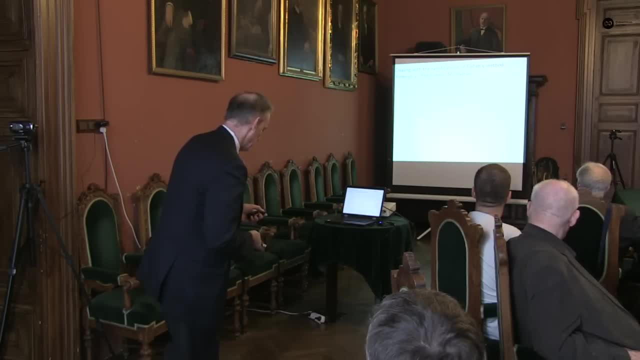 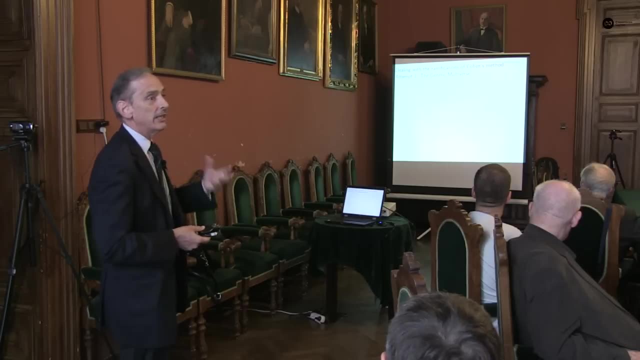 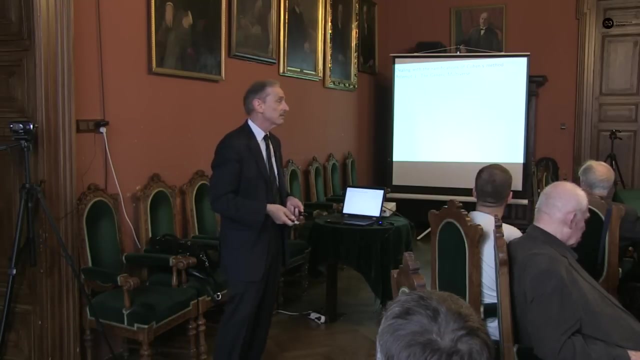 So this is even more troubling. So we need to either come up with an answer for the continuum hypothesis or change our conception of truth. So the first thing you might do is alter one's conception of truth, A little bit like what happens in physics. In physics you have these dimensionless constants like the ratio of 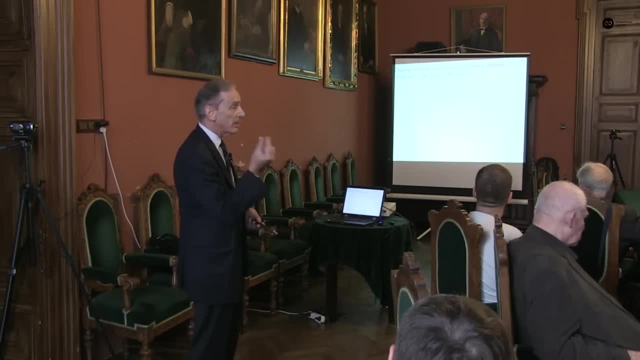 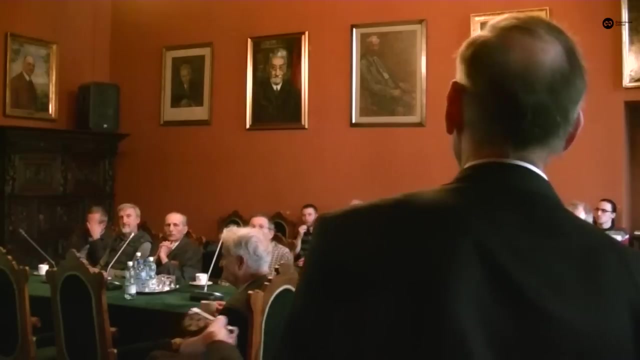 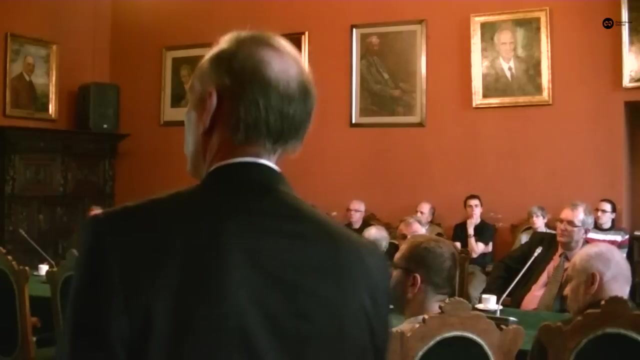 the mass of the electron to the mass of the proton. These are numbers, constants which don't depend upon the units. So the dream of physics is to compute these constants from first principles. And now some community of physicists think this may not be possible and that these are intrinsic ambiguities. All you can do is have: 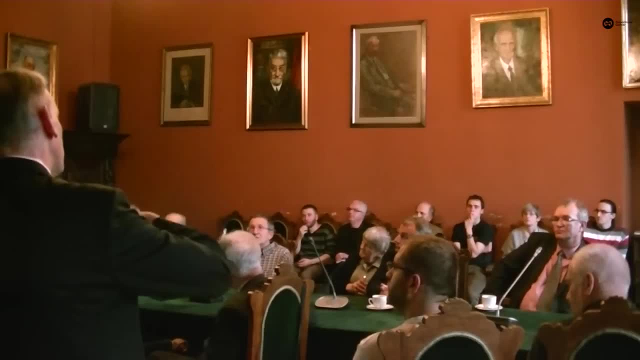 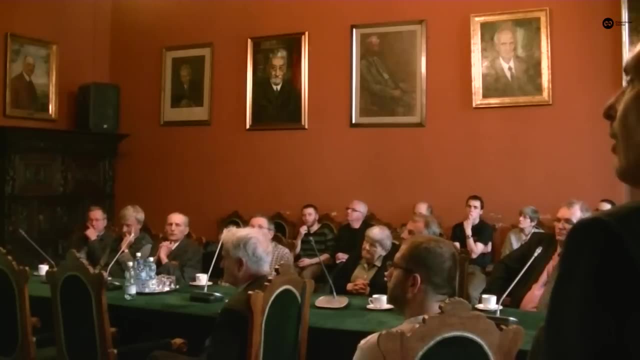 a multiverse conception, and these fundamental constants may vary from universe to universe. it's the same thing. So we could conceive of I'll call it the generic multiverse. Cohen defined his extensions, the realization of blueprints, as generic extensions. 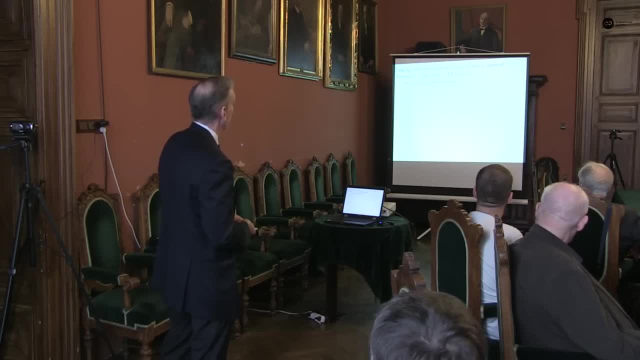 All right. so how one might do this, I'm going to describe for you the generic multiverse with capital letters. This is the multiverse that we would view as generated by the universe V. Well, therefore, V should be in the generic multiverse. 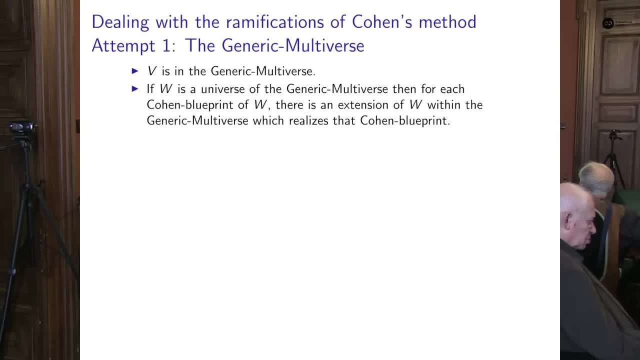 And now the idea is: if a universe is in the generic multiverse and you have a Cohen blueprint within that universe, than there should be an extension in the generic multiverse that realizes that blueprint. If you have a universe in the generic multiverse, that 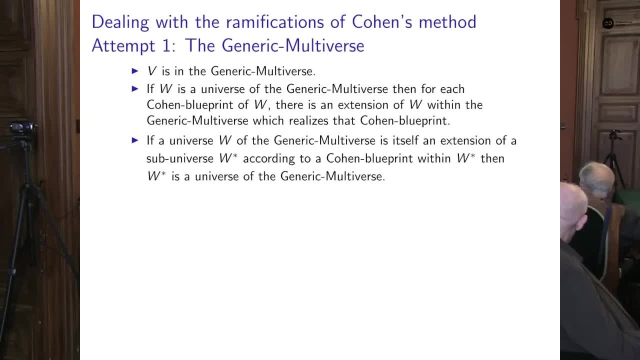 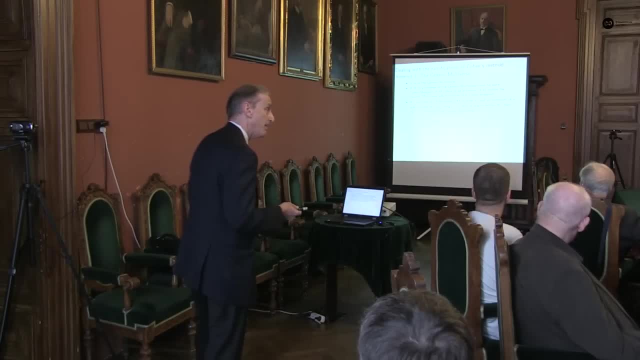 itself is an extension of a sub universe by a Cohen blueprint within that sub universe than that sub universe would be your universe. V Right is also in the generic multiverse. Now it could happen that you start in a universe, realize a Cohen blueprint and see another way that you could get to the new universe. 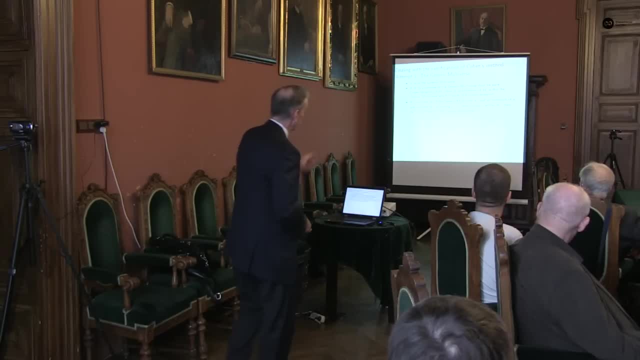 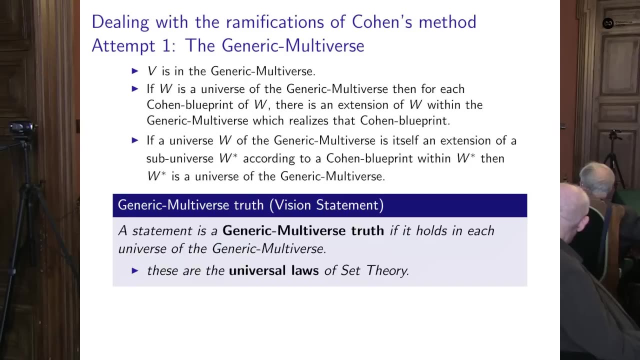 by a Cohen blueprint, a different starting point, And so this is transitizing that relation, And then this would be the conception of truth. We'll say that a statement is a generic multiverse truth if it holds in each universe of the generic multiverse. These would be the universal. 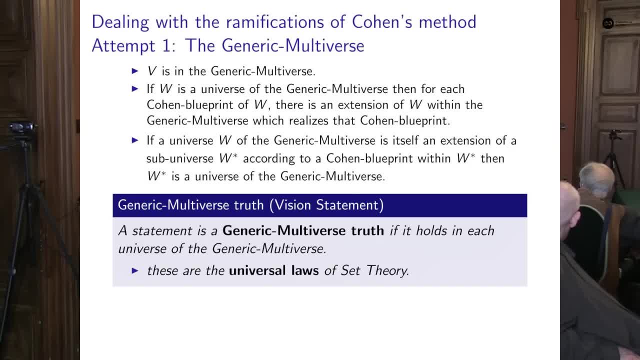 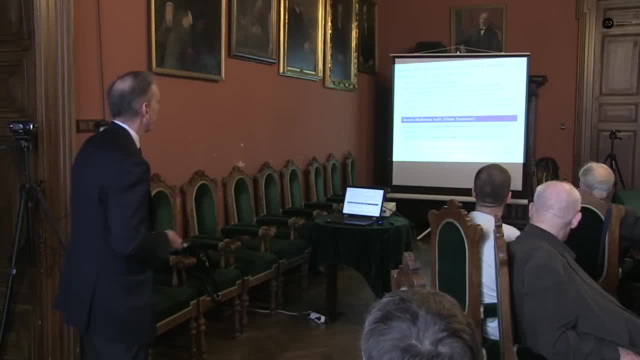 laws. So this is just taking the multiverse conception and saying this is our notion of truth. Now there's a critical mathematical theorem. you need to make sense of this because there's some ambiguity, potential ambiguity, in this conception, Because I just said there: 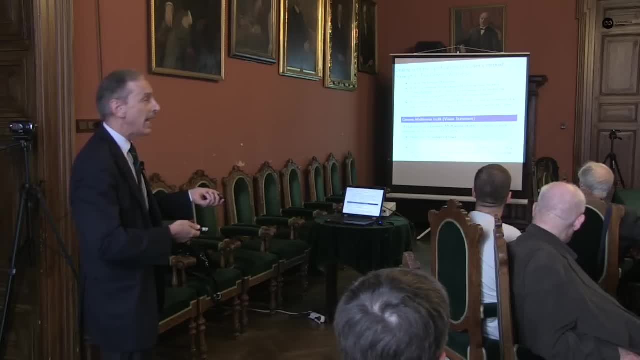 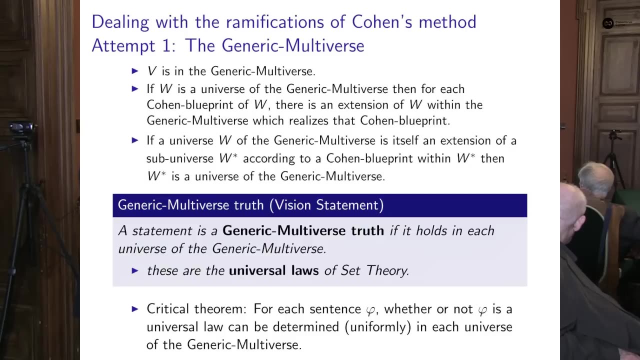 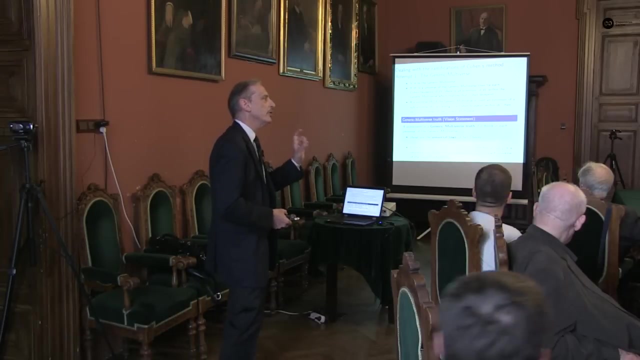 was one extension. Maybe it should be all extensions, or maybe it matters. And the answer is it doesn't, For each sentence phi, whether or not phi is a universal law, can be determined uniformly in each universe of the generic multiverse. So this does two things: It says, it doesn't. 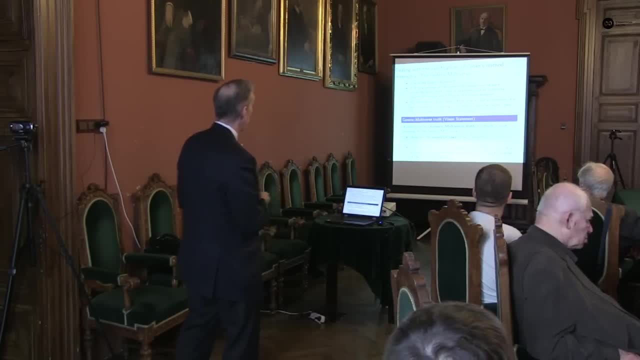 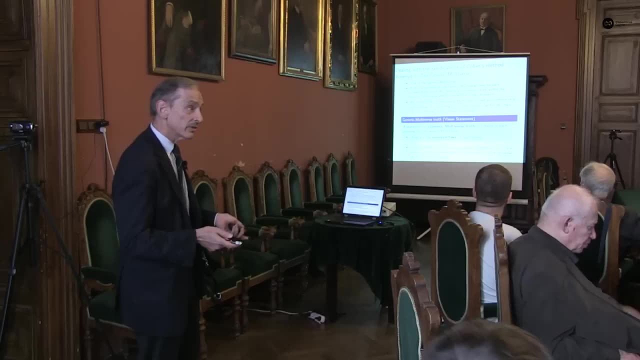 matter how you conceive of the generic multiverse, as long as it satisfies these two principles, you get the same universal laws. It also says it doesn't matter what meta-universe you're forming the generic multiverse in, because every universe of the generic multiverse will compute the same universal laws. 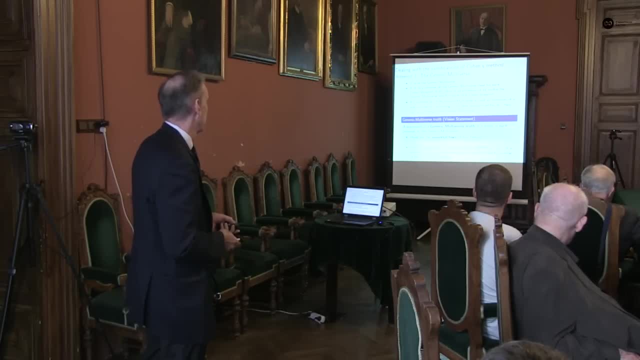 Okay, so you need that mathematical theorem to make sense, to show that this is a philosophically coherent view. Now, since the laws can't change when you pass to a Cohen blueprint, Cohen's method cannot be used to show that statements are independent or unsolvable in this notion. 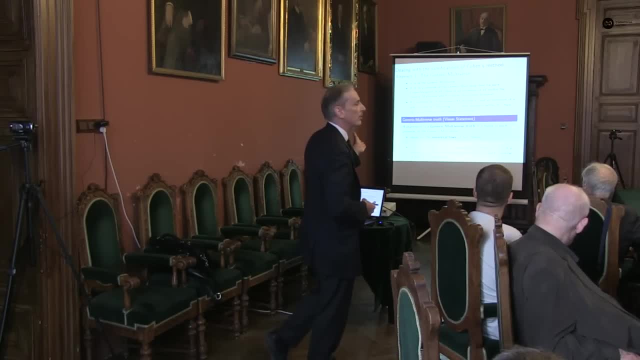 of truth. Now there's statements that are neither true nor false, Like the continuum hypothesis is not a universal law, Because you can make it true, you can make it false. All right, so we now have three categories of statements: The statements that are always. 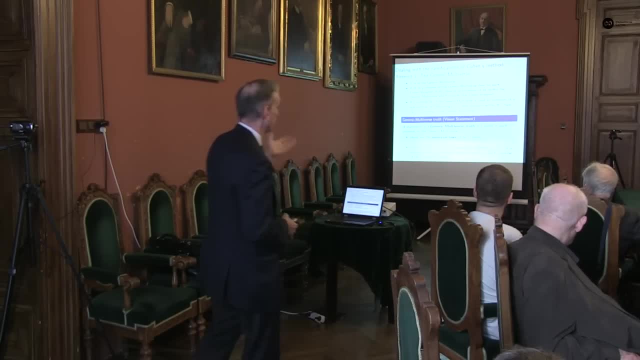 true. those are the laws, The statements that are always, that's the laws of like your hypothesis, So you can claim this statement is true. that's the laws of like your hypothesis is like yours make it false, always false. Those are the negations of laws, And then the statements in between, So that's. 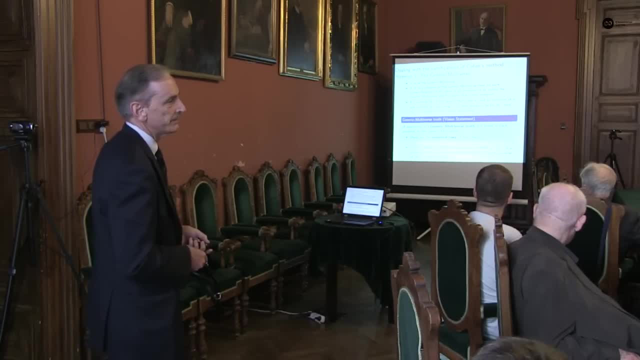 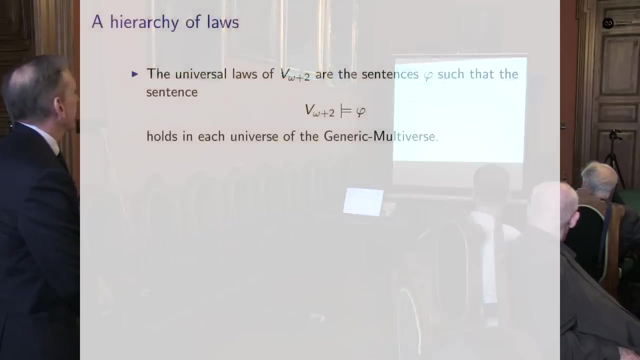 what you give up. Very appealing view, But now we want to analyze this view. I'm worried I'm going to lose track of the time. I see no clock, But I have my phone. Okay, So end of thought. All right, So we actually have a hierarchy of laws, So the universal laws? 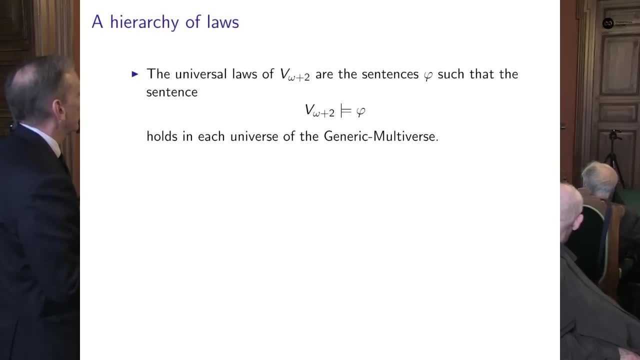 of V? omega plus 2,, that's the power of the reals, are the sentences whose truth in that stage of the universe is itself true in each universe of the generic multiverse. So these are the local laws, And then you could define the laws of V? omega plus 3, V? omega plus a. 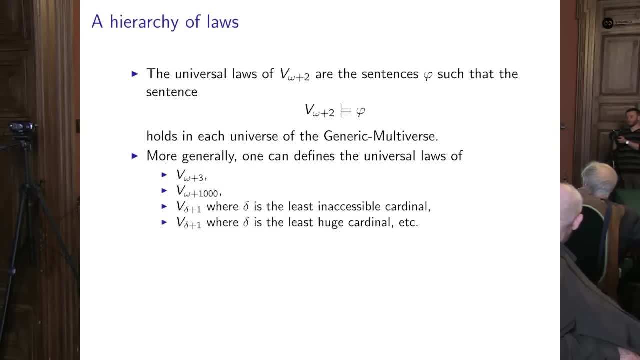 half A thousand V, omega, V, sub delta plus 1, where delta is the least inaccessible, and so forth. There's a hierarchy of local laws. These sets of laws are of non-decreasing complexity. If you know the universal laws for V, omega plus 3, you can compute the universal laws. 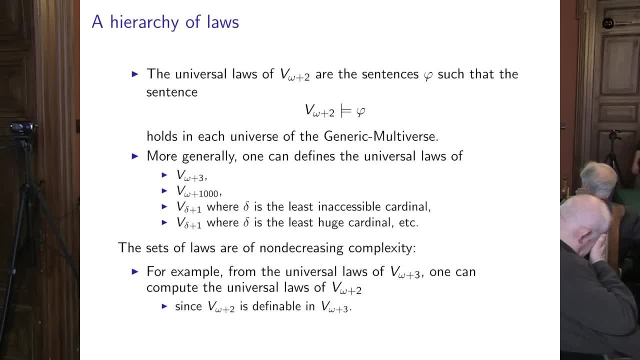 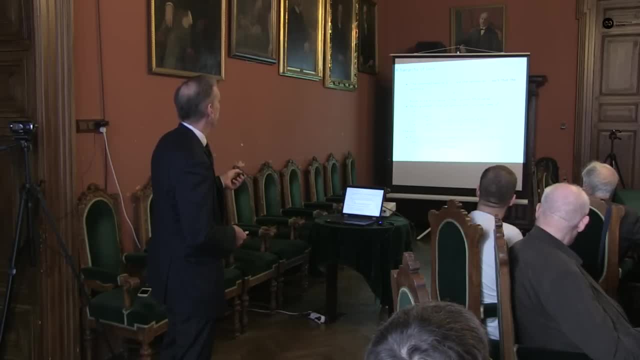 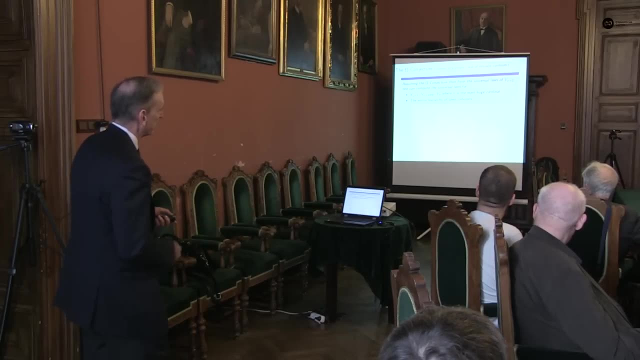 of V omega plus 2, because V omega plus 2 is definable within V omega plus 3.. So this is okay, Everything looks great, But then something happens. So I'm not going to define the omega conjecture, but when you 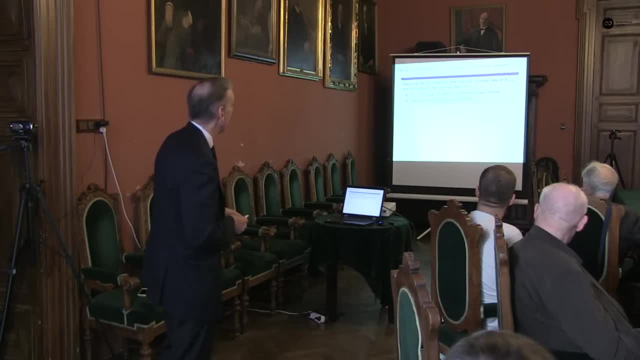 analyze this conception of truth, you're led to this mathematical conjecture called the omega conjecture. It comes out of defining the logic of the generic multiverse. There's a logic for that notion of truth. The universal laws become the omega provable sentences. 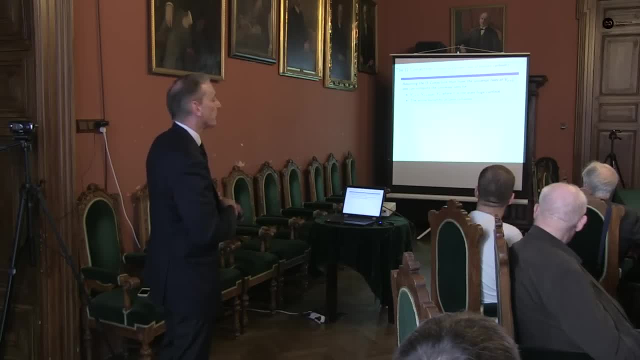 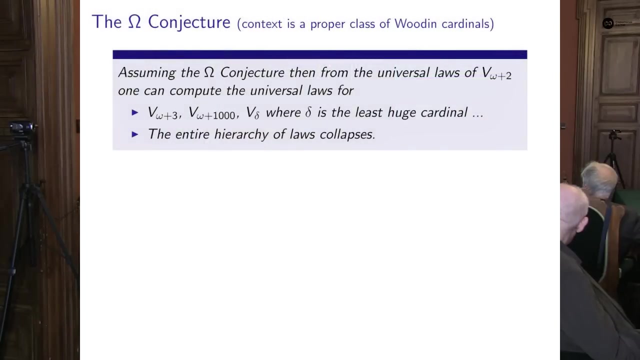 And the question: you can prove soundness? And the question is: you can find a notion of proof? And then the question is whether the analog of the girdle completeness theorem holds, and that's the omega conjecture. If the omega conjecture is true, then this entire hierarchy collapses. If you know the 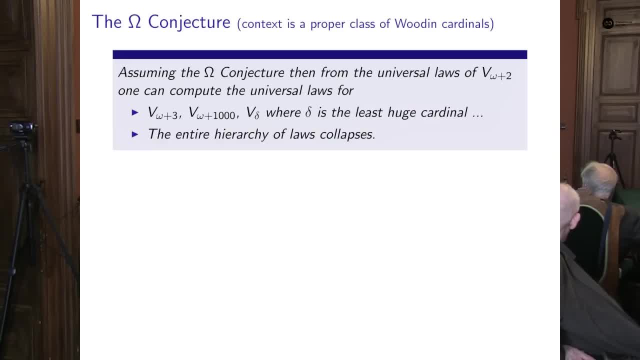 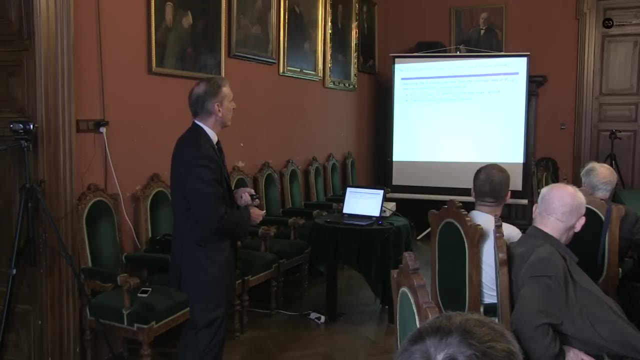 universal laws for V? omega plus 2,. you can compute the universal laws for V? omega plus 3, V? omega plus a half, V omega plus a thousand V delta. where delta is the least huge cardinal, The whole hierarchy of local laws collapses down to just the local universal laws of V? omega plus 2.. 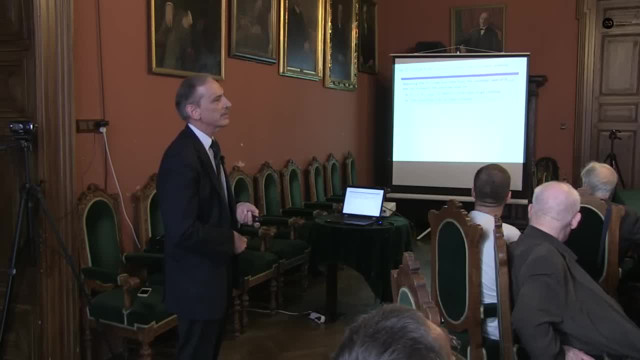 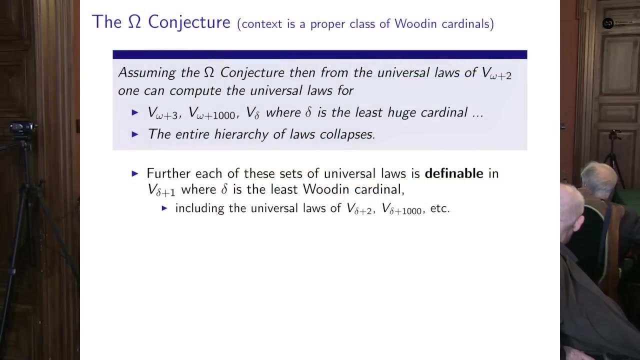 Well, in the philosophy of mathematics, there's another way of saying this: It's formalism. In formalism, you reduce all truth to truth about the integers. This is reducing all truth to truth about sets of reals. Clearly it cannot be correct, And it's even worse. So the hierarchy collapses, but each. 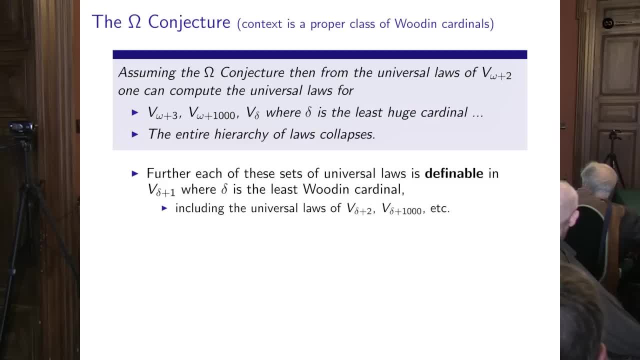 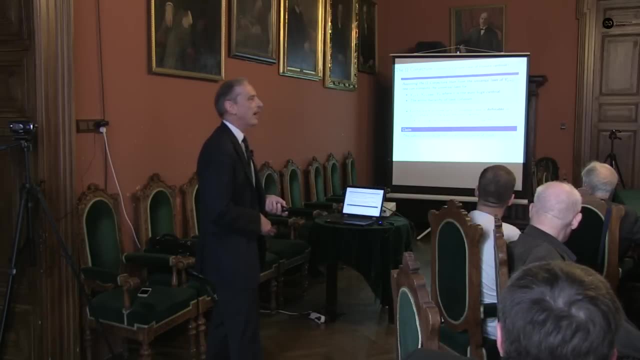 of these local sets of universal laws is definable in V delta plus 1, where delta is the least wooden cardinal. This includes the universal laws of V delta plus 2, V delta plus a thousand. This is clearly not right. It violates the whole transfinite iterative. 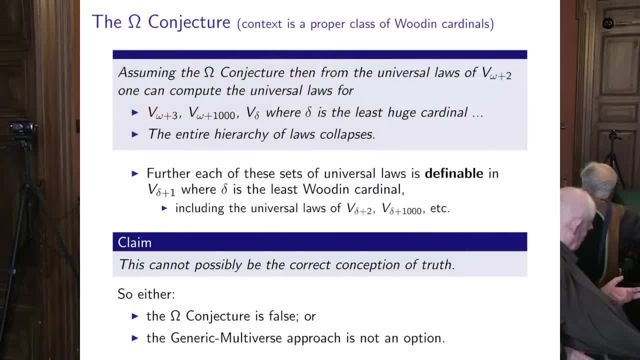 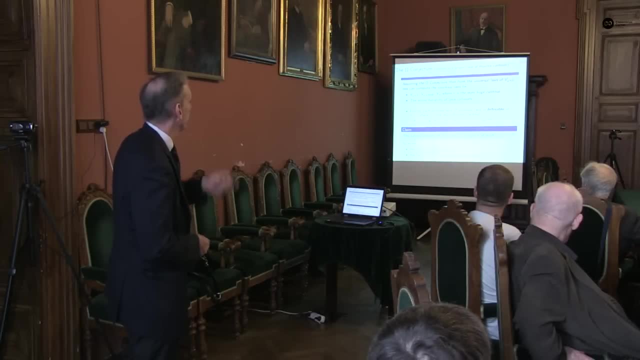 conception of the universe of sets. So either the omega conjecture is false or the generic multiverse option, which seems so appealing, we have to reject. All right. so we made a noble effort. We do some mathematical analysis, We find a conjecture. 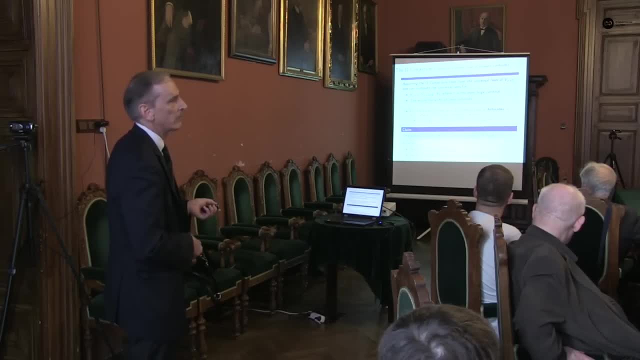 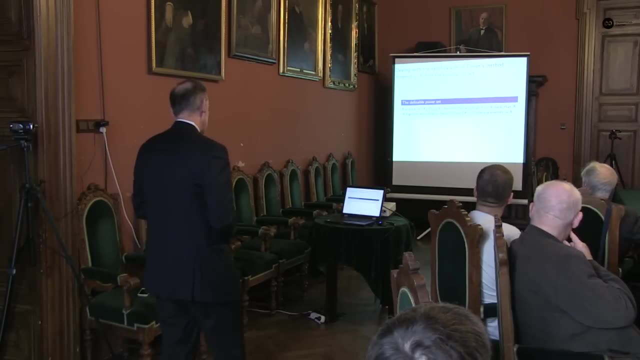 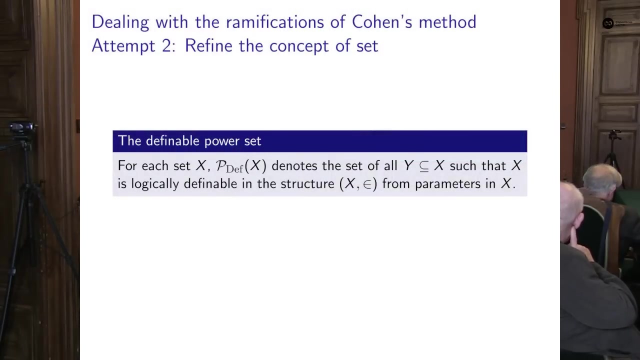 There's a mathematical case for that conjecture, so we have to give up on this option. All right. So what would the second attempt be? We need to refine the concept of set. So how might we do this? Well, it's got to be that power set operation is the problem. 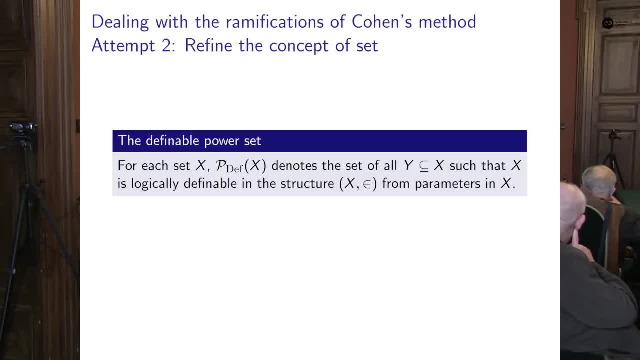 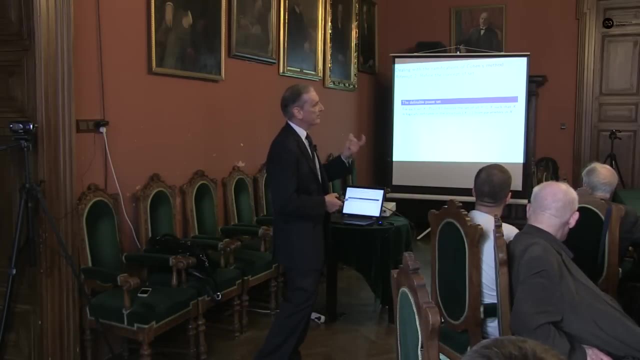 So for each set x, we'll let p def of x denote all the subsets of x which are logically definable in the set x from parameters. And the idea here is: if x is a good set- Perfect- then clearly the subsets of X that you can logically define in X is also a good set. 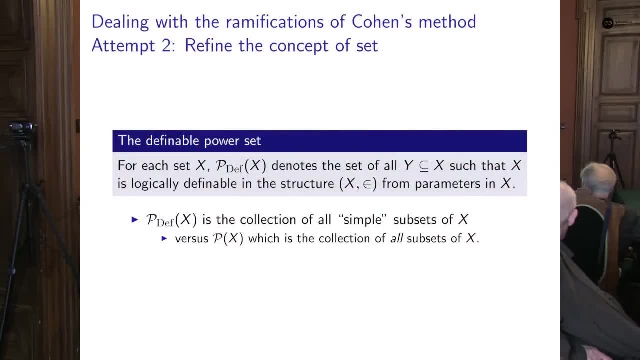 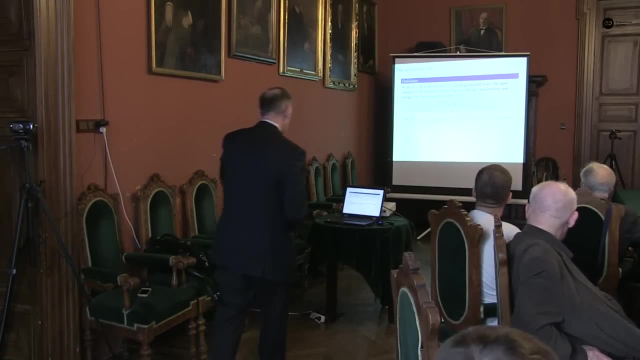 You're not going to get into trouble. So sometimes P def of X is called the collection of simple sets, versus the full power set, which is the collection of all sets. All right, so now I want to change. We're still going to be looking at the definable sets, but let's go back to the reals. 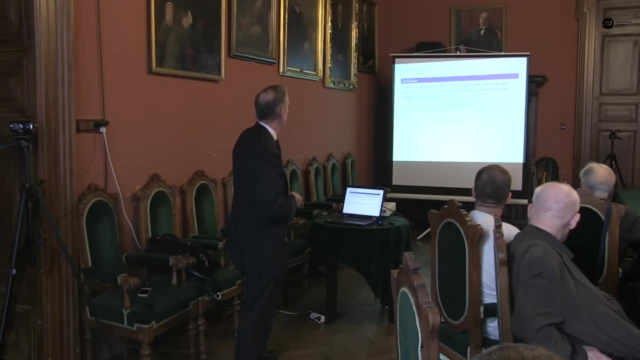 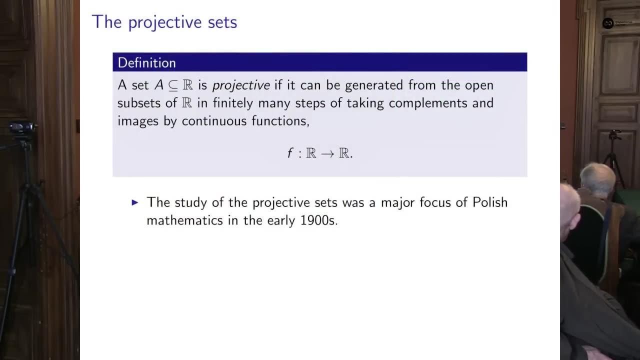 After all, that's where the continuum hypothesis lives. So we'll define a set of reals to be projective if it can be generated from the open sets in finitely many steps of taking complements and images by continuous functions. So the study of the projective sets was a major focus of Polish mathematics in the early 1900s. 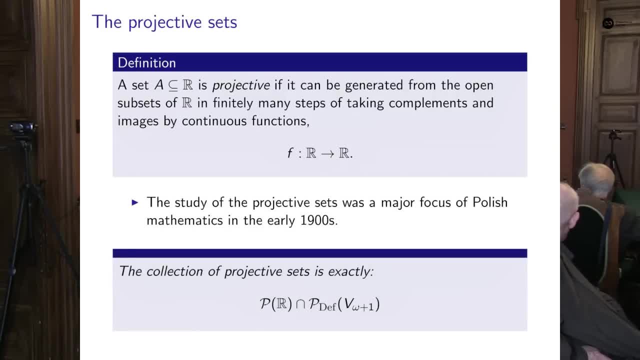 And how could you restate the projective sets in terms of the definable sets? Well, the definable power set, the projective sets of reals, what I defined here are exactly the sets of reals that appear in the definable power set of V, omega plus 1.. 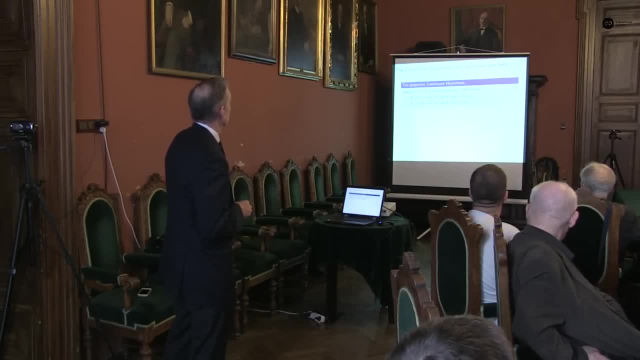 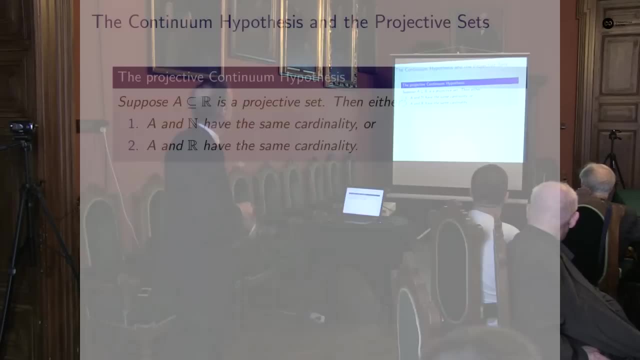 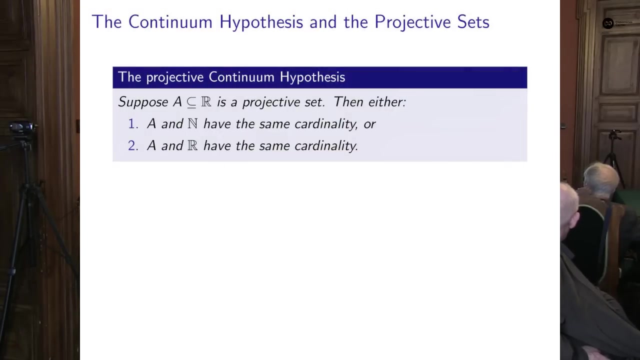 Okay. Well, if you're going to look at a complicated problem, sometimes it's good to look at simple cases. So let's look at the projective continuum hypothesis. If A is a projective set, then either A and N and it's infinite. I should have said: 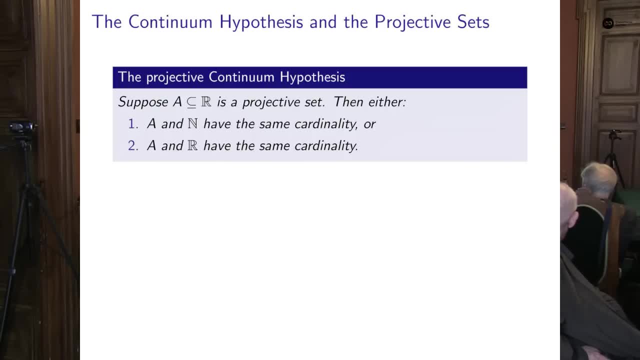 then either A and N have the same cardinality or A and R have the same cardinality, In other words, that the continuum hypothesis holds for projective sets. Well, unfortunately, the actual constructions of Gödel and Cohen show that the projective continuum hypothesis is also formally unsolvable. 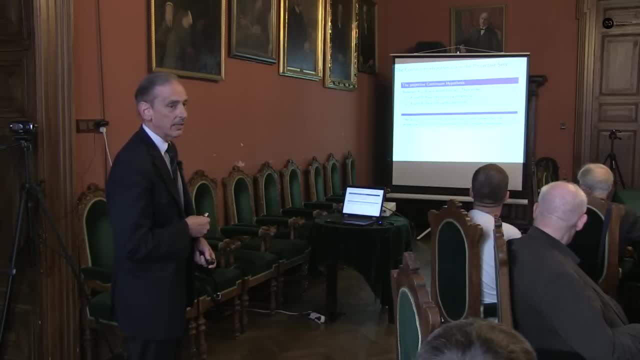 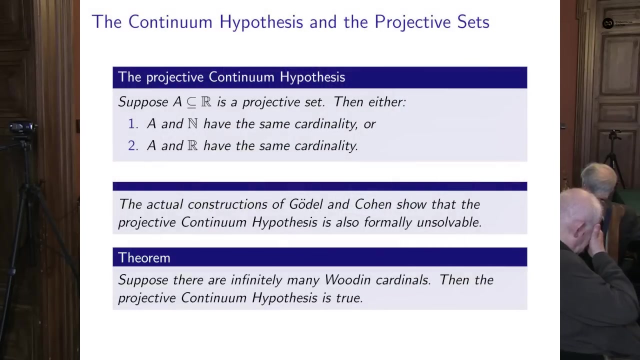 So that's very discouraging that problems occur right away. But there's some good news: The problem of the projective continuum hypothesis has an answer, and there it is. If you assume there are infinitely many wooden cardinals, then the projective continuum hypothesis is true. 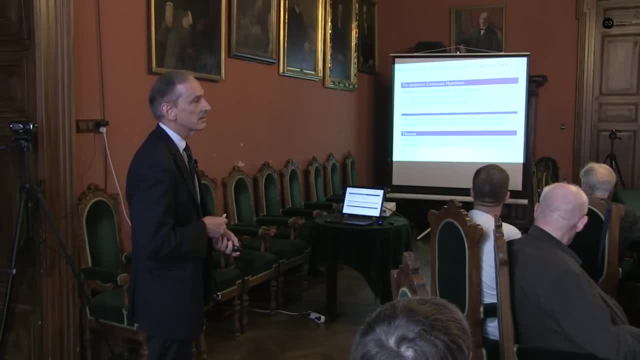 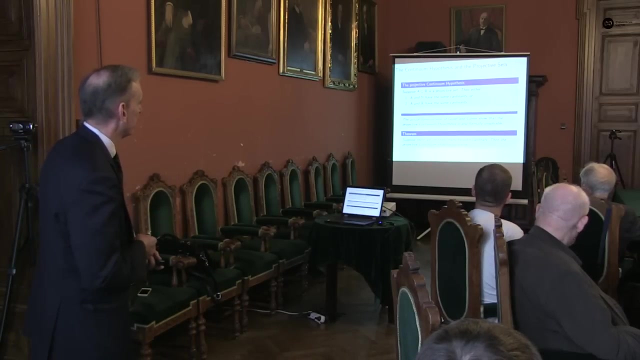 So maybe all's not lost, Okay. So in particular, in the generic multiverse view, once you have large cardinals, then the projective continuum hypothesis is a universal law, And I'm now not as a whole story here. What happened was: we now know the correct theory of the projective sets. 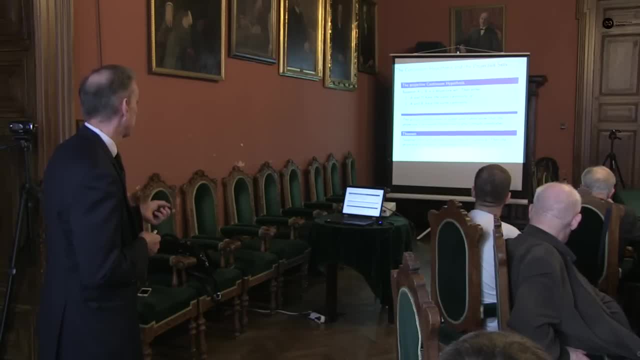 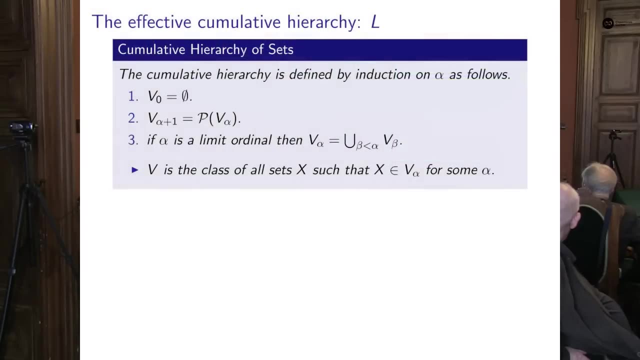 And it originates in the polar school. So, whoops, All right. So looks like we should refine the concept of sets. So recall, this was a cumulative hierarchy where we just collected all sets at a successor step and took the unions at limits. 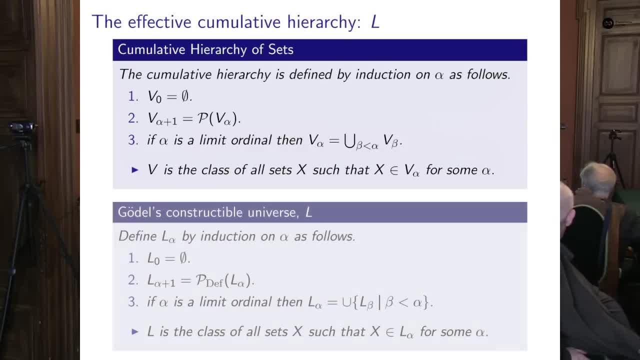 We're now going to refine this by just using the definable power set at this step. So we start with nothing. At a successor step, we take the definable power set And at limit stages we collect union. We just take the union. 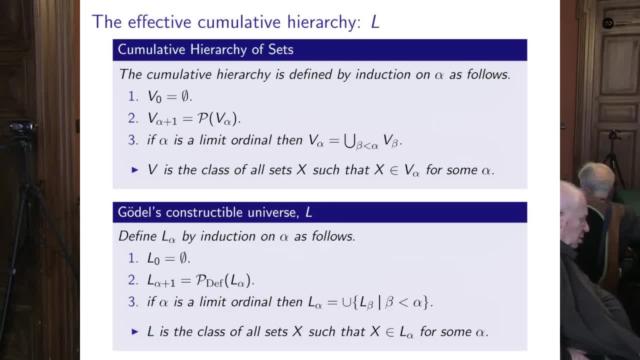 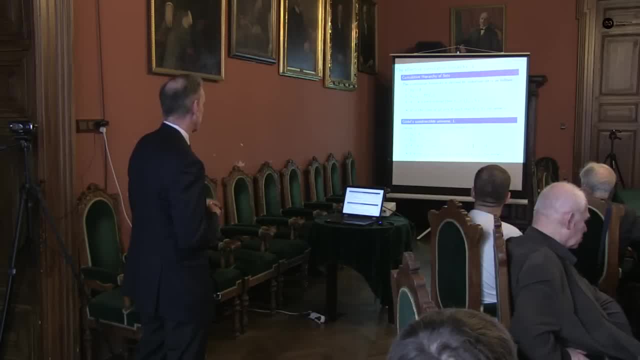 L is the class of all sets that belong to an L alpha. for some alpha, Okay Now L alpha is not V intersect V alpha, L intersect V alpha, L intersect V alpha in general, But the idea is the same, Okay, So we're just going to refine our notion of set. 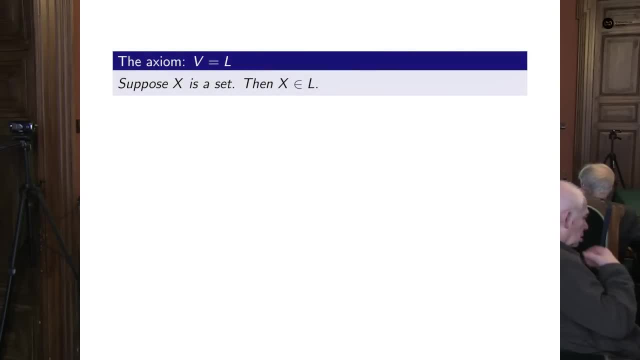 So the axiom V equals L is the axiom that every set belongs to L. Remember, every set belongs to a V alpha. We're now refining our conception. Gödel proved he's the one who first defined L And he showed that the continuum hypothesis holds. 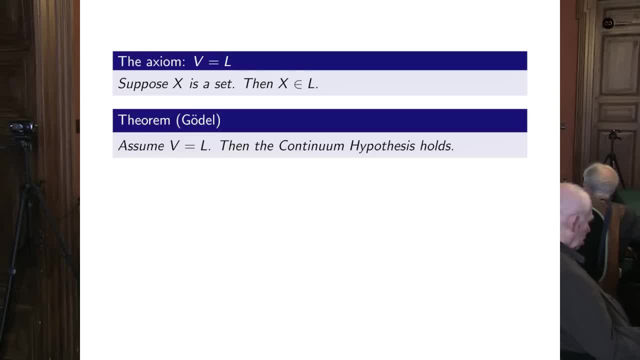 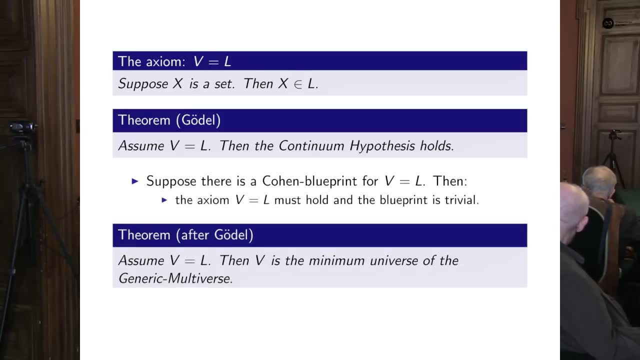 That's how Gödel showed that the continuum hypothesis could not be refuted. Suppose there's a Cohen blueprint in our universe for V is equal to L, Then the axiom V equals L must hold and the blueprint is trivial. So another way of saying it is: if you assume V equals L, then V is the minimum universe. 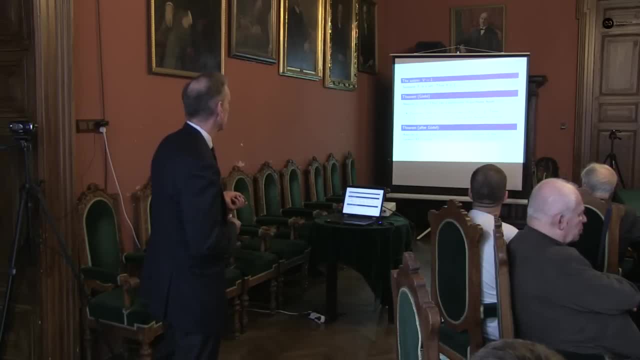 of the generic multiverse. So everything feels like it's holding. It's holding together. So, in particular, if you adopt the axiom V equals L, Cohen's method can do nothing. There's no source of independence that traces back to Cohen's method. 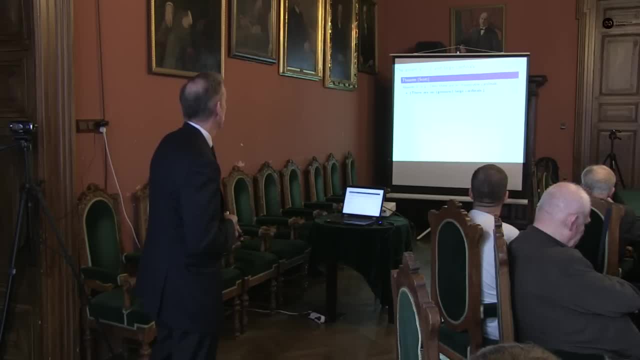 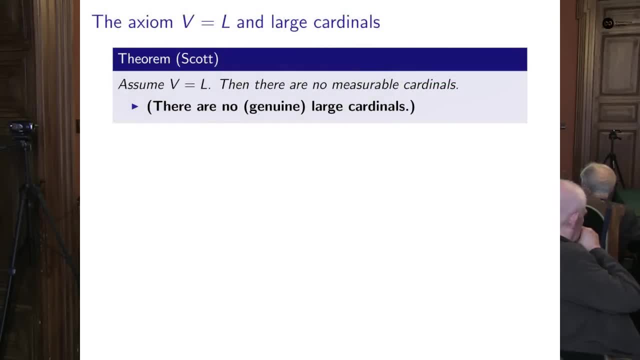 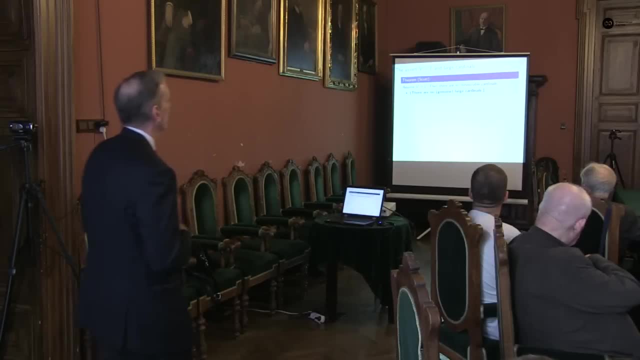 There are no rules. There are no rules. There are no measurable cardinals. That was the first large cardinal on my list. In fact, the modern view is there are no genuine large cardinals, So it's almost as if nature was toying with us. offered us a very attractive view of the 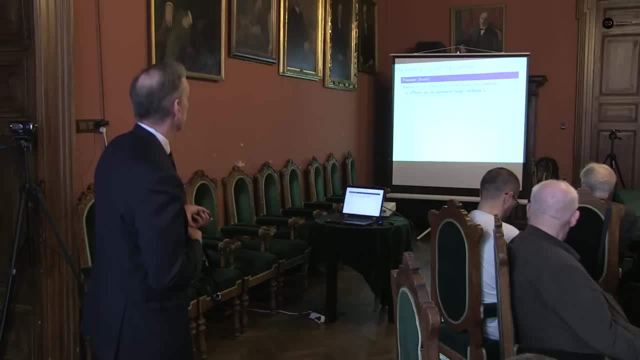 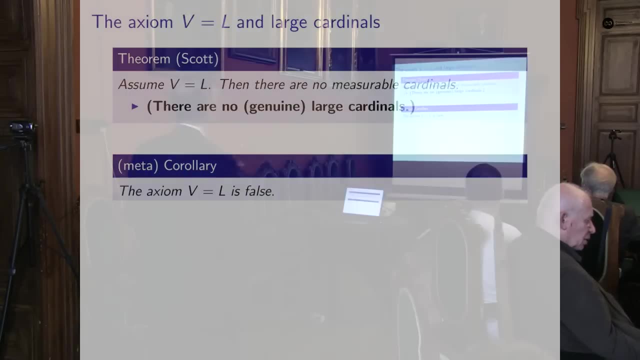 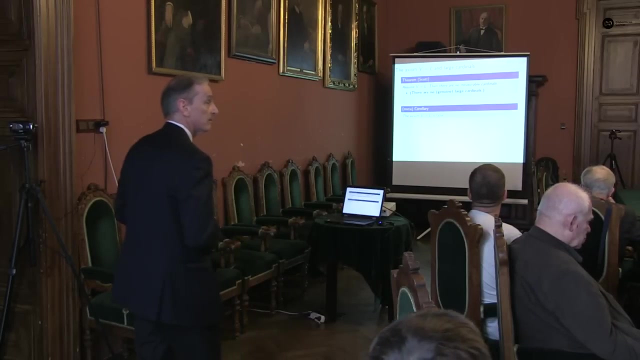 universe of sets, but at the same time gave us the evidence that compels us to reject this view. The axiom V equals L is false because the whole point of set theory is to understand infinity. It's just not true. You can't deny large cardinals, which is not true. 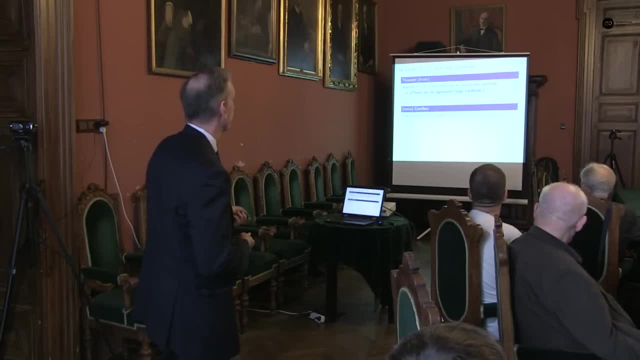 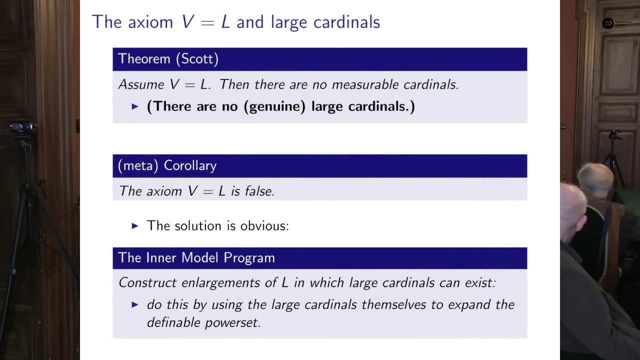 The definable power set is too restrictive, While solutions are obvious. we want to construct enlargements of L in which large cardinals can exist. How might we do this? We need to use the large cardinals themselves to expand the definable power set. 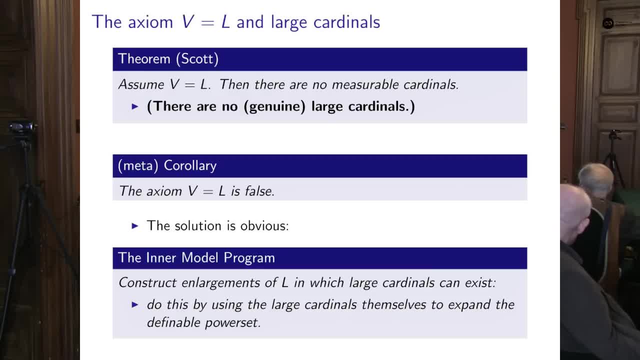 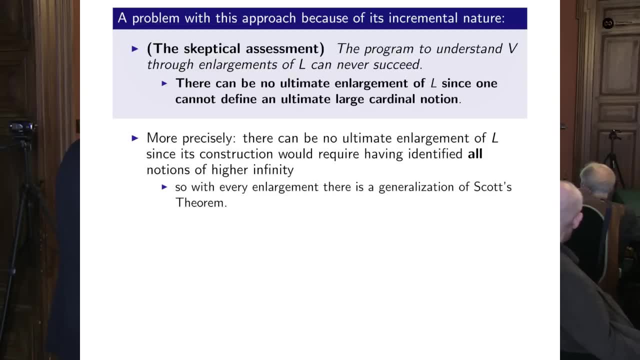 Okay, So that's the intermodal program. Now there's a problem. problem with this approach because it's incremental, And so the skeptical assessment would be: the program to understand the universe of sets through enlargements of L can never succeed. There can be no ultimate enlargement of L. 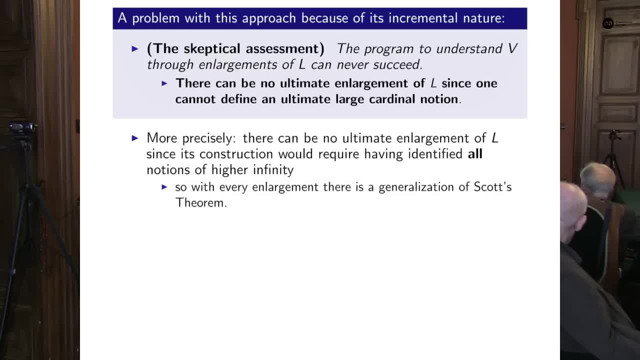 since one cannot define the ultimate large cardinal axiom. So this is the more precise version. There can be no ultimate enlargement of L, since its construction would require having identified all notions of infinity. Because you cannot do that With every enlargement, there would be a generalization of Scott's theorem. 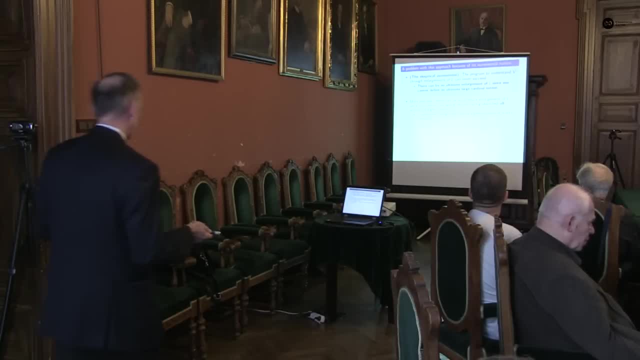 And that's actually what's happened. You build the enlargement of L for one measurable cardinal. That was done in the 60s. You don't have two measurable cardinals. Build the enlargement of L for 20 measurable cardinals. You don't have 21.. 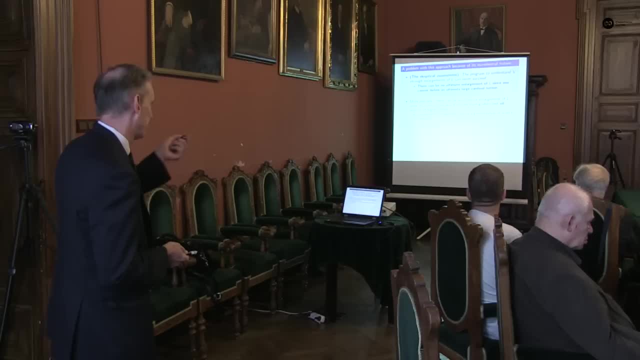 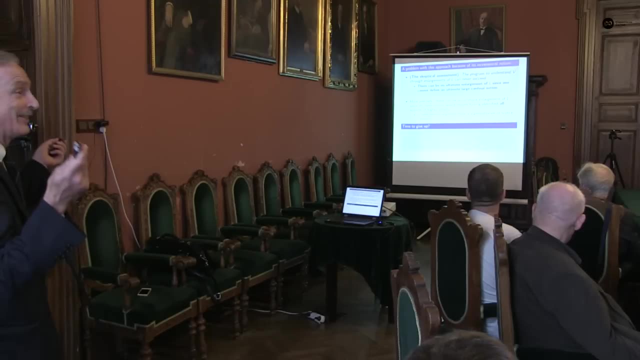 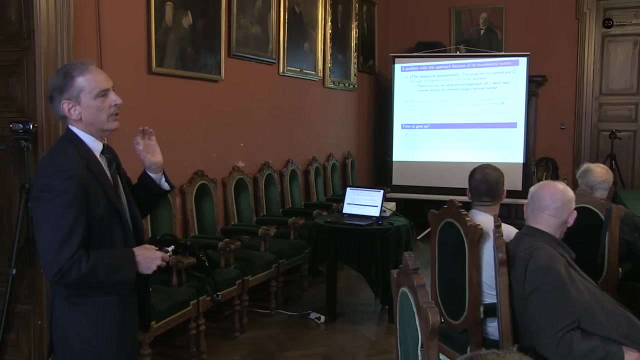 You target a large cardinal, You don't get anything more. And that's the point of the skeptical assessment. Maybe it's time to give up. Maybe it's just there's nothing we can do Now. there's something peculiar about large cardinal axioms. 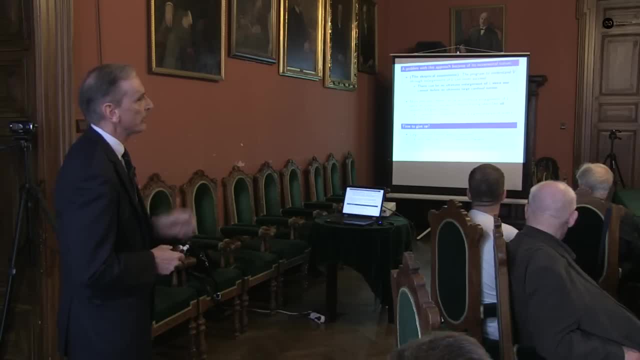 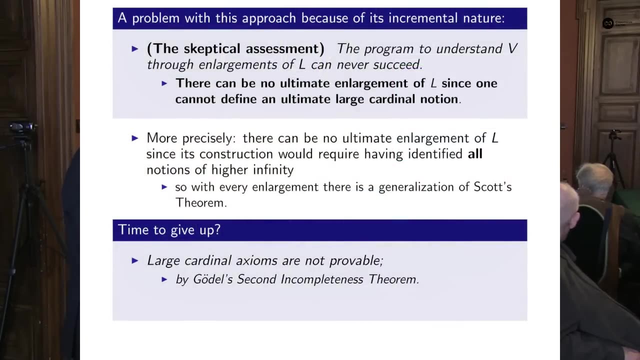 which, unless you're a logician, you're not familiar with. Large cardinal axioms, cannot be proved. That's by Gödel's second incompleteness theorem. But Cardinal axioms are falsifiable, They may be contradictory. So if measurable cardinals are consistent, they don't lead to a contradiction. that's a truth about the physical universe. Search as much as you want, you will not find a contradiction. So if you want to take the position that large cardinals exist, they have falsifiable. their existence has falsifiable consequences. 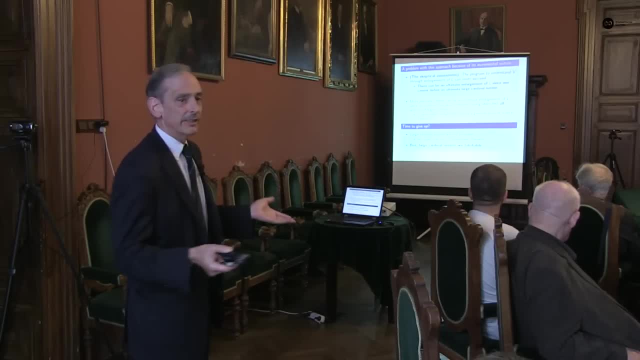 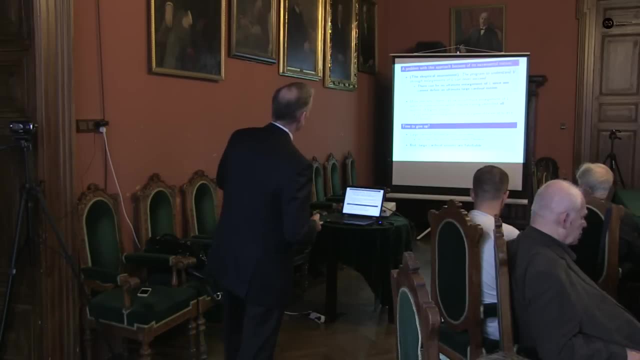 on finite sets. How else can you explain those? There's no way that we know of to explain why measurable cardinals are consistent. That doesn't trace back to. measurable cardinals exist in some sense. So the large cardinal hierarchy which has emerged as a robust 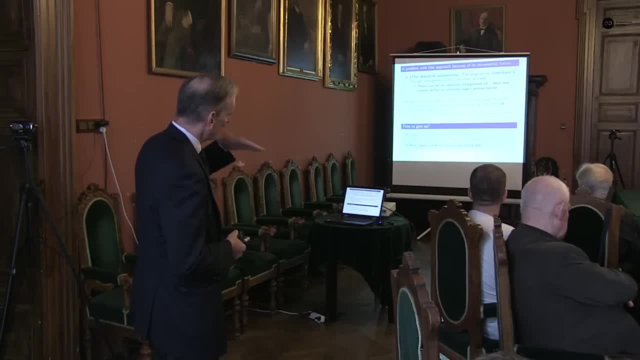 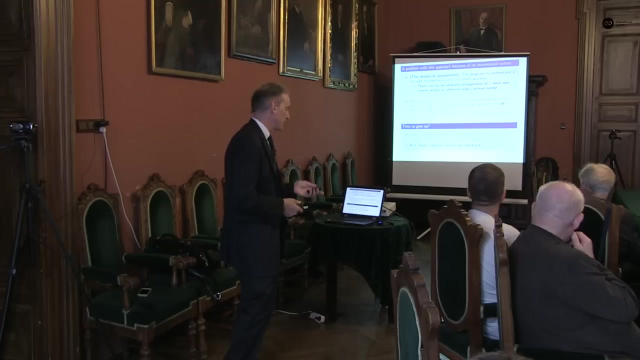 conception is an increasingly stronger sequence of predictions about the universe. So, and the only way to account for this is to conceive of them, just to conceive of set theory. So we can't give up. If we give up, we can't explain something. 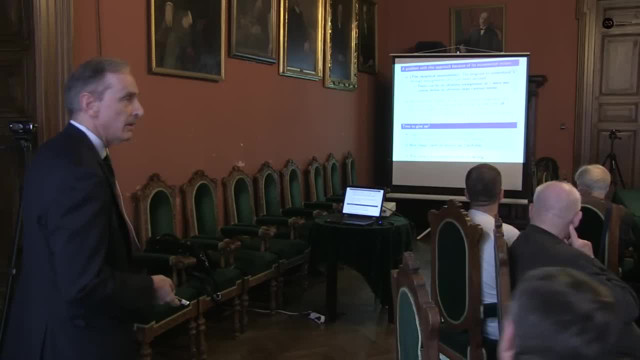 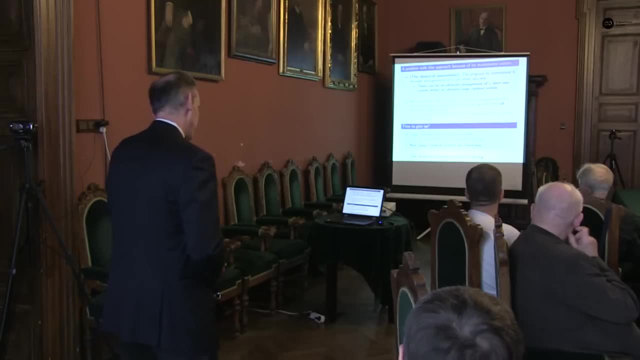 that seems meaningful, not only in number theory but in this universe. I mean. I have stated to be controversial infinitely many wooden cardinals. we know exactly where it is in this hierarchy. It has to do with the axiom of determinacy. 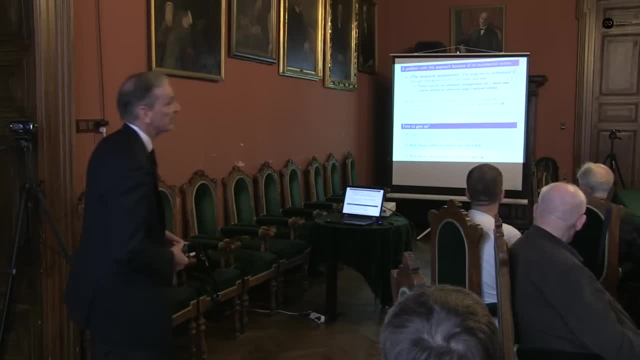 So this was an axiom introduced by Michelsky in 1960. And it's kind of the intermediary that solves the problems about the projective sets. When I was a graduate student it was highly dubious whether this was a consistent axiom. So by transference, the consistency of infinitely. 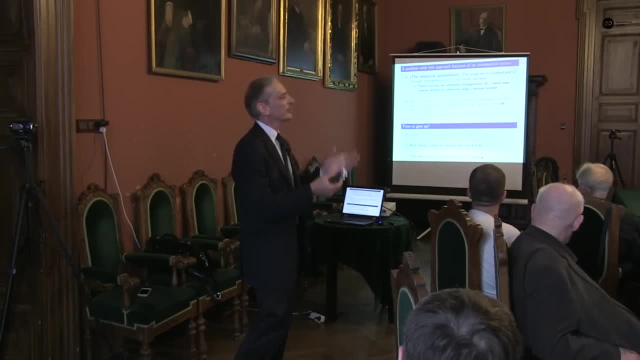 many wooden cardinals is a dubious fact. But now we understand the whole picture and so we have to take the position that it is consistent. So we are making a prediction. Go out as far as you want. in the future you will never refute this axiom. 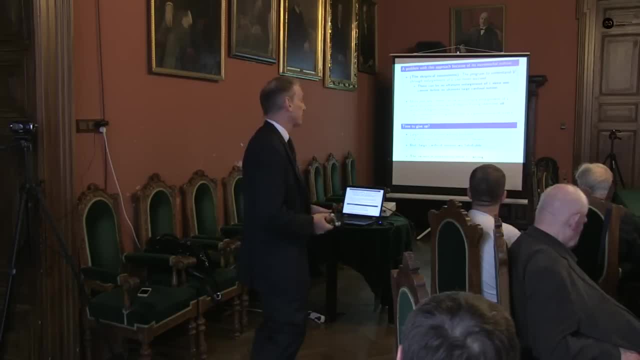 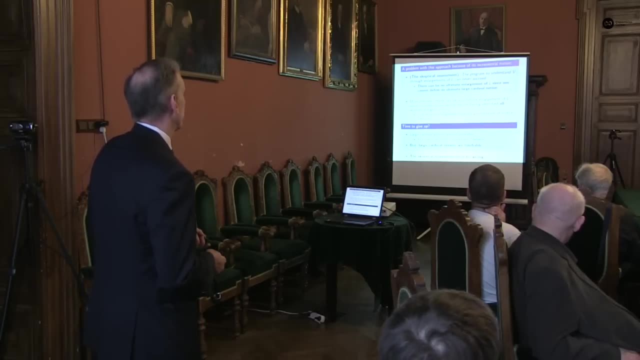 How do you explain that? Now, maybe the prediction's wrong, but if it's not, how do you explain it? All right, so if these falsifiable predictions turn out in fact to be true, and the only way to account for them, 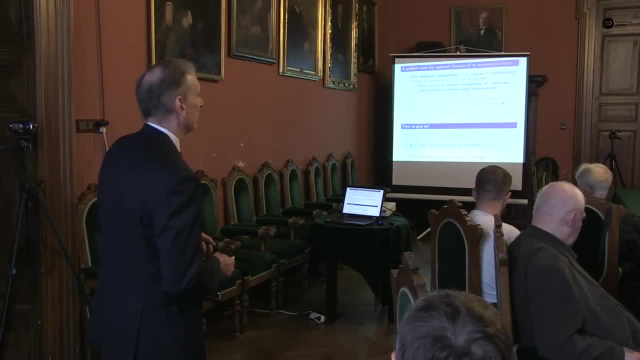 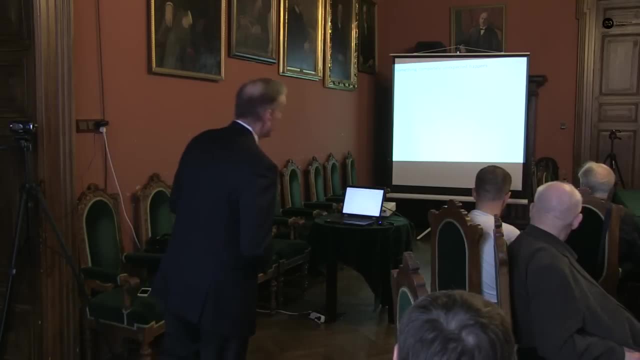 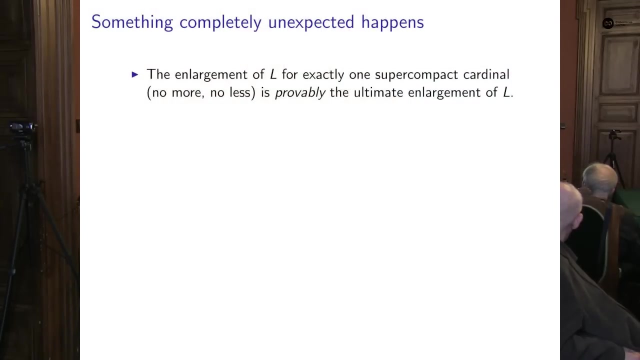 is to conceive of the universe of sets, then this skeptical assessment must be wrong And it is. Maybe something completely unexpected happens If you take the enlargement and valve for one super-compact cardinal. now, I gave you that list. Super-compact cardinal is around in the middle. 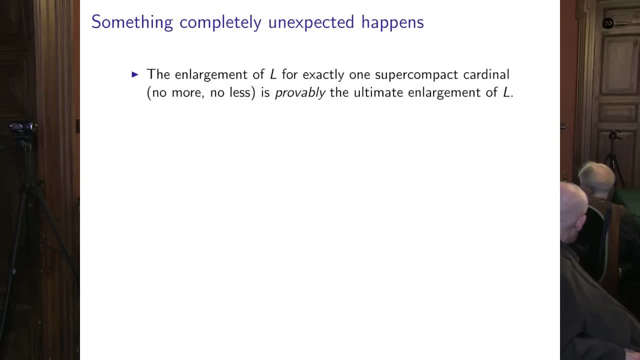 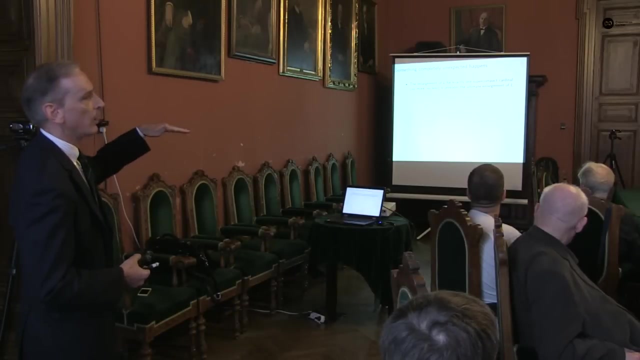 So it's nowhere near the top. There is no top. But the enlargement valve for exactly one super-compact cardinal, no more, no less, is provably the ultimate enlargement. So that skeptical view that you target one level and you don't get anything more is wrong. 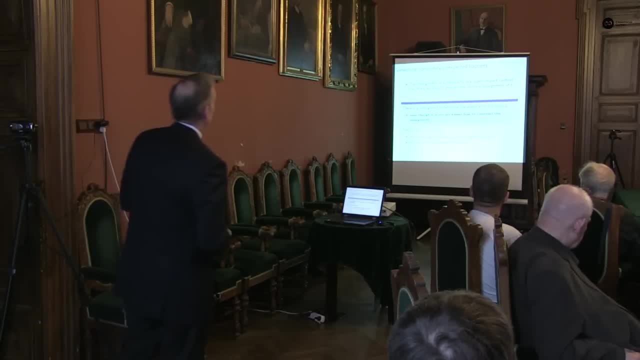 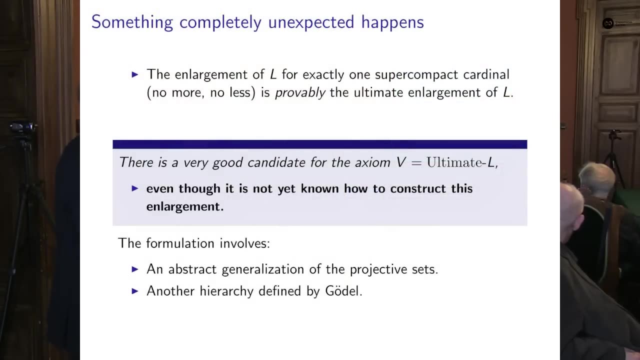 So completely a complete surprise. Okay, there's a very good candidate now for the axiom. V is ultimate L, even though we don't know how to construct it yet, And the formulation involves a generalization of the projective sets and another hierarchy. 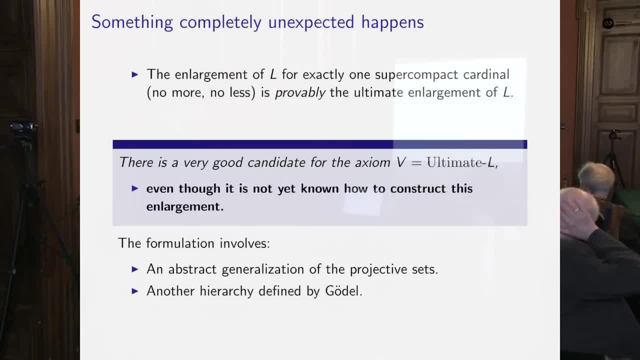 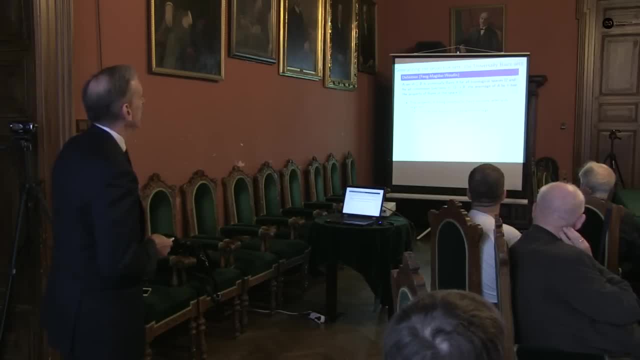 defined by Gödel. So I hope you bear with me. I'm going to show you what this formulation is. Okay, so I have to make some definitions. So how are we gonna generalize the projective sets abstractly? So this was done 20 years ago. 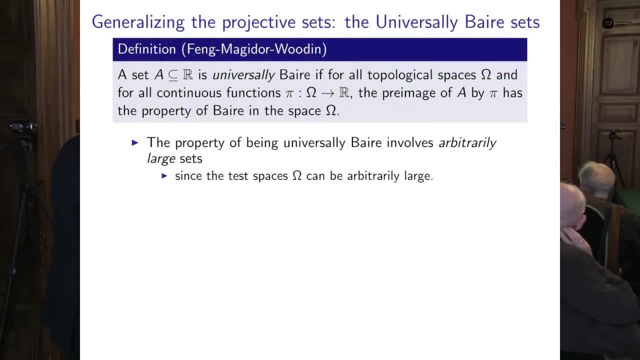 This notion of universally bare sets. So here's the definition. If you're not a mathematician, this may not make a lot of sense. Sets universally bare if it's continuous pre-images in any topological space have the property of bare in that space. 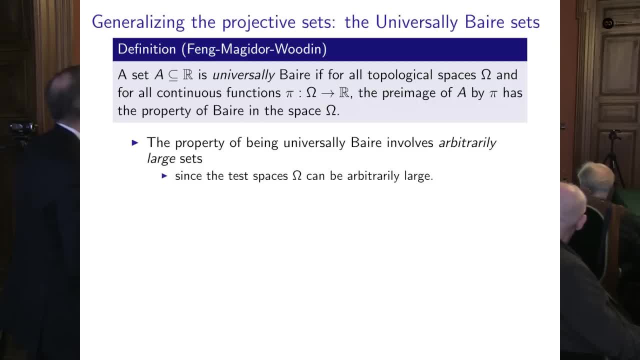 That means they differ from an open set by a meager set Doesn't really matter what the definition means. It's important to note that being universally bare involves arbitrarily large sets. because these test spaces can be arbitrarily large, The continuum hypothesis holds for all the universally bare sets. 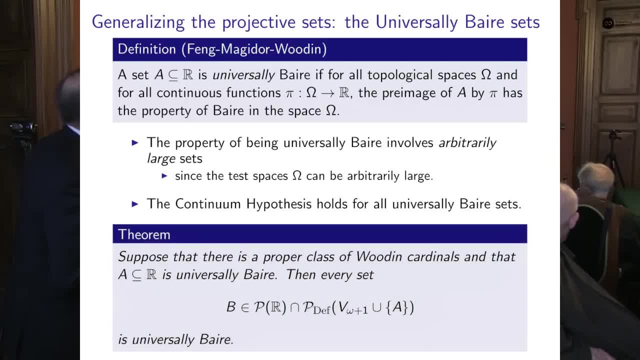 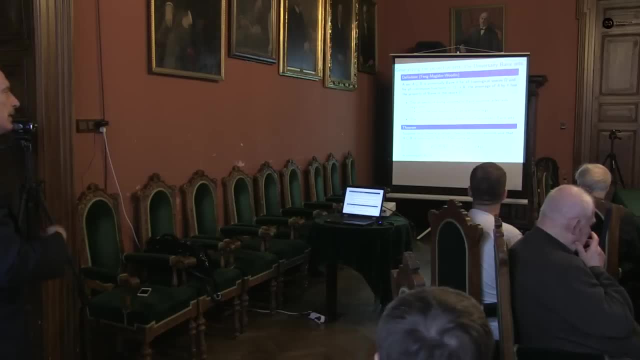 That's just a theorem. If you assume you have a proper class of wooden cardinals and you have a universally bare set, everything in the definable power set that you would generate by throwing A in at the bottom is also universally bare. So that's the relativization of the projective sets to A. 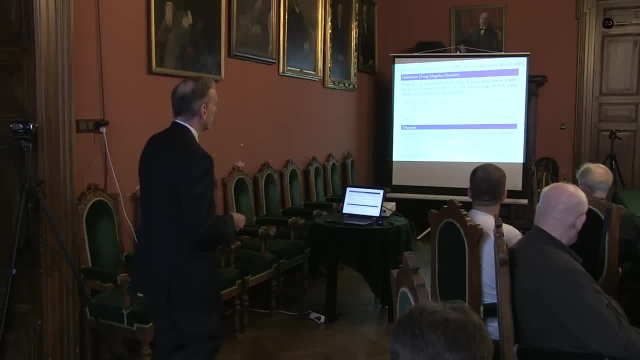 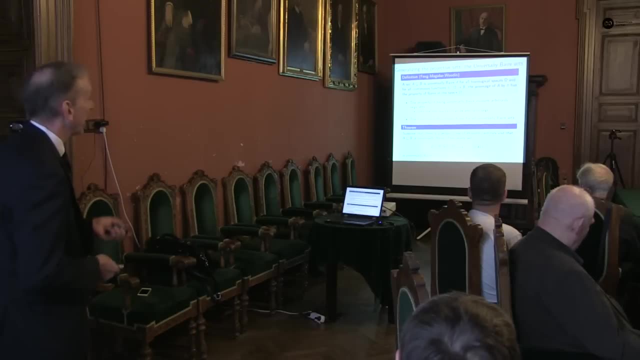 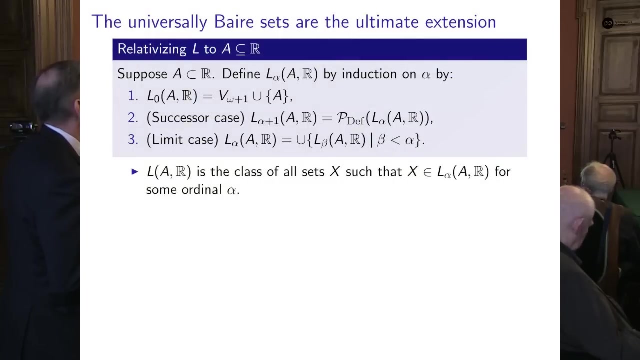 In particular since every projective set is here. every projective set is universally bare. So this is looking like a good generalization, at least a generalization of the projective sets, And they really are the ultimate extension And there are several ways that one can make that precise. 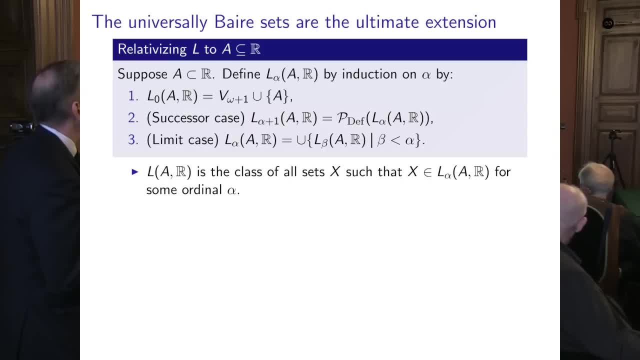 First of all, given a set of reals, you can relativize Gödel's construction of L to A in R, And that's how you do it: You just start. You start with that set I just mentioned. At the successor stage you take the definable power set. 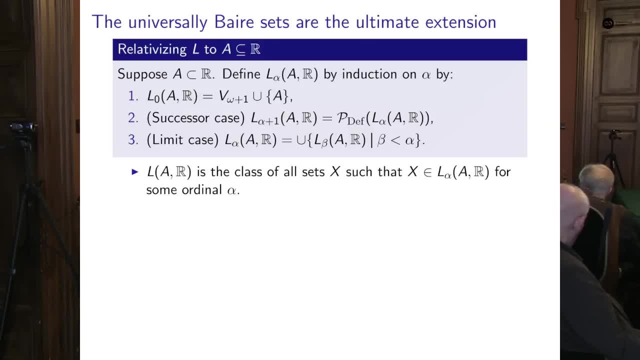 At the limit stage you take unions. L of A and R are all the sets that you get. this way, If we let A be empty, the sets in L of R are genuine transfinite extension of the projective sets. And then the theorem I stated on the last slide. 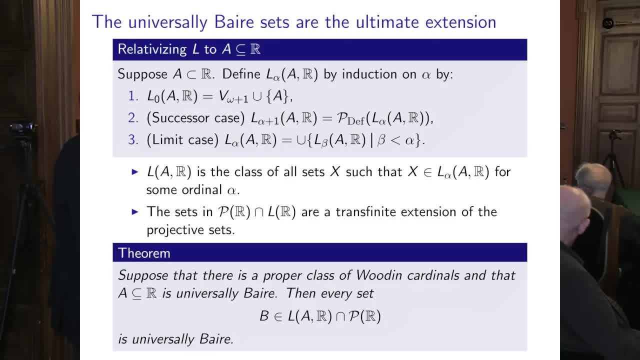 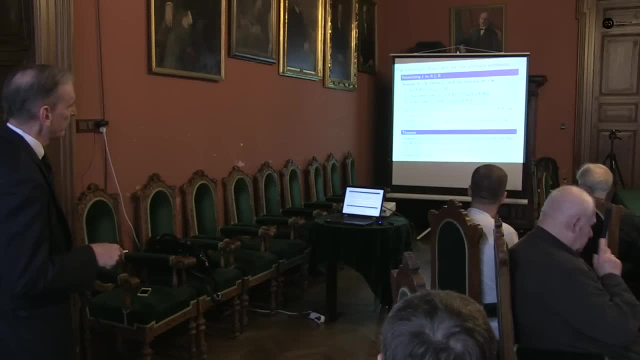 generalizes to this much richer collection. Suppose you have a proper class of wooden cardinals and A is universally bare, then every set that you can generate from A by passing to L of A in R is universally bare. It's a very rich collection because within this universe 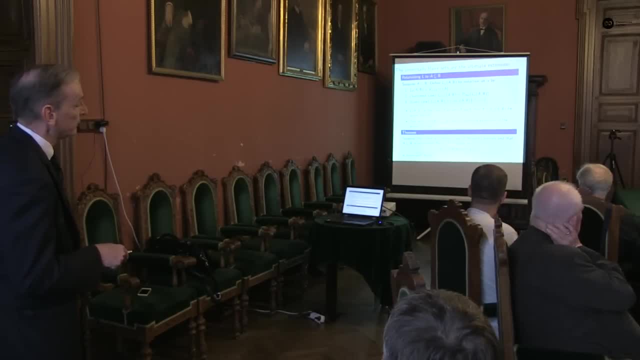 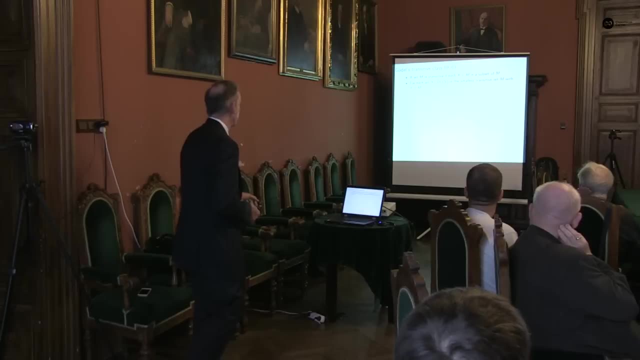 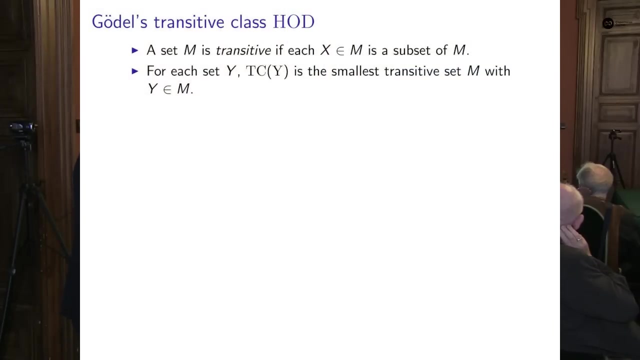 all the axioms of set theory hold, except for the axiom of choice. So the universally bare sets have tremendous closure properties. Here's the other hierarchy that Gödel introduced. It's called Hobson, It's called HoD, That's hereditarily ordinal definable. 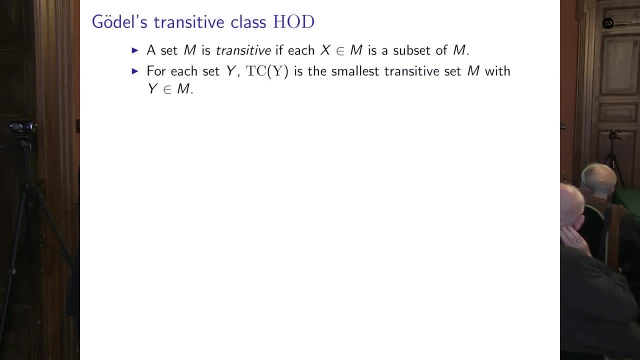 I have to introduce another definition. first, An M is transitive. if every element of M is a subset of M, The V alphas are all transitive. Every ordinal is transitive. Every set has a transitive closure: Tc of y. 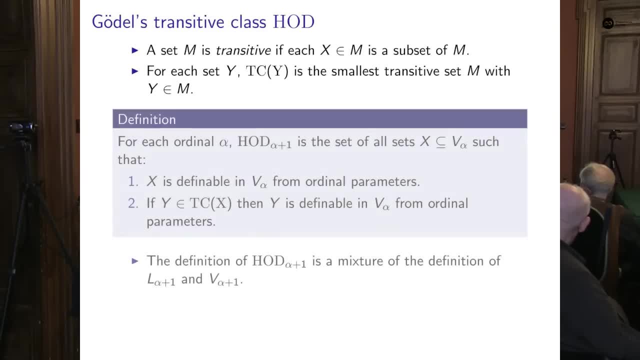 It's the smallest transitive set to which it belongs. And now we're going to mix the definition of L alpha plus 1 and V alpha plus 1.. HoD alpha plus 1 is the collection of all subsets of V alpha, Such that x is definable in V alpha from ordinal parameters. 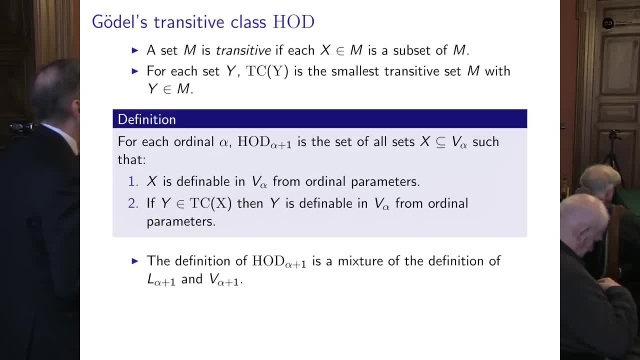 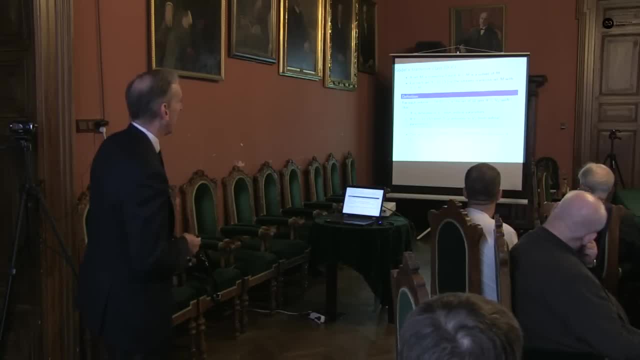 along with every element of the transitive closure of x. So it really is a mix. Instead of remember L alpha plus 1 was all things definable From L alpha, you could have actually done ordinal parameters and gotten the same thing. 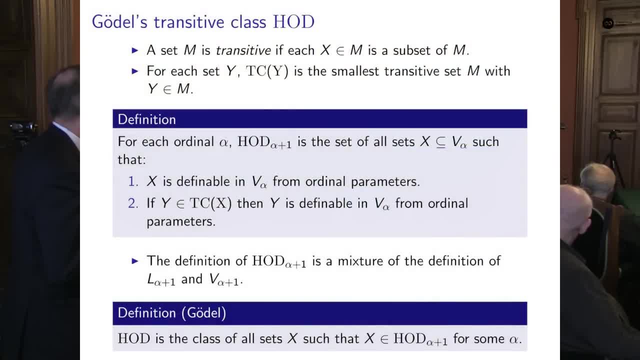 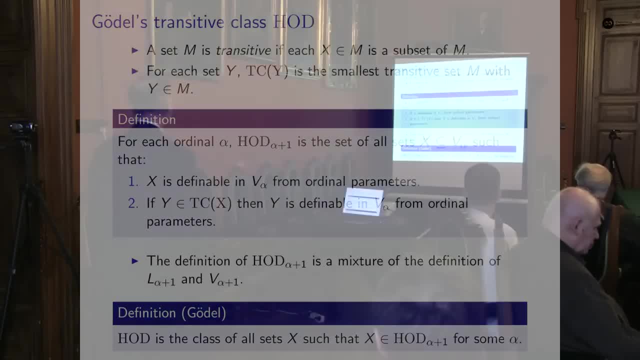 All right, a HoD is. this is what Gödel defined. HoD is a class of all sets such that x belongs to HoD, alpha plus 1 from some ordinal alpha. Gödel introduced HoD in his Bicentennial Lecture. 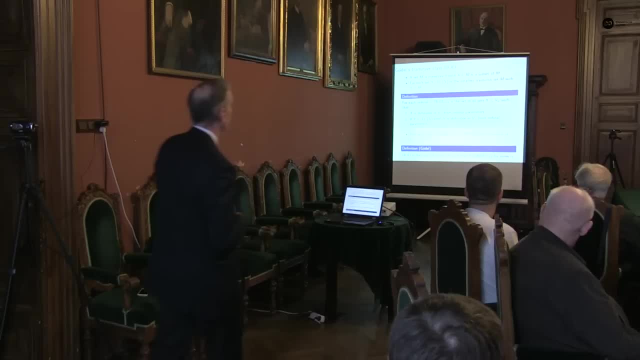 at Princeton in the 40s, the Princeton Bicentennial, And he introduced it as an alternative way of showing that the axiom of choice cannot be refuted by the other axioms of set theory, because this whole definition does not require the axiom of choice. 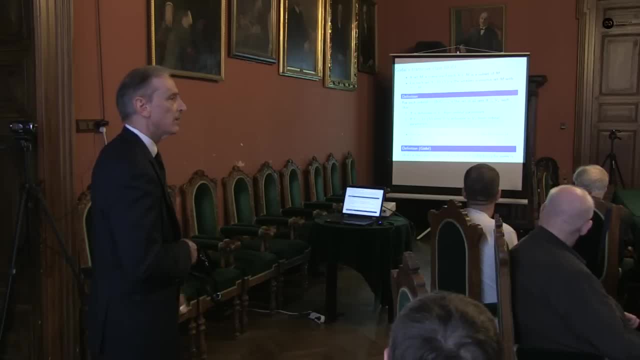 And yet this, the axiom of choice, holds here. So in other words, if you have a universe in which all of the axioms, except possibly the axiom of choice, hold, you can build a universe in which the axiom of choice holds as well. 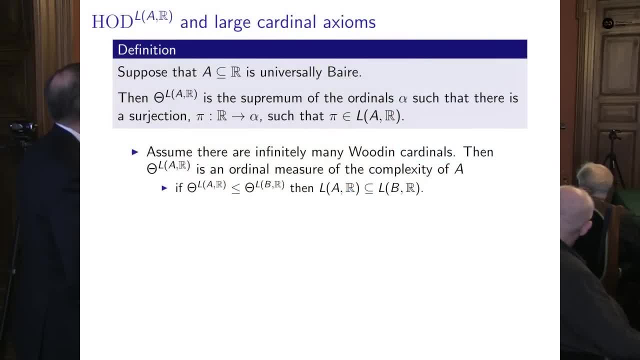 All right. so I need to connect the HoD, universally-bare sets and large cardinal axioms. So I think this will be the last definition I'm going to make you sit through. If A is universally-bare, theta of L, of A and R. 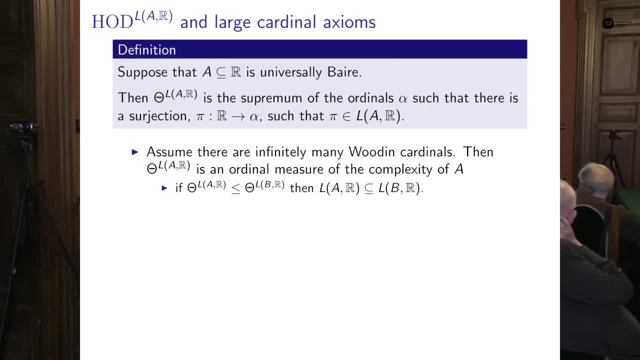 are the supremum of the ordinals on to which you can map the reals by a function that's in L, of A and R. It's a measure of the size of the reels within this sub-universe of the universe of sets. 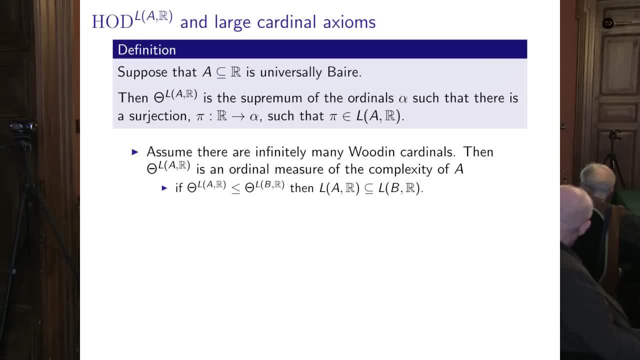 And what's interesting is that if you have just infinitely many wooden cardinals, this ordinal, it's an ordinal, is an ordinal measure of the complexity of the universally bare set. One way of making that more precise: if the theta of L, of A and R 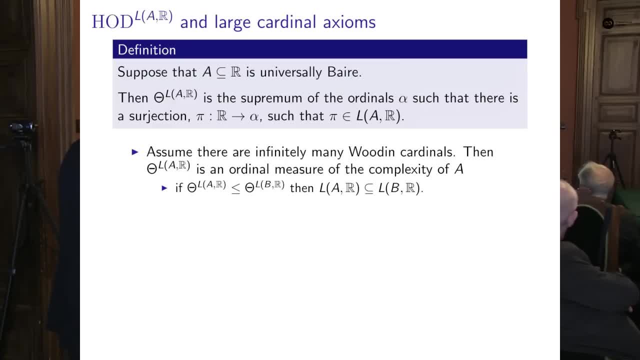 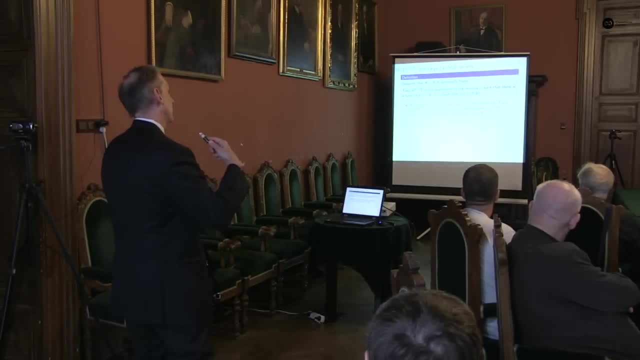 is less than or equal to the theta of L of B and R, then L of A and R is actually a subset of L of B and R. So this is a very so. it really is an ordinal measure of complexity. Now you need the large cardinal assumption for this. 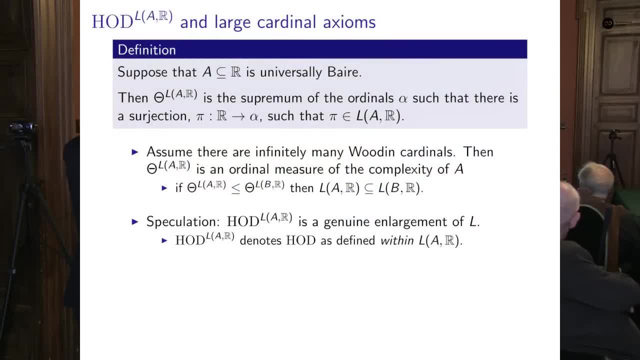 So the speculation would be that the HOD computed in L of A and R, which must be a model of choice, is a genuine enlargement of L, Where HOD- that's what this denotes. it denotes define HOD, not in V as I just defined it. 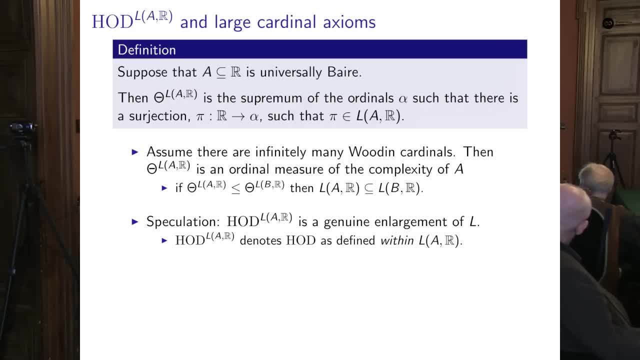 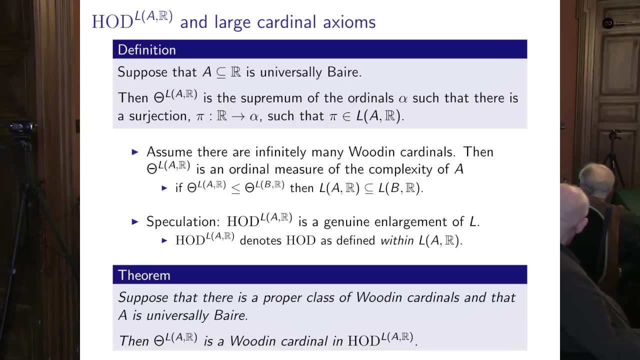 but living inside this universe. Well, we better have large cardinals there, or this isn't going to be very useful. And there's a kind of surprising theorem and it's like 20 years ago, Suppose you have a proper class of wooden cardinals. 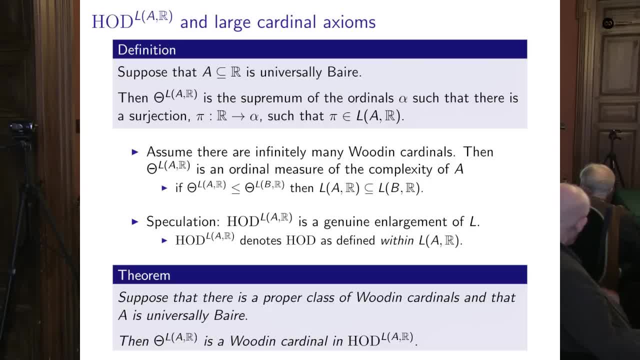 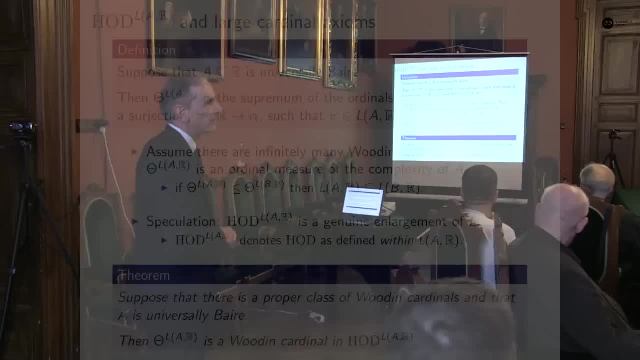 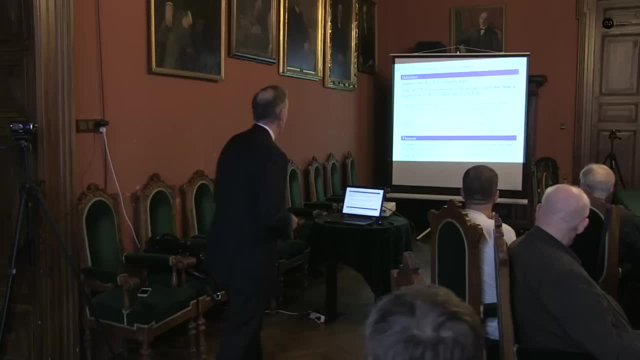 and A is universally bare, then this ordinal that measures the complexity of A is actually a wooden cardinal in this sub-universe of the axiom of choice. So these candidates for genuine enlargements can at least have wooden cardinals, All right. well, when you put everything together now, 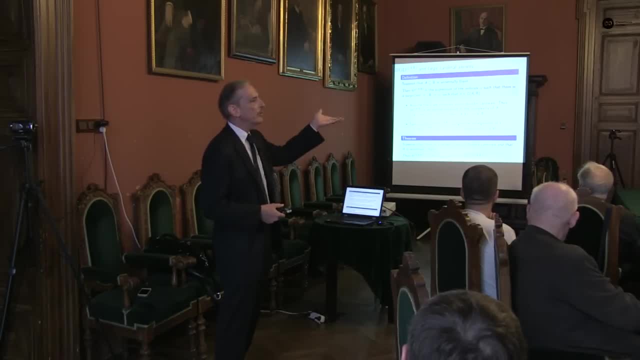 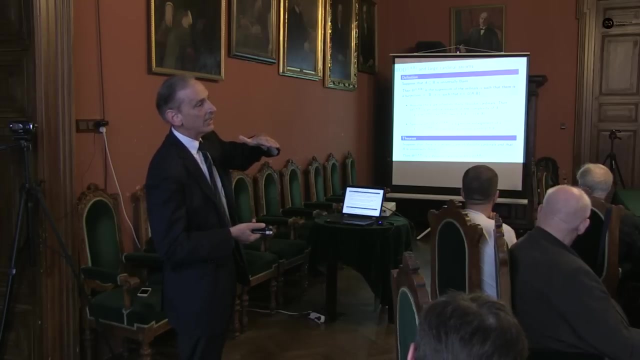 if you have an enlargement of L, you expect truth to reflect an enlargement of L. think back to the definition of L is layered And reflection would tell you that within the enlargement of L, any sentence- that's true- would have to reflect. 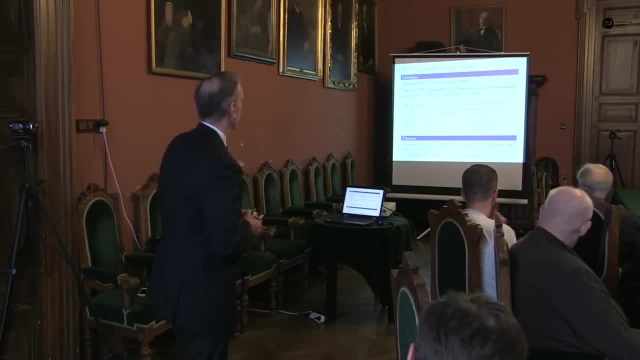 to being true at some level. Well, wait a minute. We have an abstract definition now of levels. We don't need the level by level. We don't know anything about these models. We expect them to be enlargements. We have an ordinal attached to these models, namely: 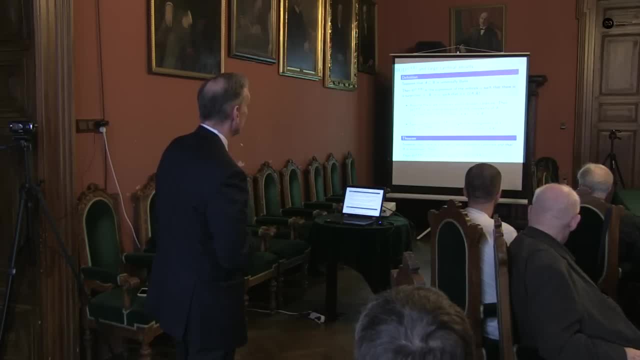 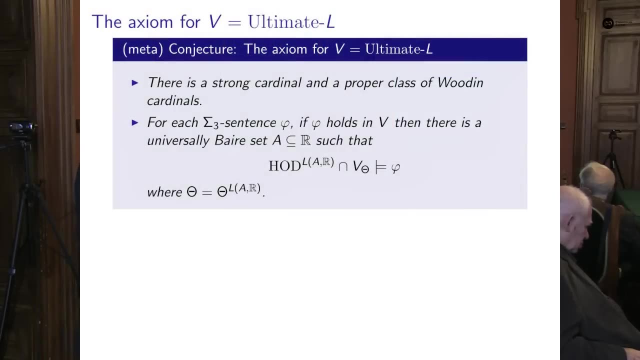 the ordinal of the parent universe. So that gives us a candidate for V is ultimate L: Okay, So this is the candidate. I need some large cardinals to initialize everything: Strong cardinal, which I didn't define. Well, I didn't define wooden cardinals either. 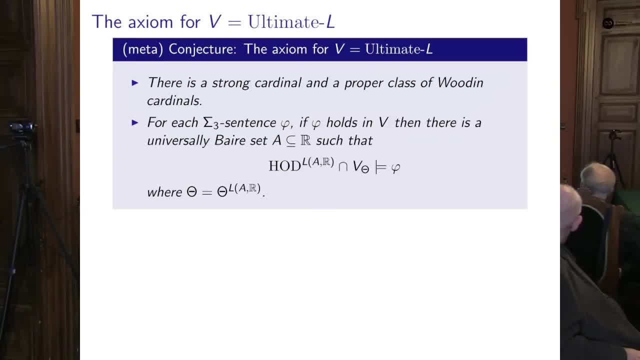 And basically all this says is that any sentence that's true in V reflects to be true into one of these models. And because I want to make this a first order axiom rather than a scheme- and there are other reasons as well- I'm going to restrict the complexity of the sentences. 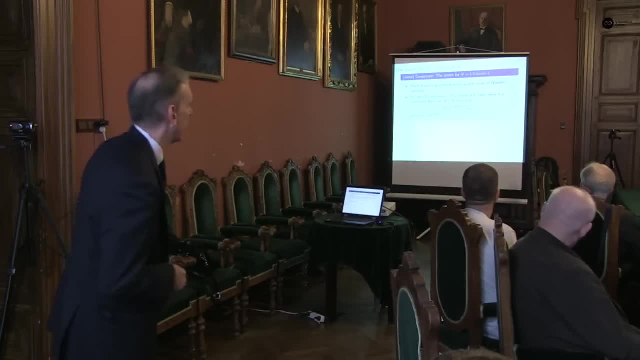 to what are called sigma three sentences, But that doesn't really matter. There's the axiom, It's you know. I mean it can be defined to a first year student in logic, A specific axiom. Suppose now we could analyze this axiom. 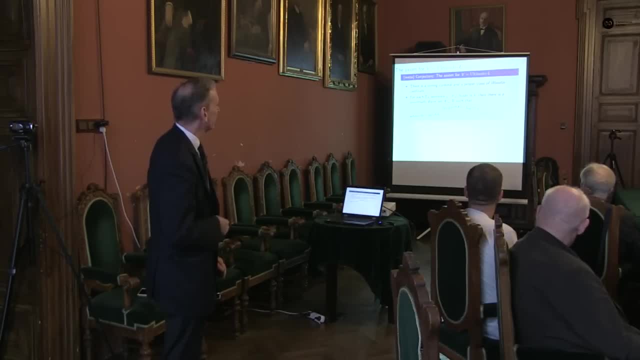 even though we don't know how to build this enlargement- And it's going to be this, this determinacy axiom that I alluded to. that gives us a lot of ability to analyze this axiom before we've even understood how to construct ultimate L. So one thing one can prove is: 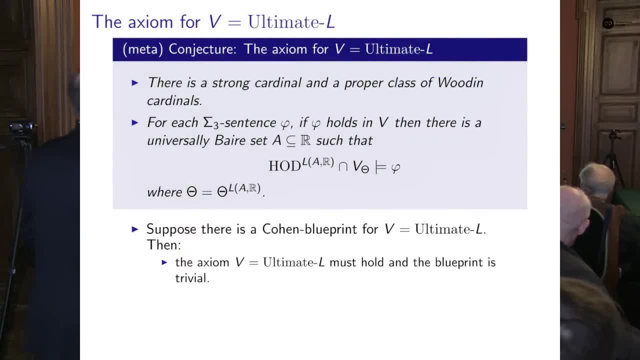 that if you have a Cohen blueprint for V as ultimate L for this axiom, then V as ultimate L must hold And the blueprint is trivial. Okay, Well, that's good. That means that Cohen's method of forcing is not good. That means that Cohen's method of forcing is not good. 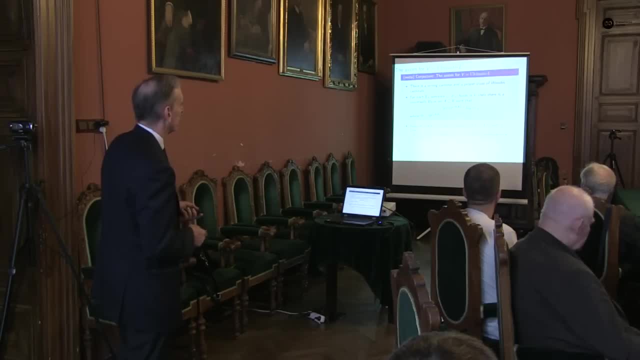 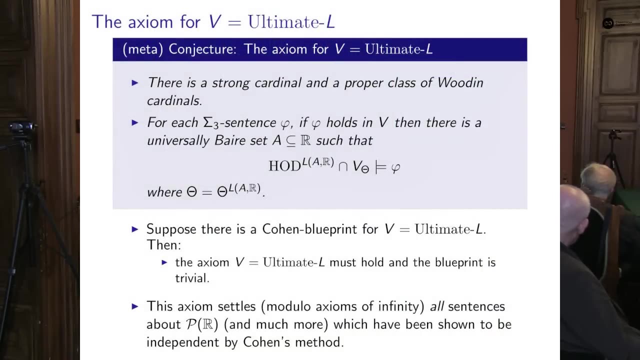 That means that Cohen's method of forcing is not going to affect the universe in the context of this axiom. So the axiom settles modulo. axioms of infinity. That will be the only ambiguity. now, All sentences about P of R and much more which have been shown: 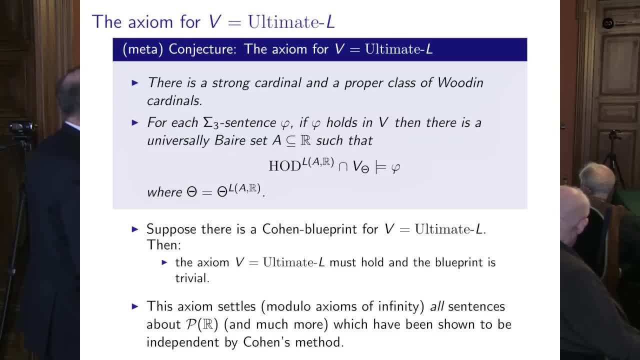 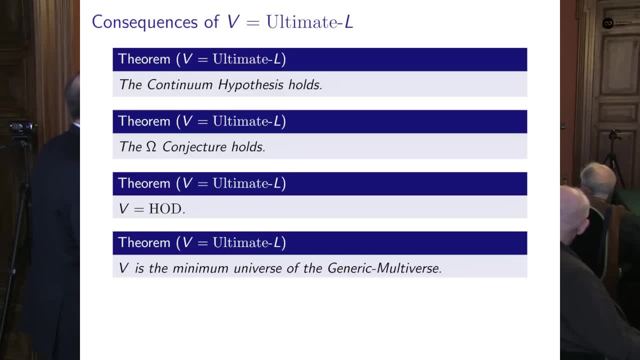 to be independent by Cohen's method. Okay, so here are some known consequences. If you assume V, this axiom that I wrote down, V is ultimate L, the continuum hypothesis holds The omega continuum holds. Remember that was the conjecture that forced us. 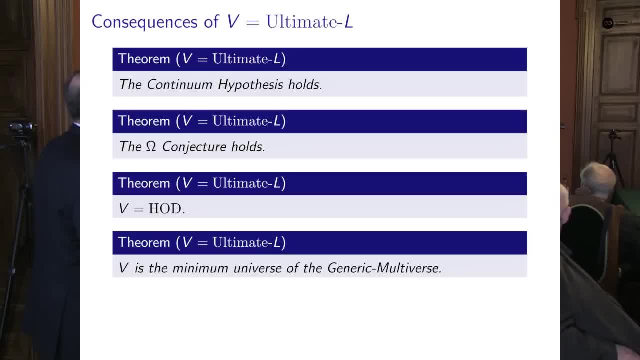 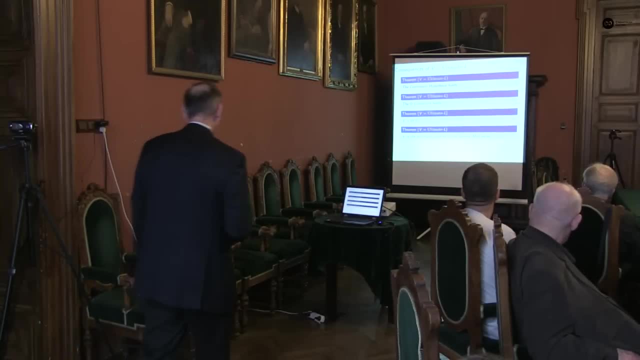 to reject the generic multiverse view More. now I'm getting into more sophisticated consequences. V is equal to hot, And then V is also the minimum universe of the generic multiverse. That was the thing about the Cohen blueprint, But now we have a key question. 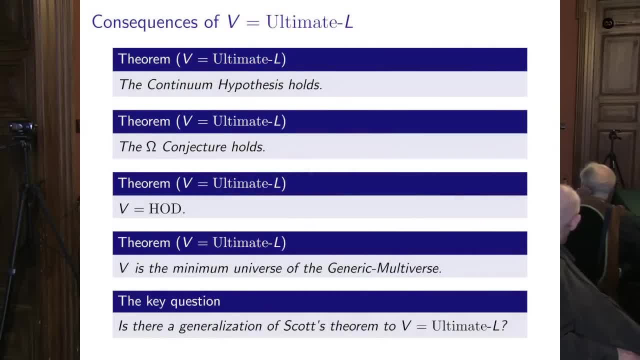 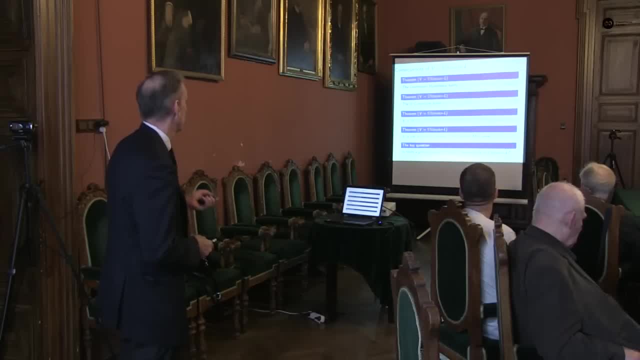 Maybe there's a Scott's theorem. I mean, how can we be sure there isn't a generalization of Scott's theorem to this axiom, In which case we've made no progress? So that's what the next few slides will deal with. 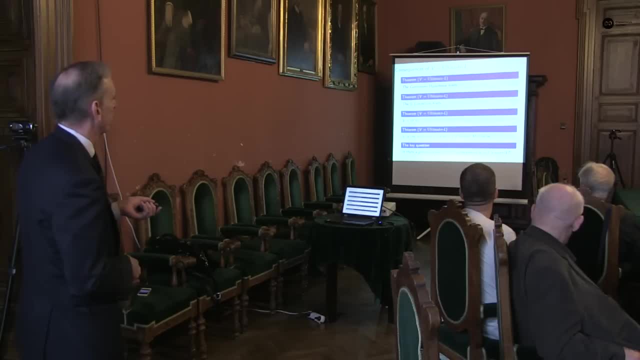 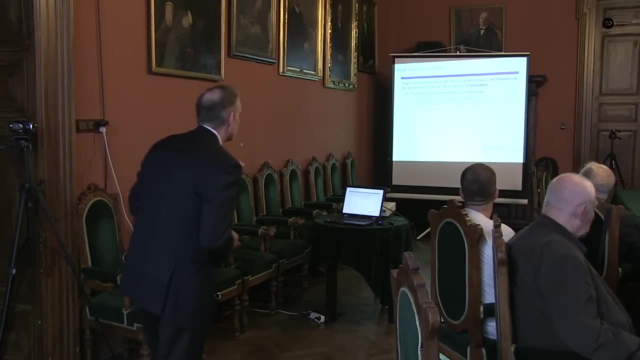 I have to make some more definitions and give you a flavor of how we even conceive of enlargements of L. Does that mean something that I need to worry about That? Oh, It took care of. oh, Which button. I only know how to go forward and back. 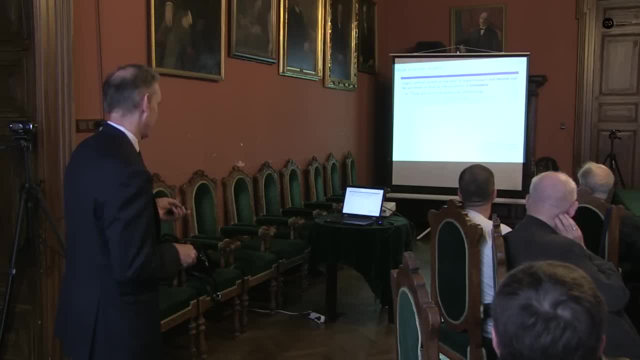 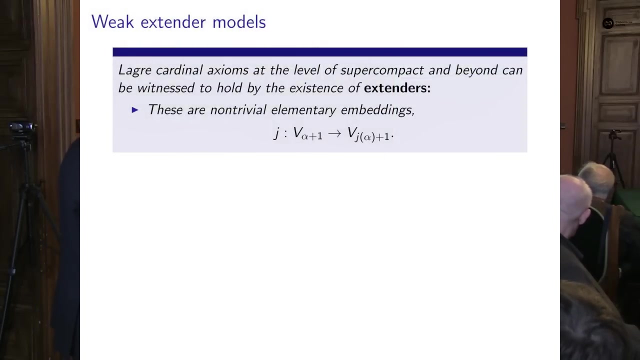 I'll go back and forward There. Okay, so large cardinal axioms, at the level of super compact and beyond, are witnessed to hold by objects called extenders, which of a certain form. now they are not called extenders. Now, if you're not a logician, 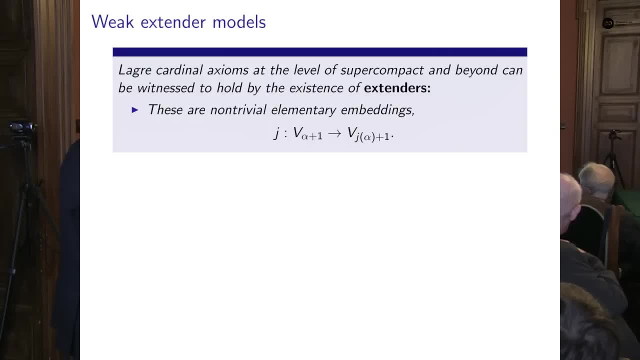 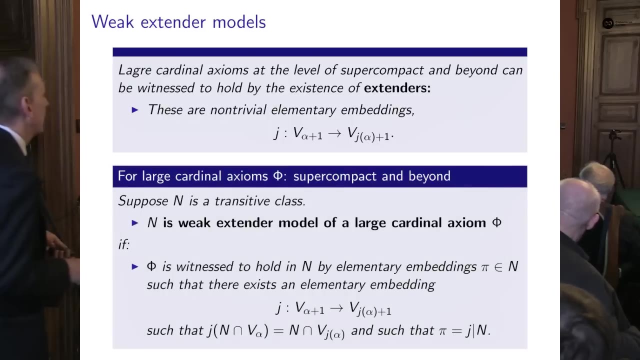 it's not going to make any sense, But these are non-trivial. Non-trivial means not the identity, Elementary embeddings from a level of the universe to another level of the universe. An elementary embedding is a function that preserves truth. So, however one conceives of an enlargement of L. 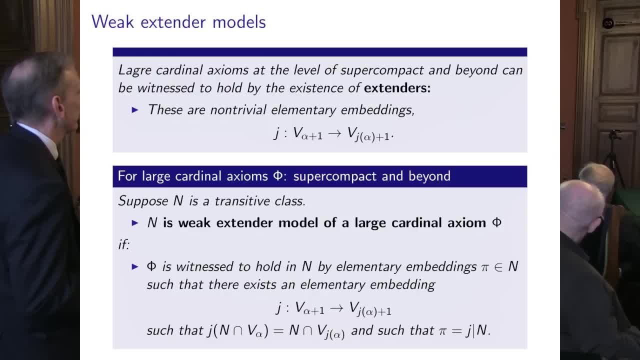 you want it to satisfy this property And the way I'm stating it. this is only for super compact and beyond. Because I've taken a lot of time, I've taken a very simple definition for extenders. We say that N is a weak extender model. 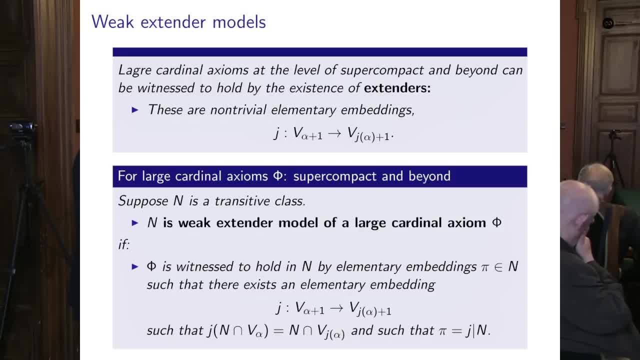 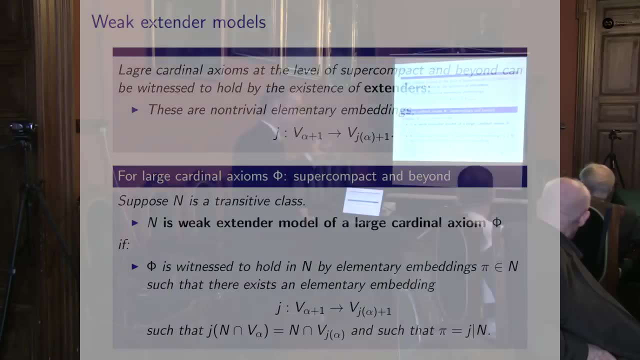 for a large cardinal axiom if it's a witness to hold in the model by embeddings like this, which are the restriction to the model of embeddings in V. So the language of extenders, the occurrence of extenders are what certify something as a large cardinal. 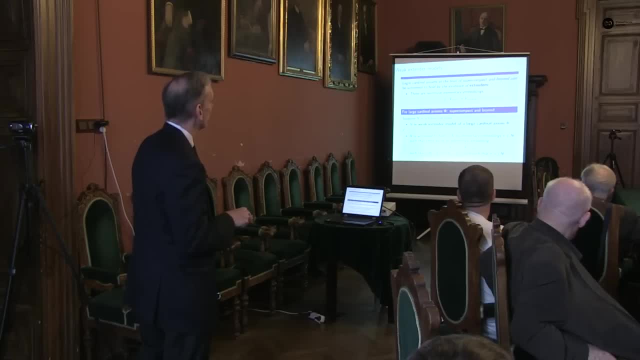 And we're just saying that this model certifies something as a large cardinal. And we're just saying that this model certifies something as a large cardinal: certificates. This model has enough certificates, which come directly from these certificates, to authenticate the large cardinal. Because if you don't couple the large 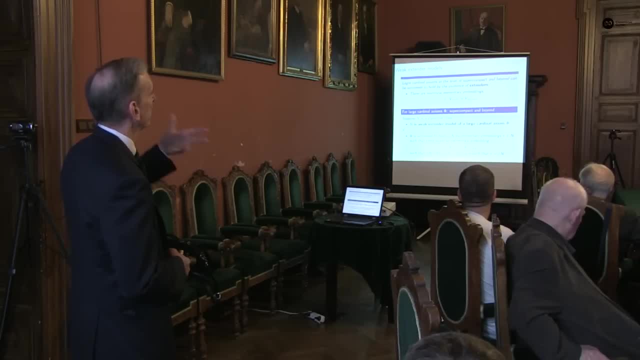 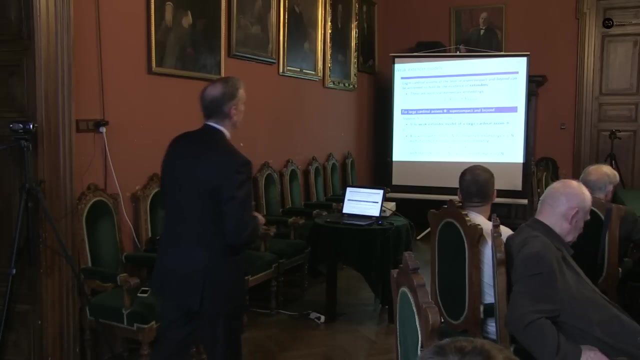 cardinals of the inner model that you're trying to build to the parent universe. they're trivial solutions. So the idea is there's a notion of a certificate for a large cardinal axiom. We're looking for enlargements of L in which there are enough certificates. 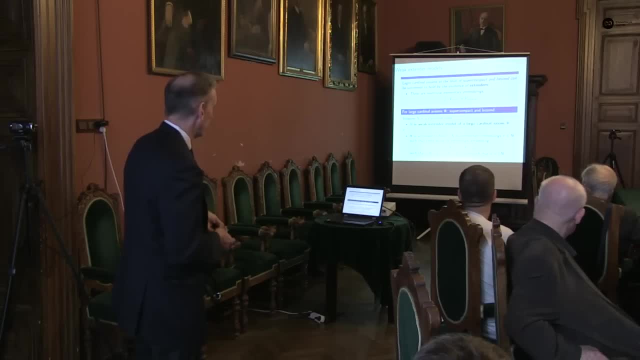 coming directly from the parent universe. So this is not an enlargement of L. V satisfies this condition, But however we build the enlargement, we expect it to satisfy this condition. That's the point. We're trying to figure out properties, enlargements of L. We have no idea how to. 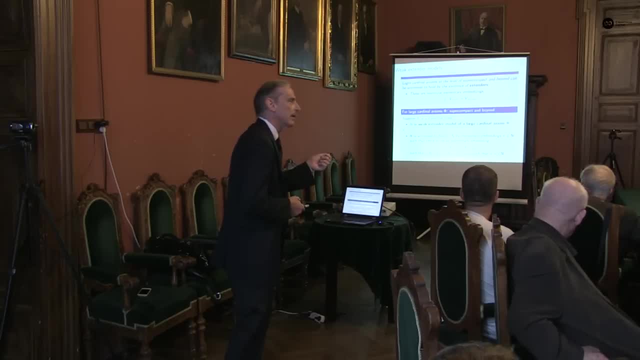 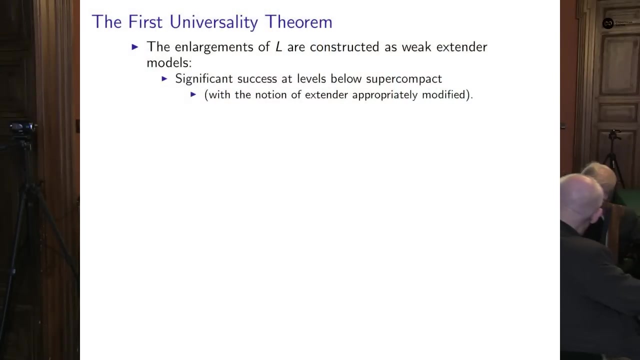 specify an enlargement of L. so we just pick a property that the enlargement should satisfy, no matter how we do it, and then we analyze all models that satisfy that condition. So there are two universality theorems. So the enlargements of L are constructed as weak extender. 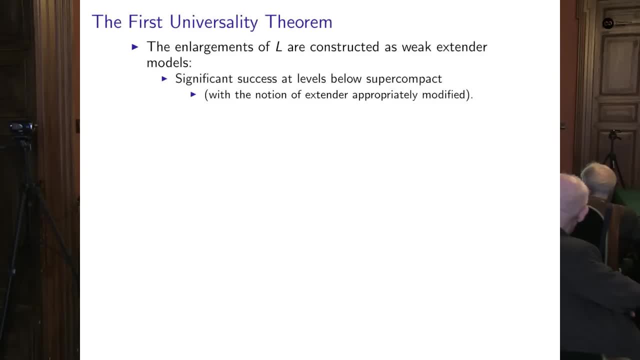 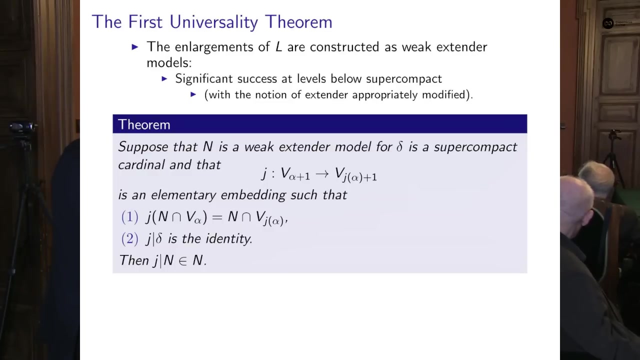 models. They're significant success at levels below supercompact. but there you have to use the right notion of extender. The notion of extender that I defined was only relevant to supercompact and beyond. So the first universality theorem says that if you have a weak extender model for delta, 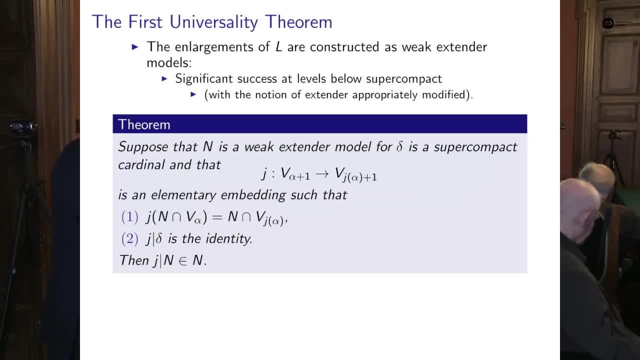 super compact and that you have an elementary embedding in v from one level to another, which is the identity at delta, and sends the level of the inner model to a level of the weak extender model, then its restriction to the model n is actually in n. 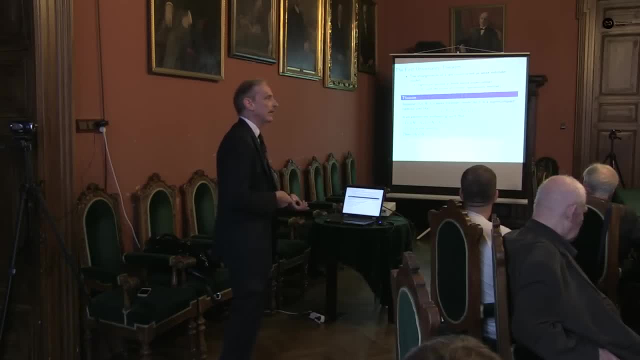 Now you might say: well, what's the fuss? You said that a weak extender model, its certificates had to come from certificates in v. What this is saying is: you put in enough certificates to witness that delta is super compact and you've basically put all certificates in. 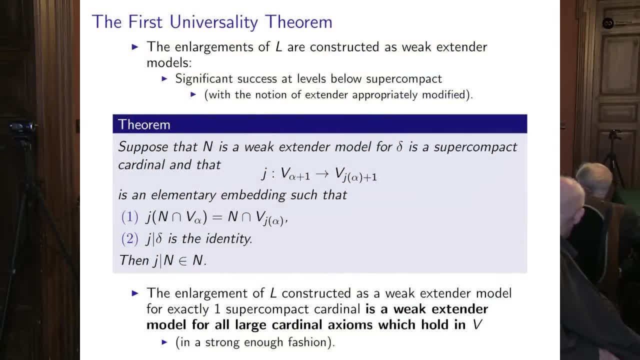 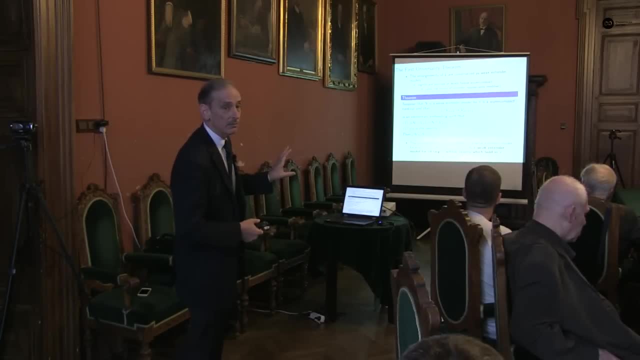 So that says that the enlargement of L, constructed as a weak extender model for exactly one super compact cardinal, is a weak extender model for all large cardinals. So that skeptical assessment was completely wrong. possibly That instead, if you target one super compact, 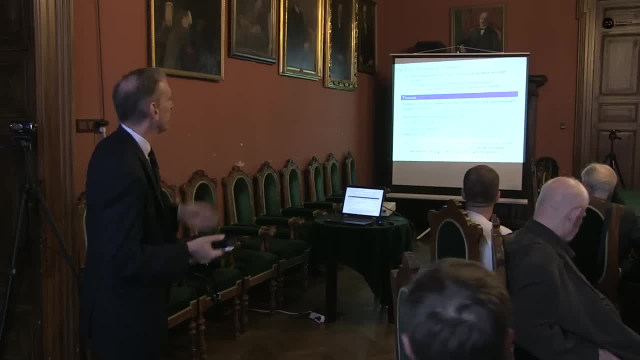 you go through all this work to build that enlargement and something magical happens: It's the ultimate enlargement. That also explains why there was no progress, Because if you try to build the enlargement for two super compacts, it's not going to work. 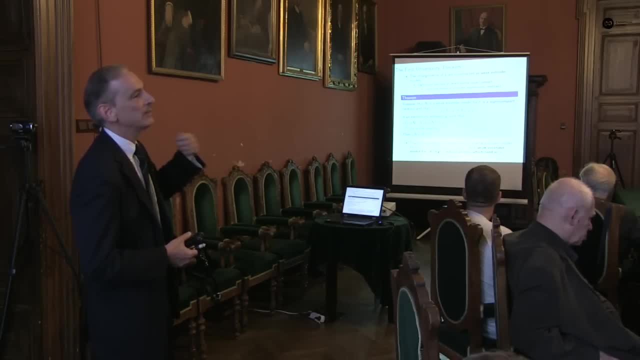 Because when you build enlargements, the danger is putting redundant information in. Because you want to control the enlargement, You never want to put information in that isn't going to be there anyway. And so what this is saying is you better not put any information in past? super compact. 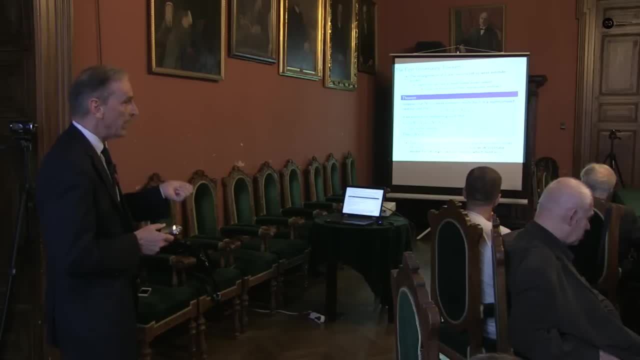 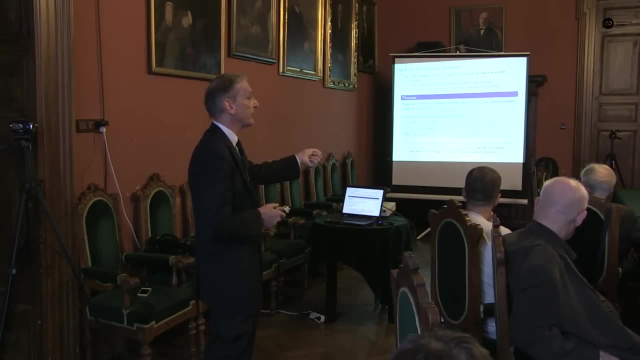 because all those certificates are going to appear anyway And if you try to put it in, there's going to be a collision between how you're putting in the new certificates you shouldn't be putting in and how they're going to appear, And that's why you couldn't make progress. 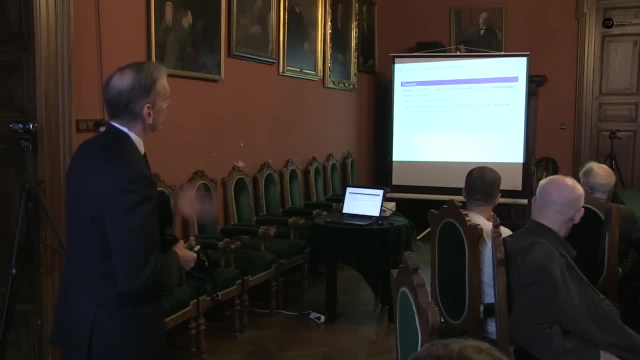 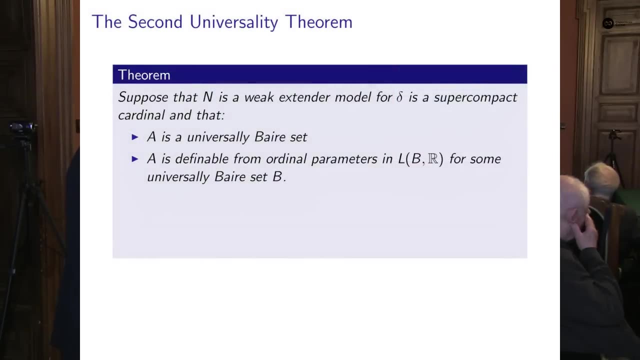 OK, there's a second universality theorem that traces back to the universally bare sets. Let me just state it. We have a weak extender model for delta, super compact. We have a universally bare set. Let's suppose that this set is definable from ordinal. 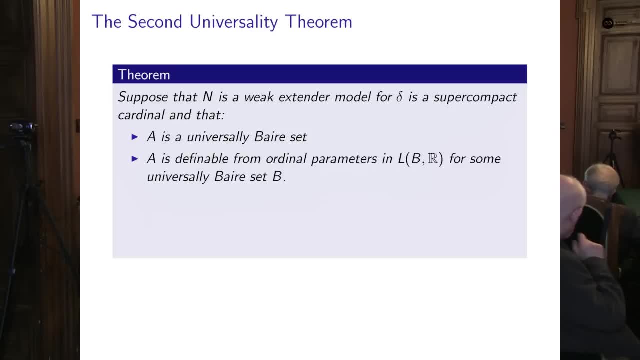 parameters in L of B and R for some other universally bare set. Now let's suppose that our weak extender model actually contains this set. If it contains the reals, then it must contain A, And moreover, A is a universally bare set within N. 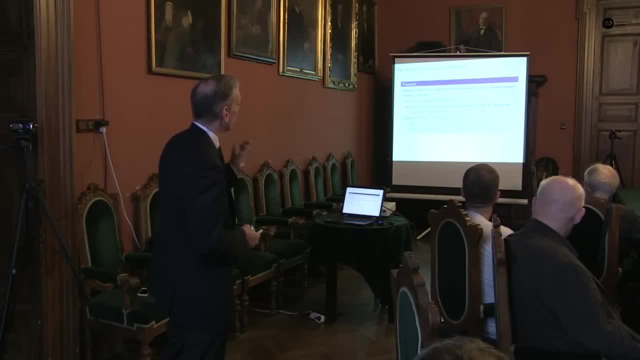 So it's a little technical to explain the significance of this, But remember we generated L of R is really taking Gödel's enlargement process, L, taking Gödel's L and relativizing it to the reals. If you had an enlargement construction for L. 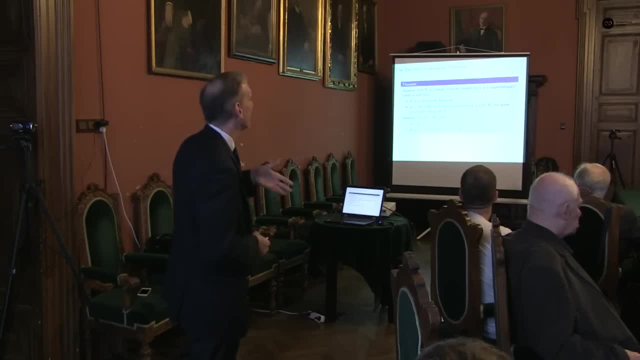 well, you could do it over the real And you would expect to get canonical sets of reals. So this is saying that if you can build an enlargement for super compact and you build it over the reals, apply that construction instead of L of R, N of R, if you want. 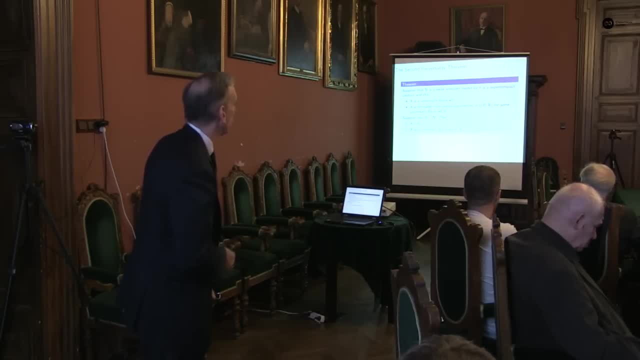 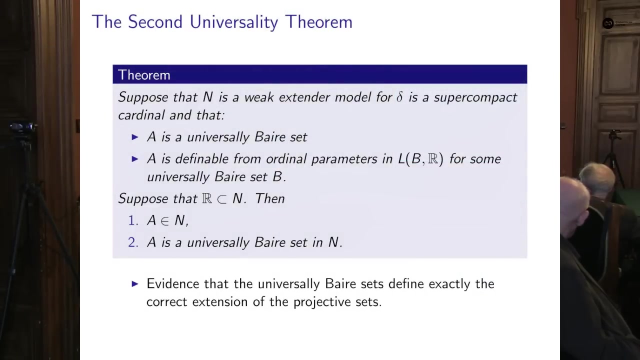 then you get these universally bare sets. So that's another way in which the enlargement of L for one super compact is also universal, the ultimate enlargement. You'd expect this to be true. OK, so this is fairly convincing evidence that if you can build the model that the universally bare sets 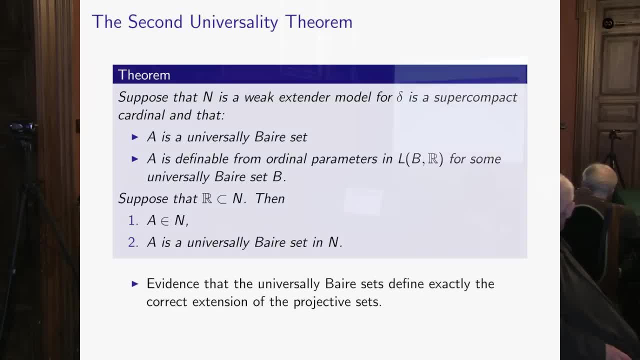 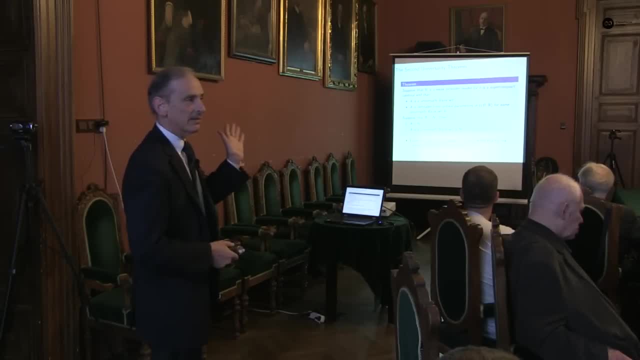 define exactly the correct extension of the projective sets. All right, so there's still something missing, right, There still may be a Scott's theorem, And we don't know whether there's going to be a Scott's theorem, But one can state a conjecture now, a precise conjecture. 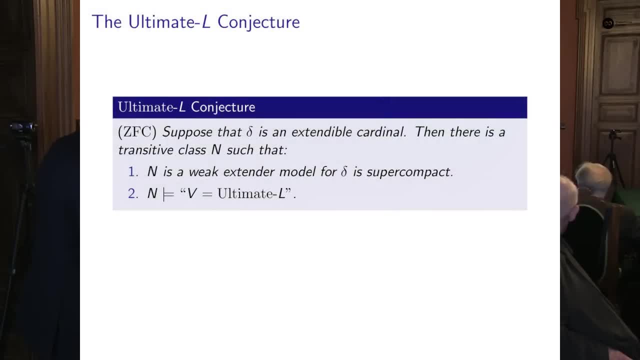 And this is the ultimate, The ultimate L conjecture Here it is: Suppose delta is an extendable cardinal. It doesn't really matter what that is. It's a bit stronger than super compact And the conjecture is there must exist a transit of class N. 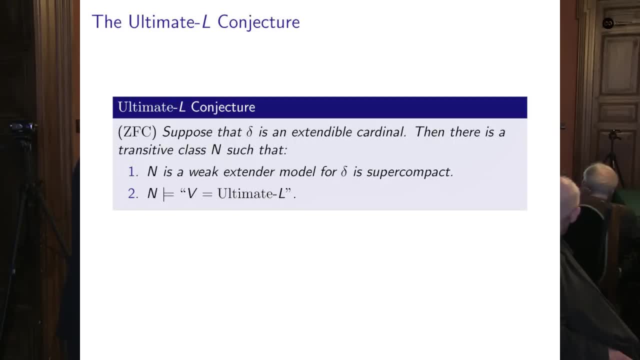 N is a weak extender model for delta, super compact, And N satisfies V as ultimate L Now by the universality theorem. if this conjecture is provable, there's no generalization of Scott's theorem to V as ultimate L because this weak extender model 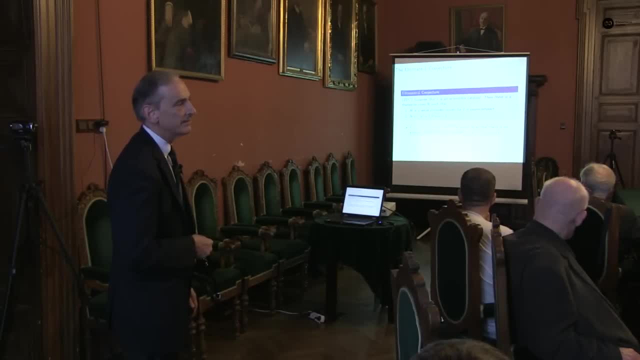 inherits all possible large cardinals from V. So if, for example, you knew that some large cardinal, like Huge Cardinals, refutes, or thought it might refute, V's ultimate L, then it must refute this conjecture. And again you have to know the cardinals hold them. 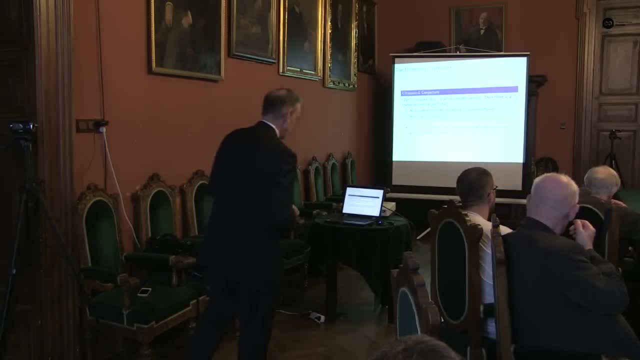 being a slightly stronger form. The precise theorem would be: we weren't very imaginative in naming large cardinals as one huge, two huge, three huge people were running out of imagination. But the theorem here would be: the universality theorem says that if for every finite k you 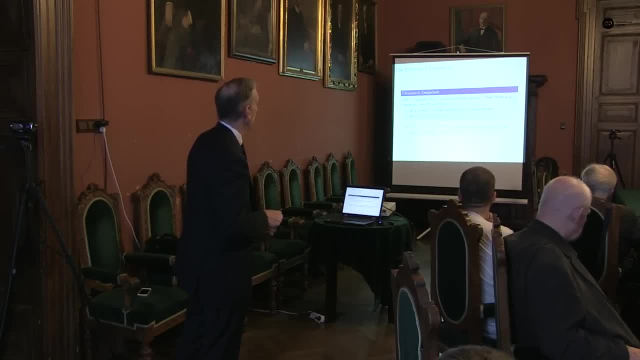 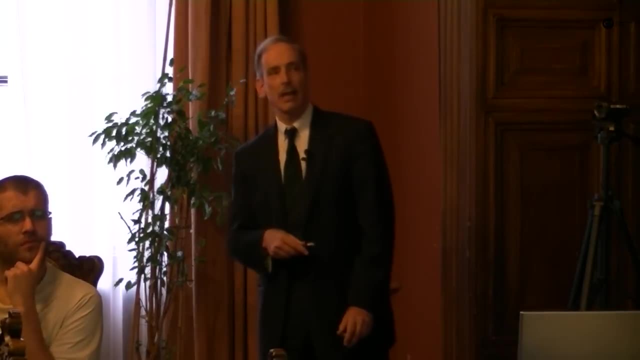 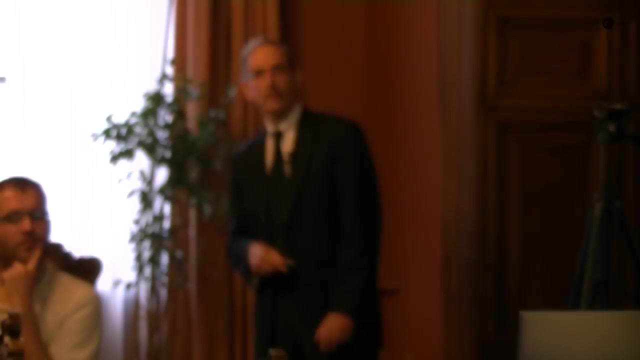 have a proper class of k- huge cardinals. and you have a weak extender model for delta, super compact, then in n for every finite k, you have a proper class of k- huge cardinals. So if this conjecture is true, huge cardinals cannot refute. V is ultimate L And this works. 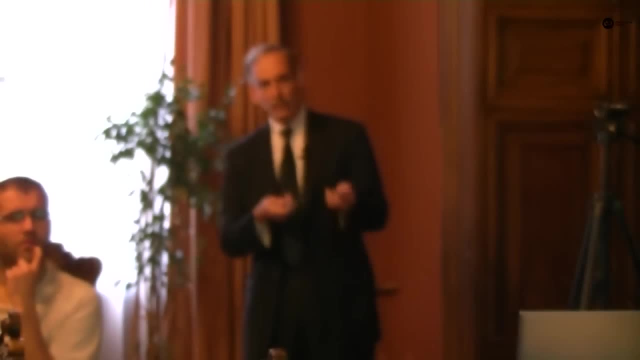 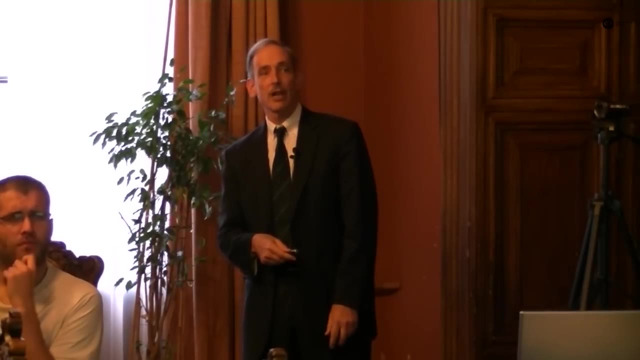 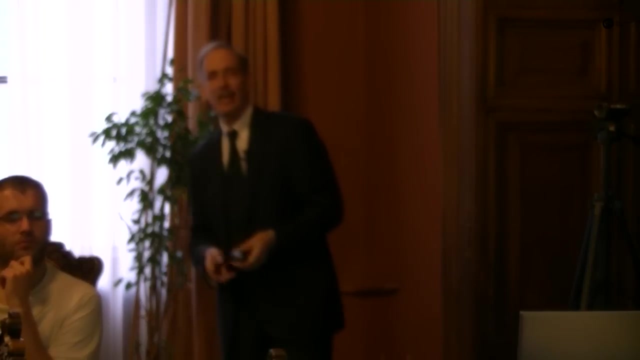 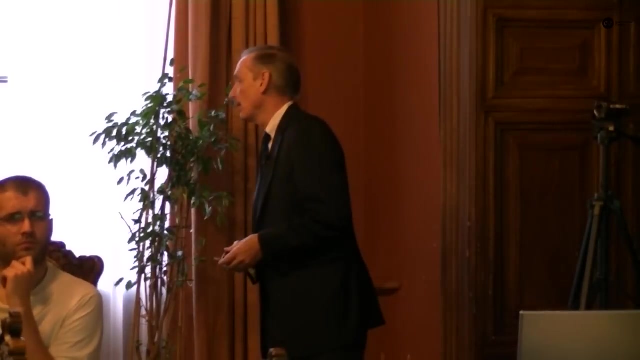 for any notion. So this conjecture would really say there is no generalization of Scott's theorem to V is ultimate L. It would be the ultimate refutation of the skeptical assessment. And there are a host of other results that argue that if this conjecture is true, there's 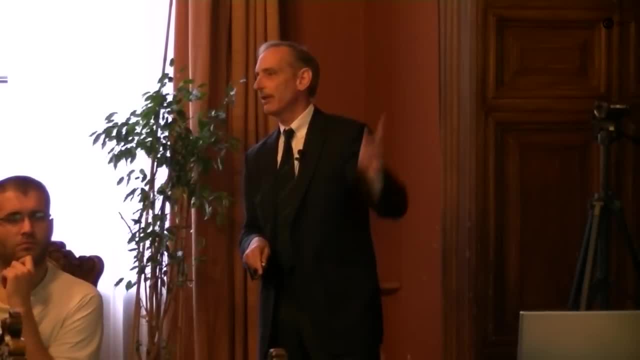 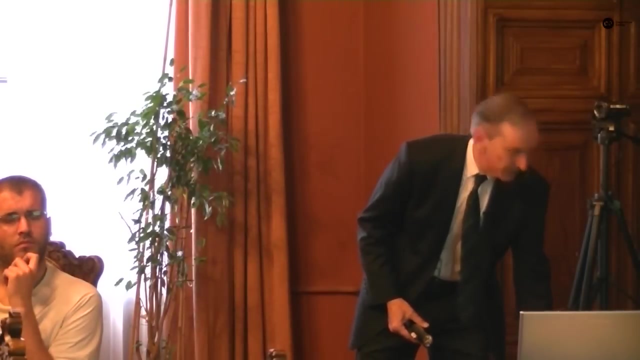 a compelling case that V is ultimate L. I mean the consequences of V is V equals ultimate L that I listed, and there are other consequences as well. So it all comes down to this conjecture. Now, the minute, you're in a framework where you have a specific conjecture, well that. 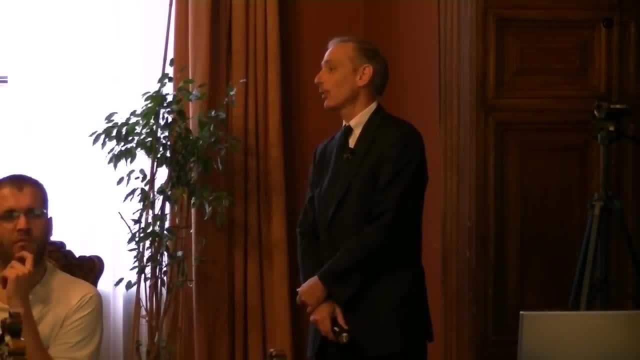 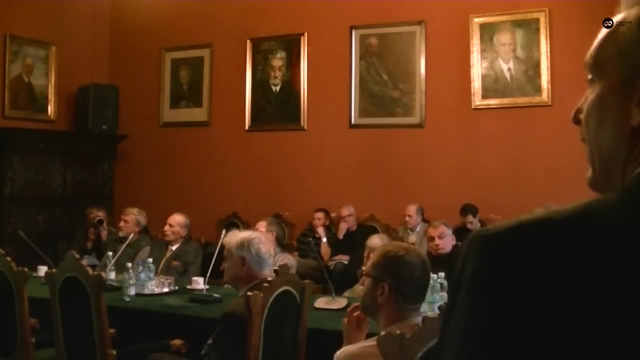 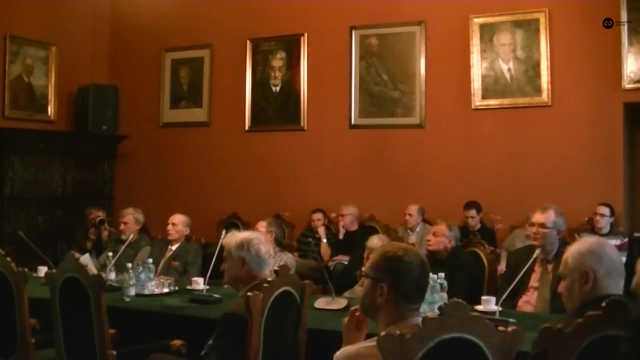 conjecture could be wrong, It could be refuted. So that's where we are right now. We have a specific conjecture. If it's provable, we have the case for V is equal to ultimate L. We have, arguably, the new axiom that we've been looking for for the universe of sets, which, in conjunction, 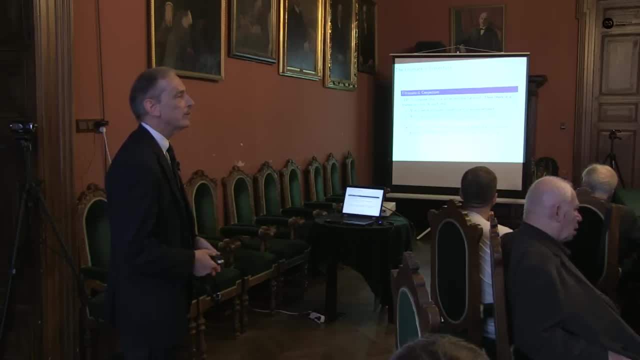 with the other axioms would give an unambiguous conception of the universe of sets. The only ambiguity would be what large cardinals are present. The only solution, The only source of independence would be: how tall is the universe? And that was always Gödel's dream, that you might reduce all questions to questions about. 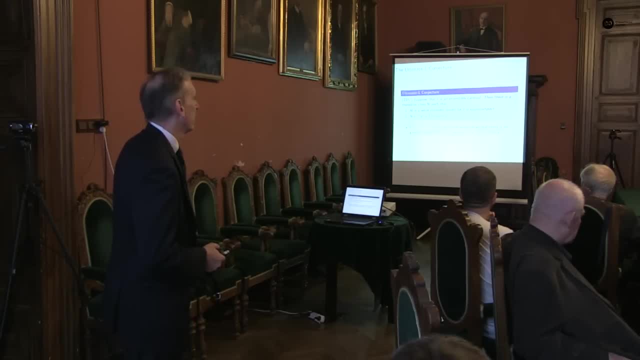 infinity. This would do that. But there's another possibility: that the universality theorem is the first indication that this whole approach fails at supercompact. In particular, this conjecture is false, In which case it's backtracking. It's backtracking. 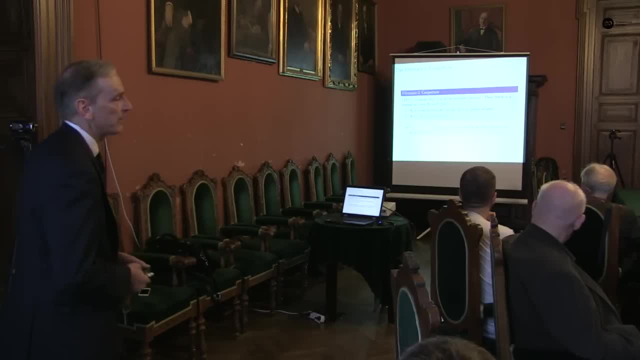 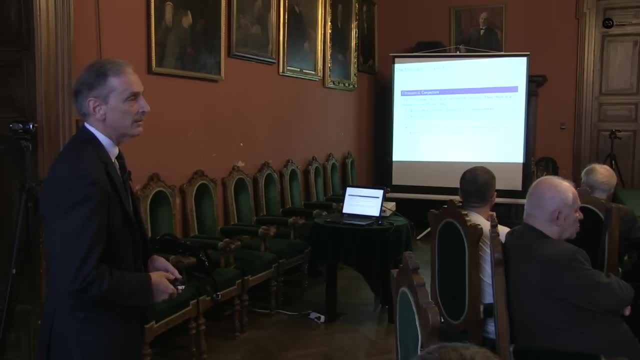 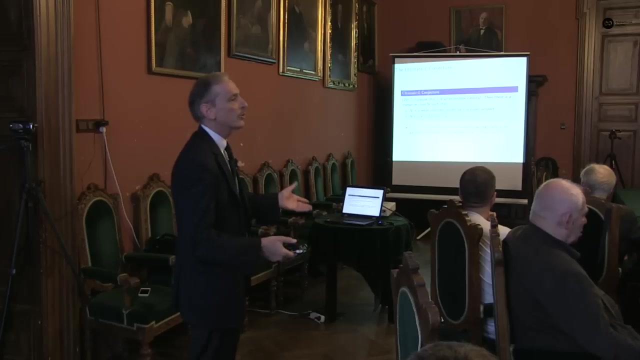 Maybe in the end the ultimate skeptic is correct, that the entire conception of the universe of sets is a complete fiction. It's just intuition gone wild. It's a human creation That there's no truth there. Now the consistency claims are just false. 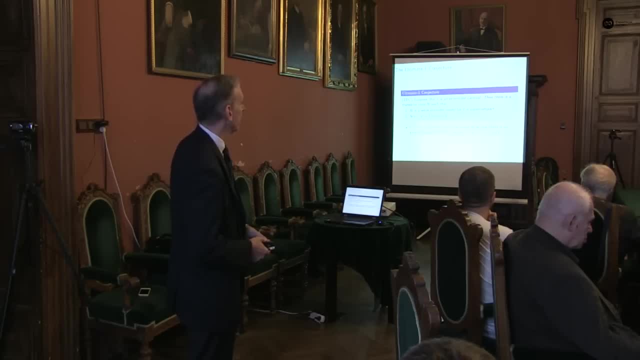 you are pushed back against that a little, but we can't be sure that's not true. I mean I get asked a lot. I mean one criticism of the study of infinity is that it has no applications. you know it's not going to help you least yet it. 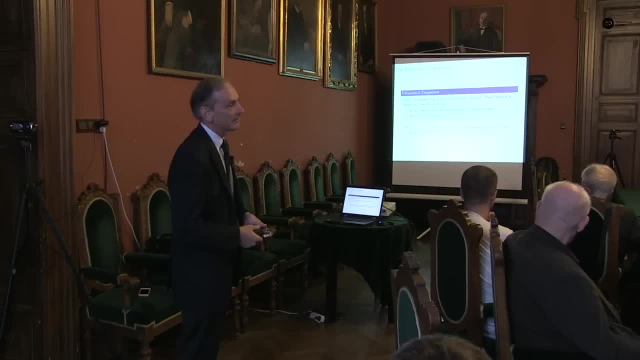 plays no role in the theory of physics. we don't know what will happen eventually. but you know I'm not troubled by that. I mean assuming this conjecture is true, then to me it's a win-win situation. that's a human English phrase. win-win. in other words, there are two possibilities: either at some point, 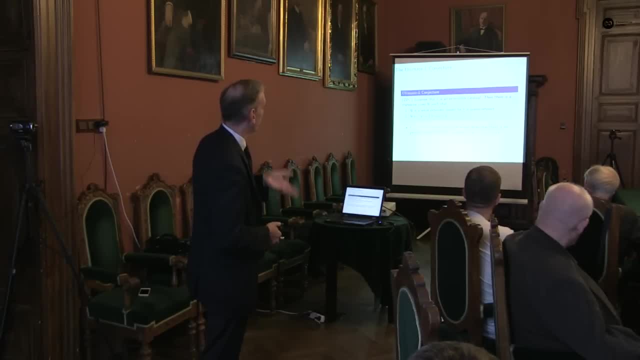 physics develops, the mathematical physics, or the mathematical understanding of the physical universe, starts to need large cardinals. remember large cardinal axioms with finite istic consequences. so it's not completely unreasonable that large cardinal axioms provide mathematical truths that you need to do the analysis of physics. we already saw an instance of that. infinitely many. 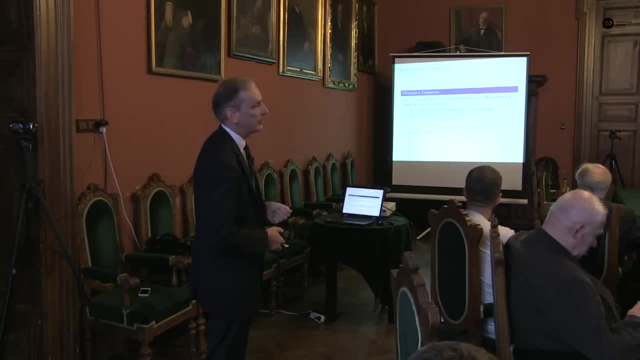 wooden cardinals imply that the projective continuum hypothesis is true. that's a remarkable connection between very large sets and very small sets. who's to say that doesn't happen in physics somewhere? so that would be a win. and I'll tell you I would be a stunned. 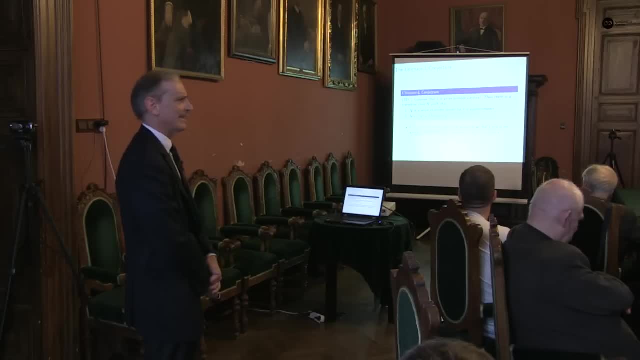 you. if that ever happened, I would. in my think that's never going to happen. alright, so then there's the other possibility. set theory is completely irrelevant to physics, never has a connection. but wait a minute. that's almost more interesting because we have a span. if this conjecture is true, we've 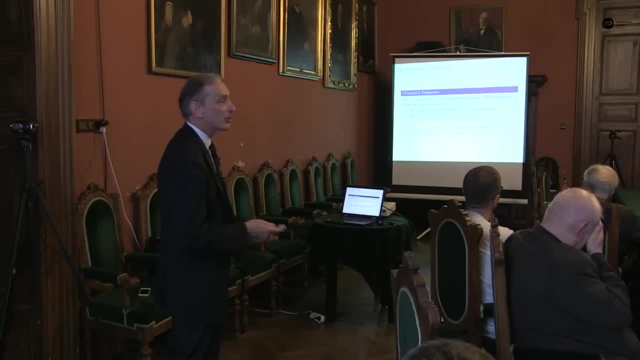 argued. there's truth here for set theory and it's a truth that's not about the physical universe. we continue to get bottom of the problem with this one. should I imagine that also mushrooms? so the question is if a universe hasику vanished and they've gone through the 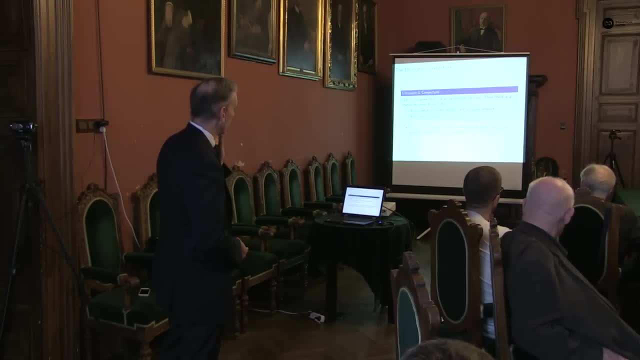 conjecture. let'sца 38, where the emergence has shown that certain intuitions along the way were completely wrong and so 15 years ago I would have said there could be no. I would have stood up here and given a lecture explaining why there could be no. 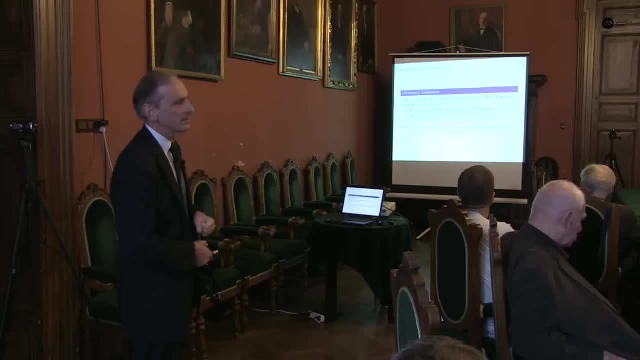 ultimate L just seems so clear and it was just completely and totally false because of that unexpected development. so that's where we are. to me, set theory is at a tipping point. it's another English phrase, right? we don't know which way it's going to tip, and which way it tips depends upon this conjecture it may. 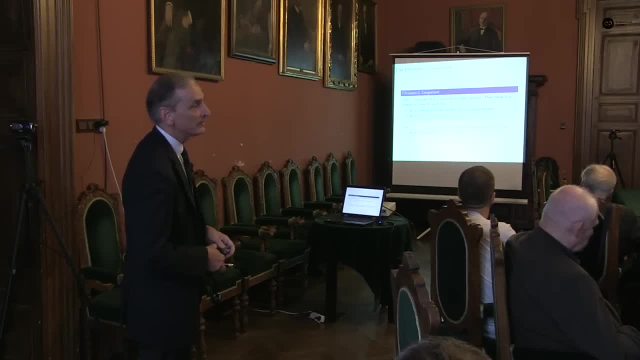 tip into light. the conjecture is true and now we can really get started in set theory. the trouble with set theory is it's very hard to do math Tomatics when every problem is unsolvable. how can you build a framework of set theory when every set their- and it's not just ch- that's unsolvable? many 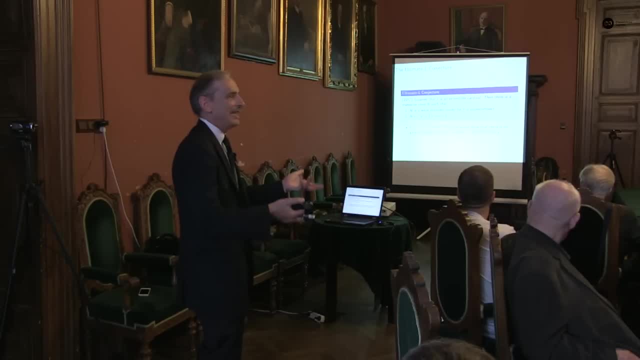 set theoretic questions are: it's like you can't get started because you, you just can't get started, right, it's like you have to make choices? oh, I want to analyze this problem. oh, it's independent. I've got to choose an answer. all right, I. 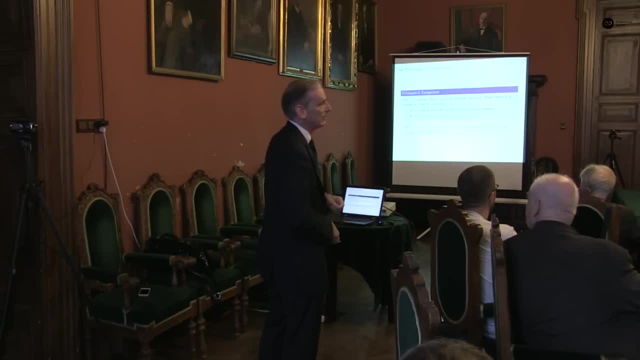 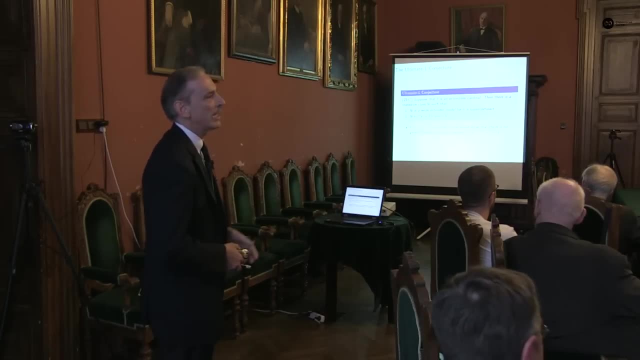 choose true. Now I go on to the next problem. Oh, it's unsolvable. Well, I'm going to make another choice. That's not mathematics, So set theory has never had a chance. V is ultimate, L removes all of that. 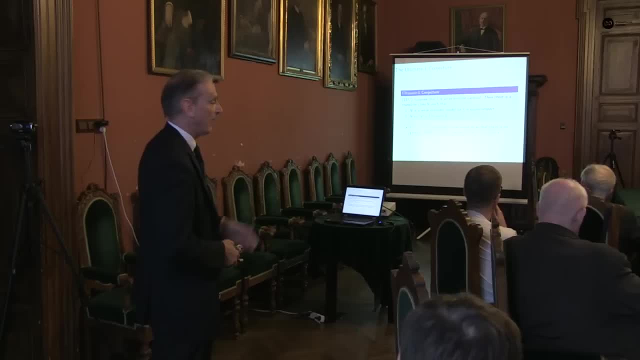 The only ambiguity is the size. Well, that's OK. If I encounter a problem and I say, oh, it needs some large infinity. well, we want all infinities to exist, So we have a way of deciding that question. 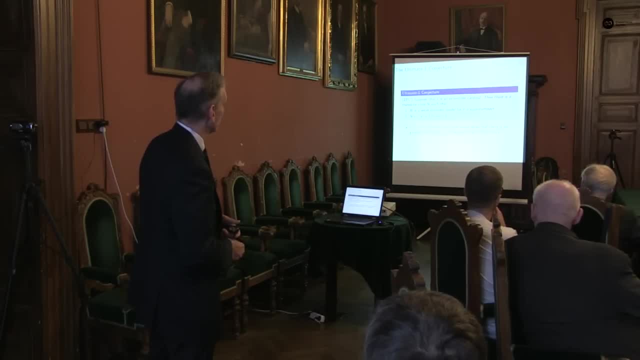 All right. So what's the other way it could go? Well, it could tip into darkness- Maybe I shouldn't use light and dark, So tip into chaos. And that is. this conjecture is false. The universality theorem is the first.